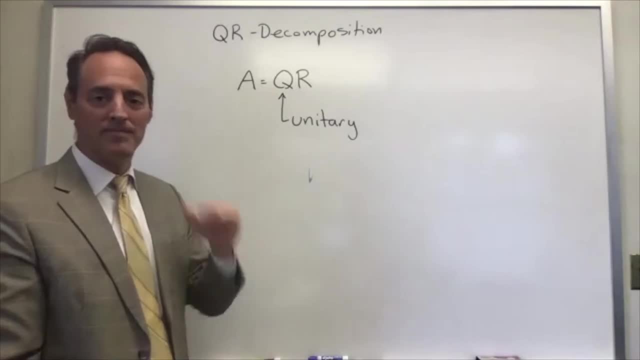 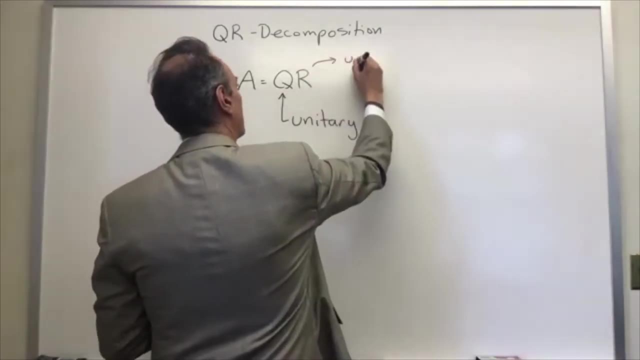 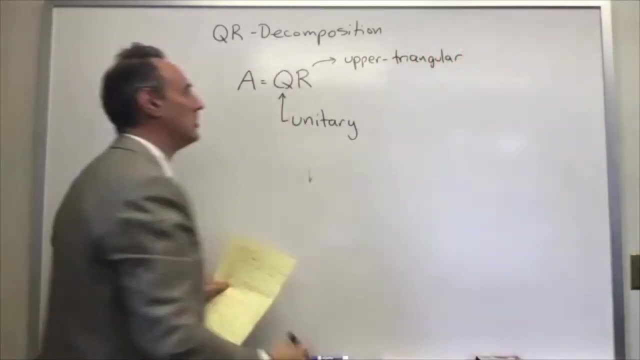 associated with them. All the eigenvalues live on a unit circle. So you prove that in your homework. one And R is upper triangular. Okay, So the idea is to write A as a product of Q and R. In fact, part of what we're going to learn. 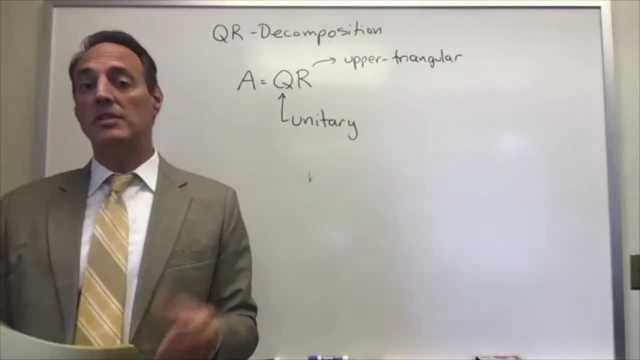 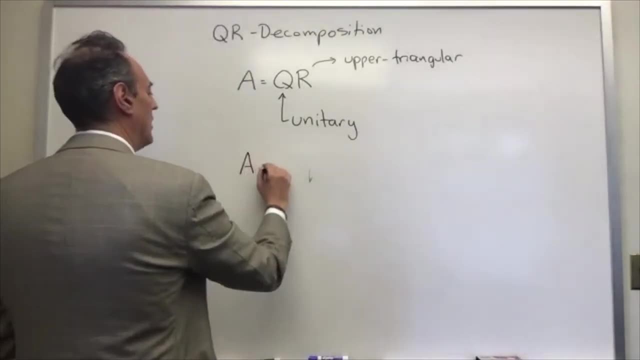 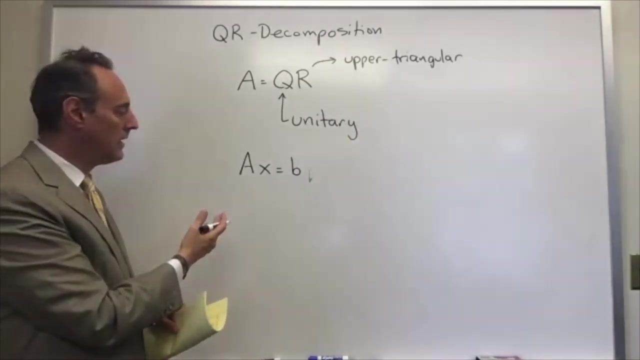 today is how to do that. Okay, How to do this decomposition in particular. Now, how does it relate to AX equal to B? Most of what we're going to do, of course, in linear algebra is always going to come down to thinking about AX equal to B. And so now you say: well, I have X equal to B. 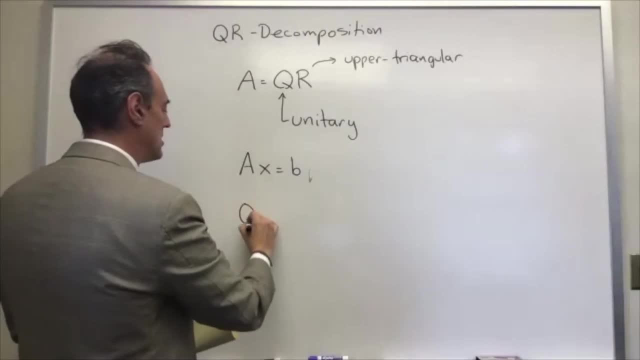 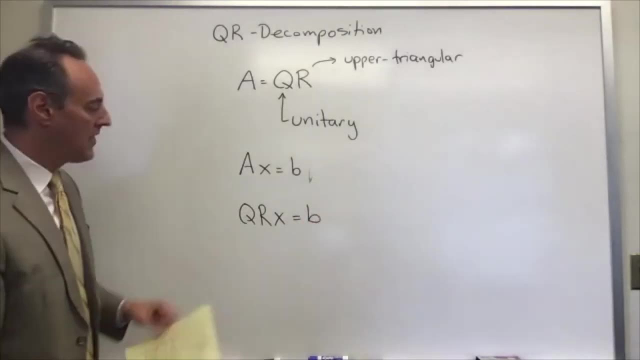 but A. if I can do this, then I'm going to be able to do this, So I'm going to be able to do this decomposition right. It becomes QRX is equal to B, And then what I can do on both sides is: 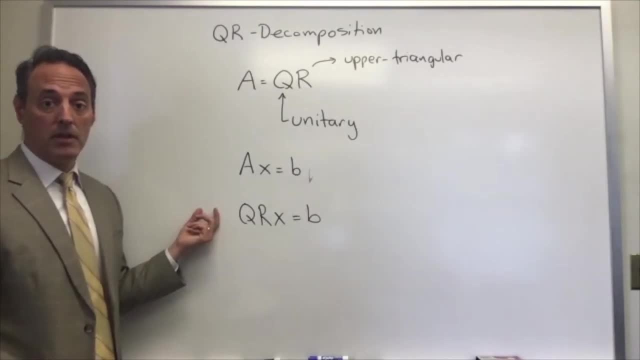 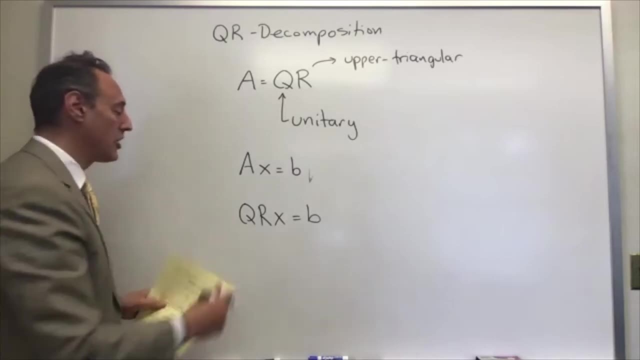 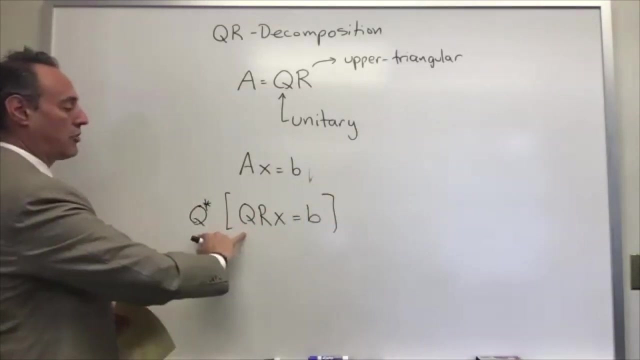 multiply by its adjoint. Remember that, or sorry, it's transpose here, And so if it's a unitary operation, I can just multiply by Q star, by the adjoint on both sides. If it's unitary, Q star, Q. 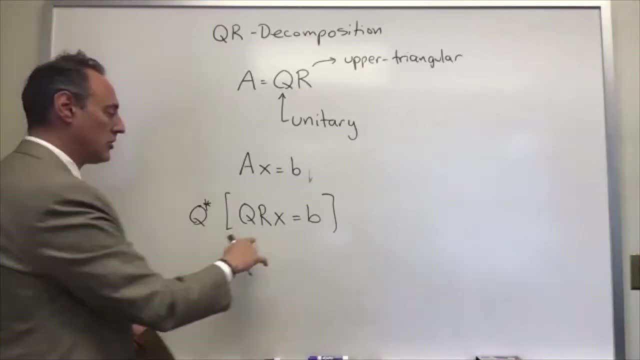 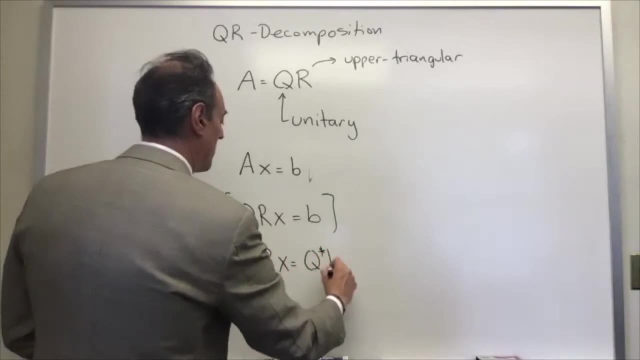 is equal to B, And then what I can do on both sides is multiply by its adjoint, And so if it's identity, so it's one. So then here you're just going to get. RX is equal to Q, star B. 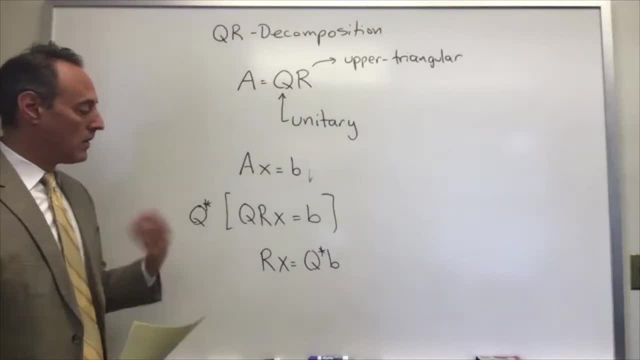 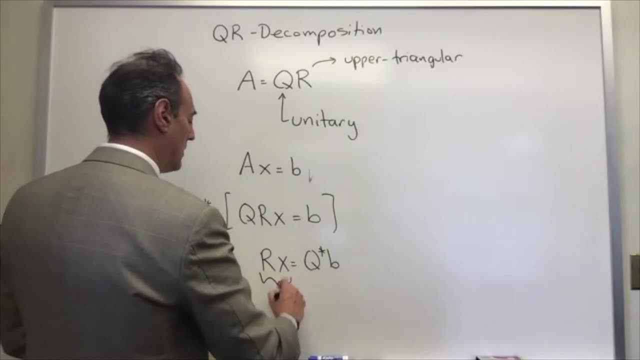 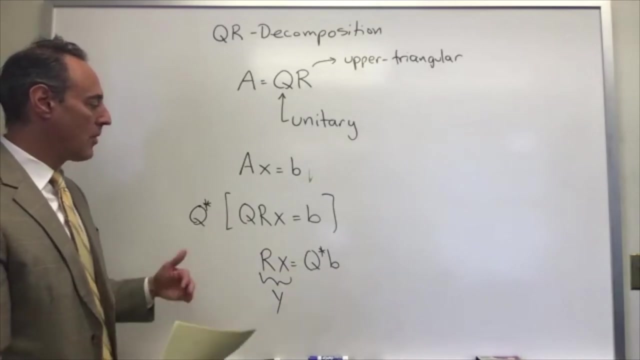 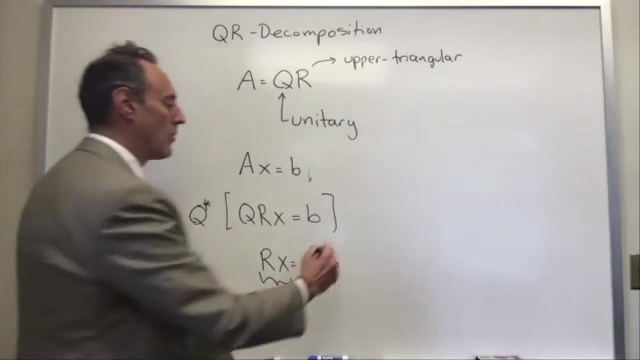 Okay. So now you can start thinking about this and saying, okay, well, what I'm going to do is call this RX Y. I'm going to call that variable Y, Okay. So notice then what we can do with this problem in solving for it. The first equation, then one. 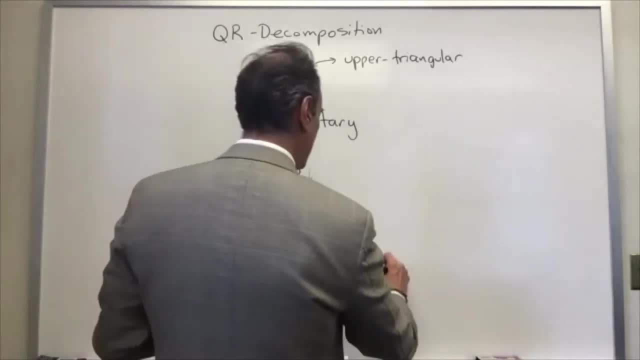 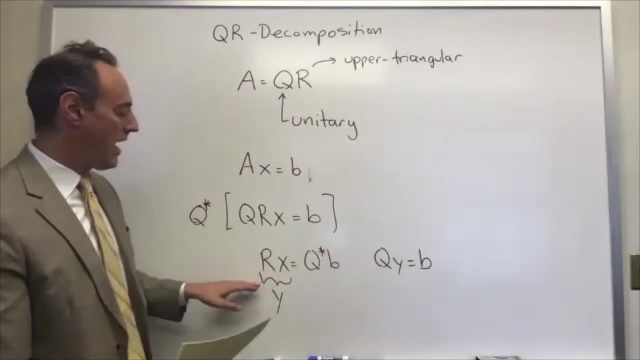 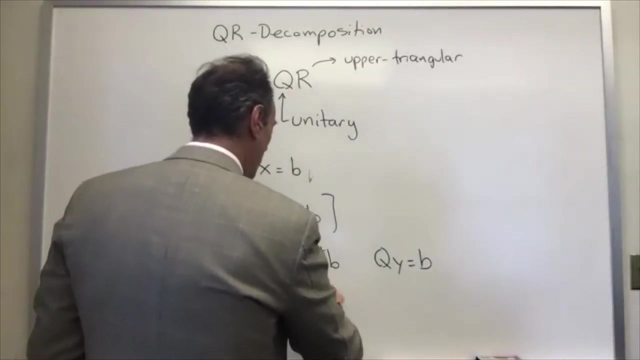 way to think about it, if that's Y is to say that the first equation is: QY is equal to B, And then I have: once I have solved for Y, then I have here: Y is equal to Q, star B: Okay. 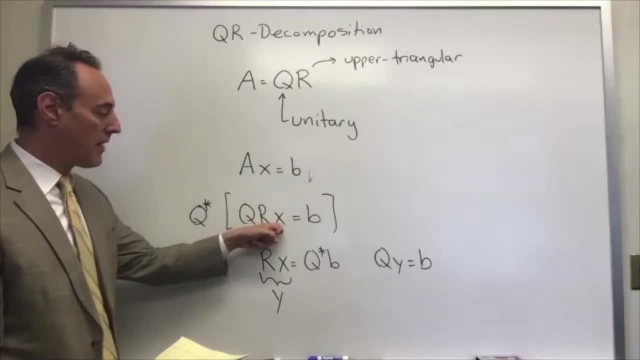 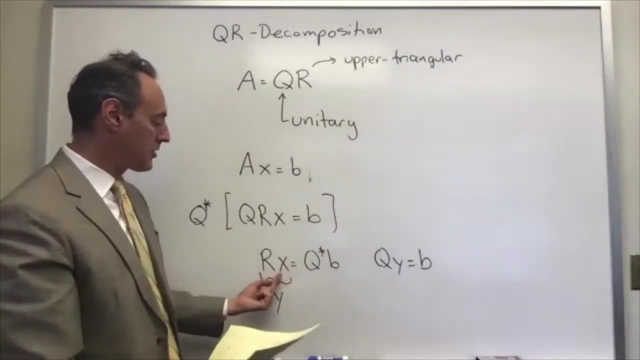 So the decomposition, remember, I'm trying to solve for X, So the first thing I'm going to solve for is is is right here. I'm going to sorry, I'm going to solve for Y from right here And. 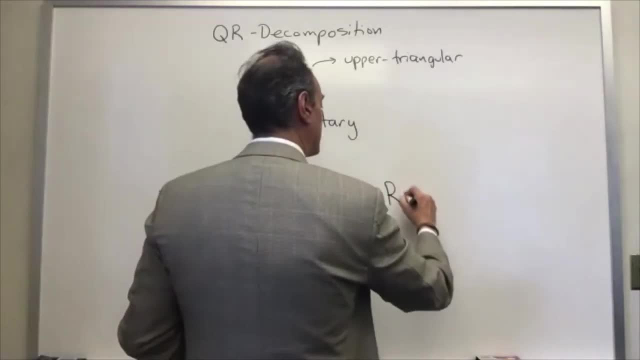 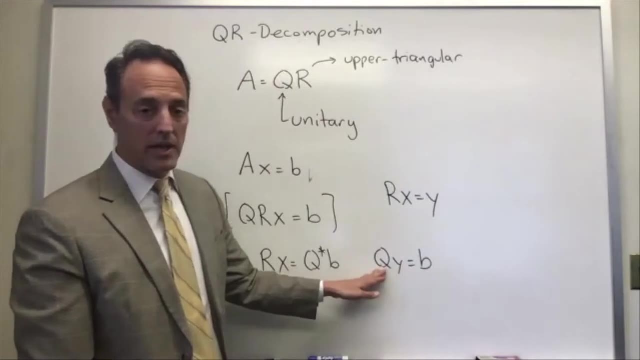 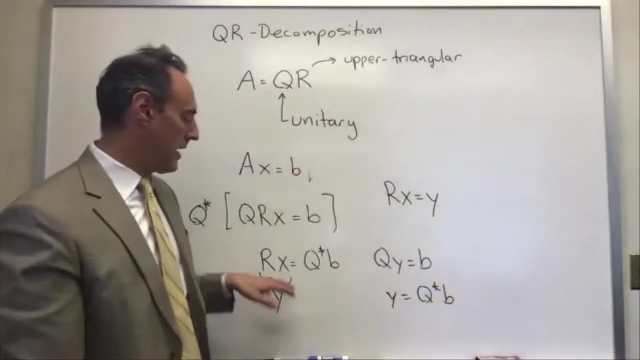 once I solve for Y, I have that RX is equal to Y. So Y is pretty easy to solve for because Q is unitary. All I got to do is go And do this right, Which is exactly what I showed you here. So Y is- just take this unitary matrix. 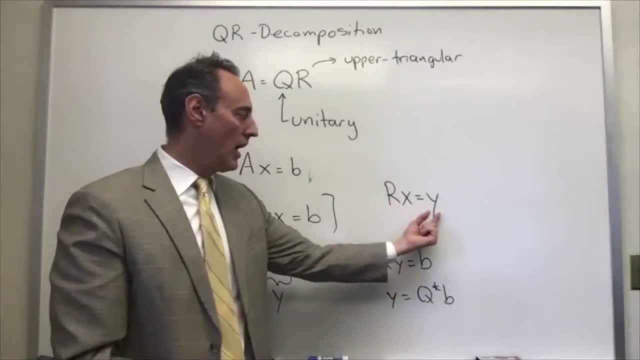 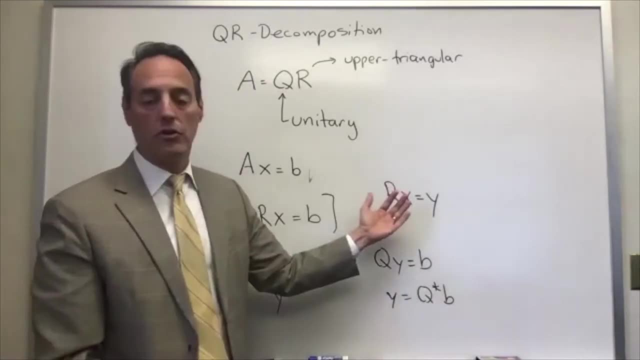 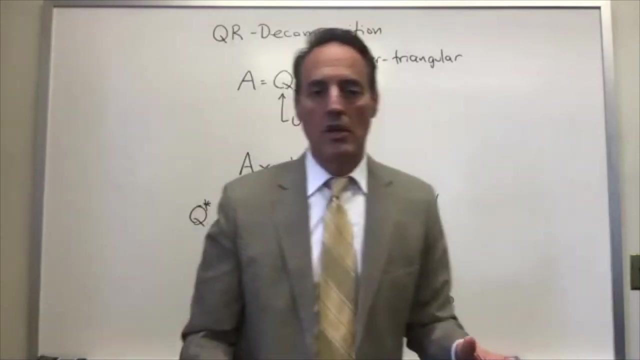 multiplied by B, So that's Y. Once I have Y, I have that right-hand side And now I solve this. but R is upper triangular form, So all I have to do is do back substitution and I'm done. Okay, So this is the structure of solving AX equal to B, Basically, if I have the decomposition. 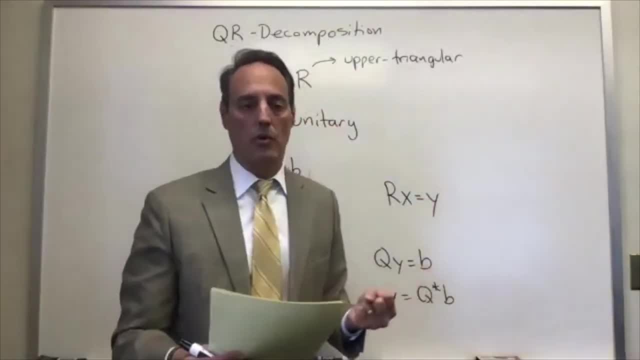 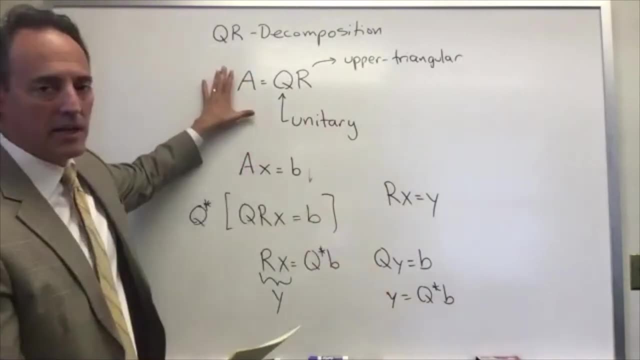 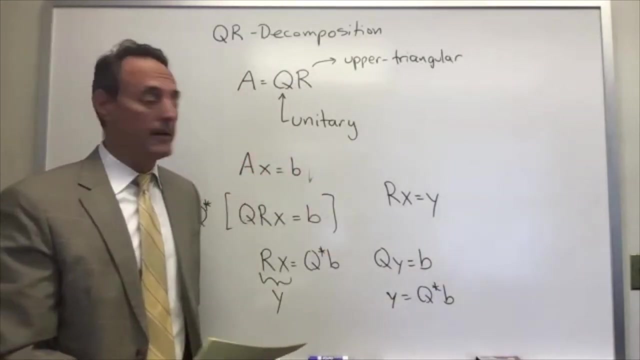 all I'm going to do is back substitution to get the solution. One matrix multiply, one back substitute and I'm done. Okay, So that's the idea of how you can take advantage of this decomposition and solving AX equal to B. Okay, So that's one of the major themes, obviously. 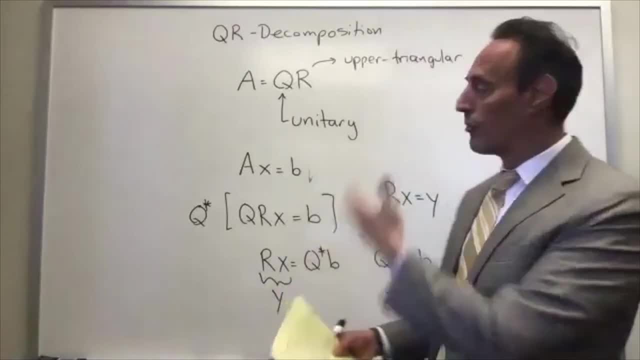 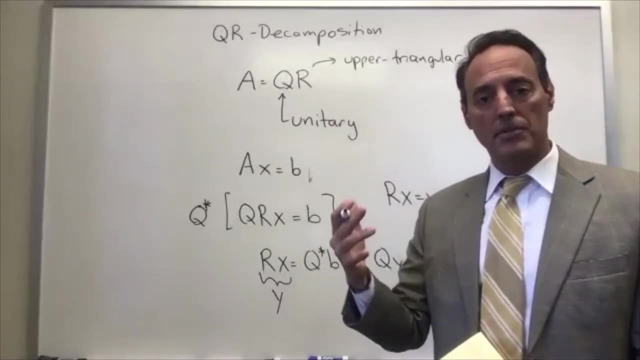 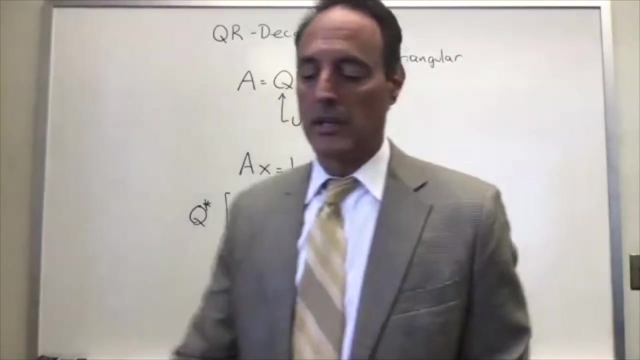 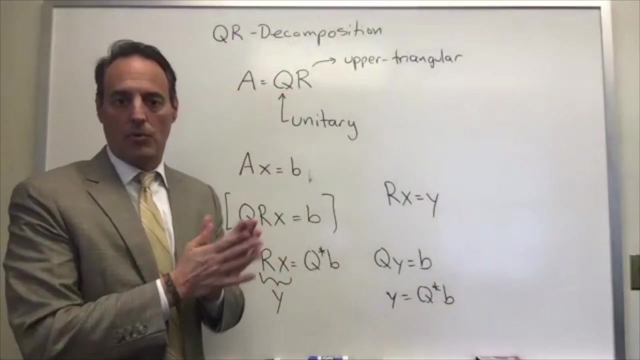 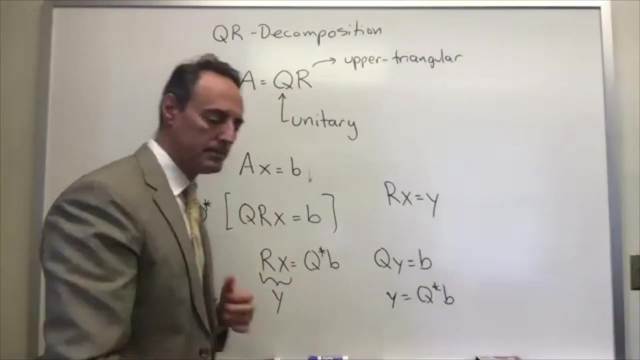 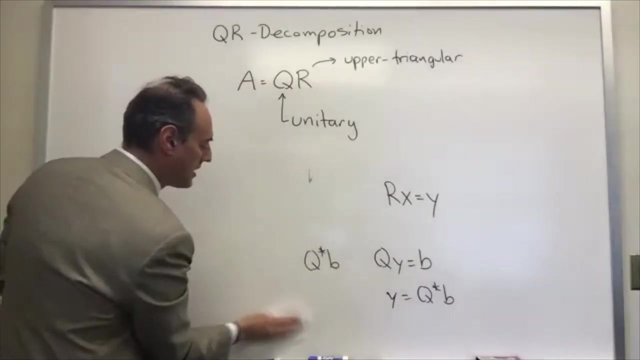 throughout the course is solving linear algebra problems of AX equal to B, And this is just one of the decompositions, And if you go back to the very first lecture, I walked through a bunch of decomposition. Okay, So that's going to be the concept. It's a decomposition we can exploit. 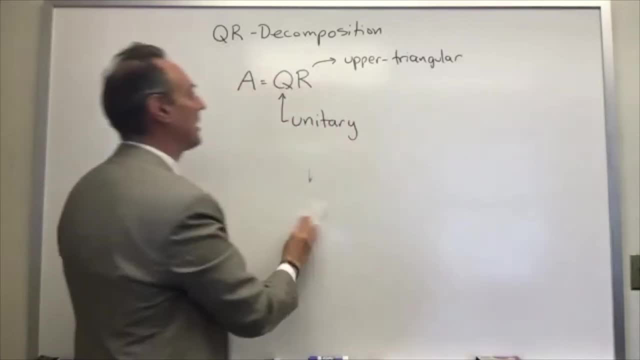 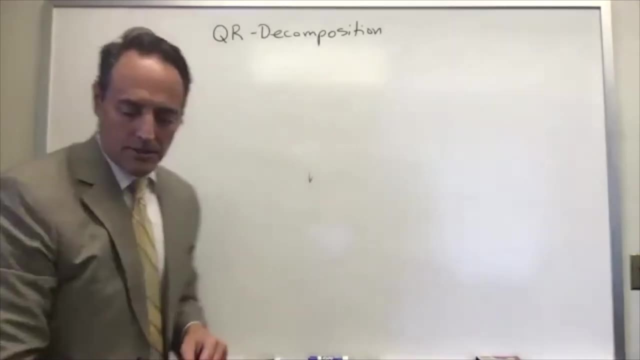 Okay, So that's going to be the concept. It's a decomposition we can exploit. It has very nice structure for us to start thinking about solving AX equal to B. So let's start with some ideas from linear algebra And in particular, I want to start. 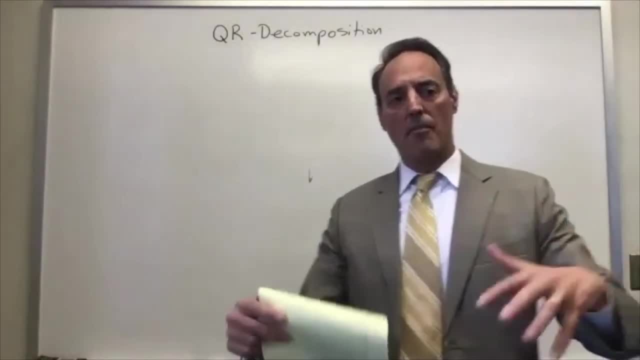 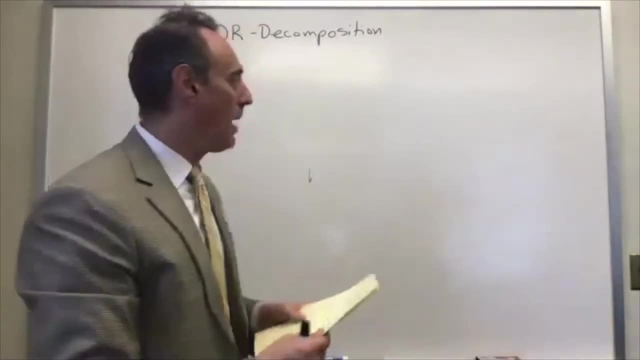 building up some- just like we did with the SVD- is start building up some background and intuition around this QR decomposition. So I'm going to think about a matrix A right And I'm going to say that the composition of AX equal to B is going to be a matrix A right, And I'm going to say that. 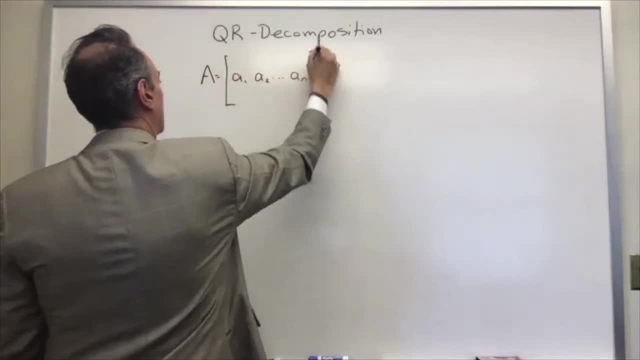 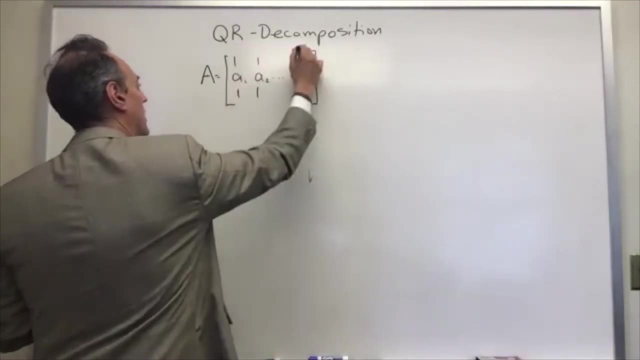 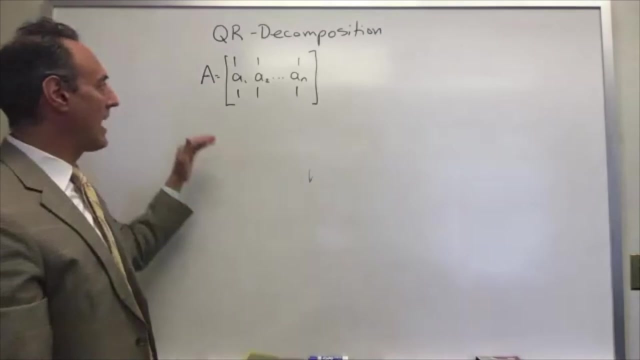 the column space is given by these vectors: A1, A2, so forth. So these are my columns of a matrix A And for the moment let's assume that in fact the determinant of this matrix is not zero. So all the columns. 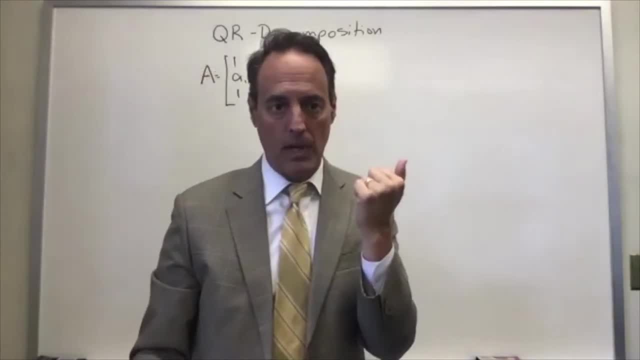 are linearly independent. Okay, So this could be a data matrix, It could be some matrix that I get from you know, a matrix A. So I'm going to say that the column space is given by these vectors: A1, A2, so forth. 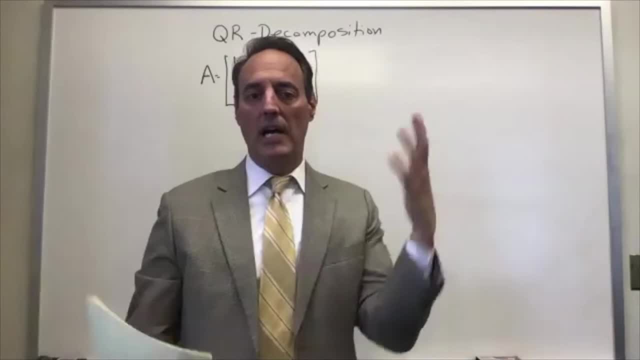 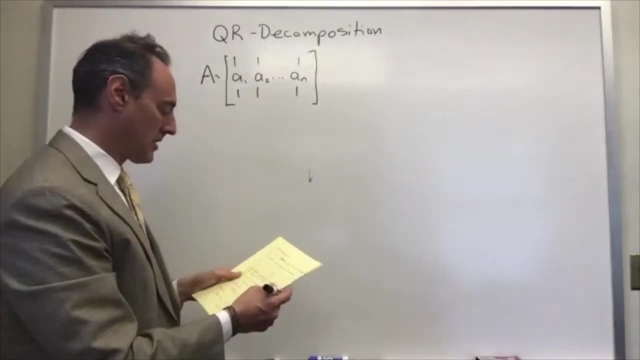 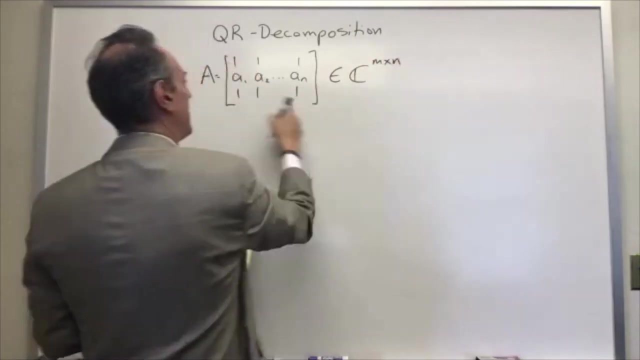 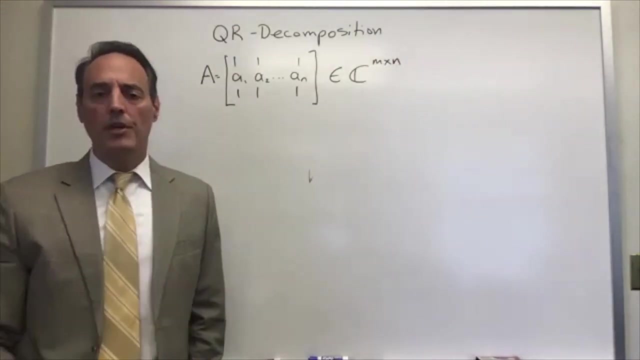 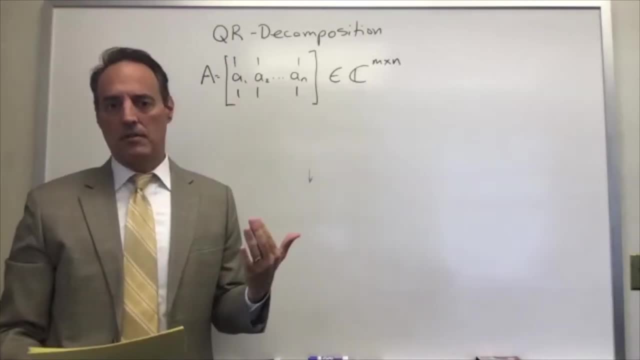 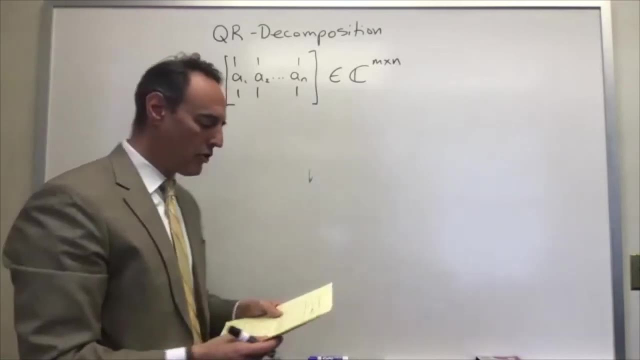 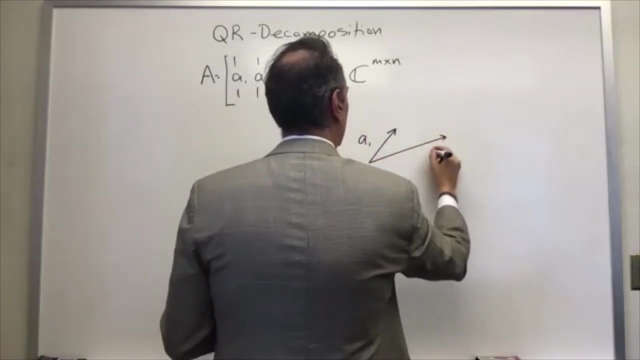 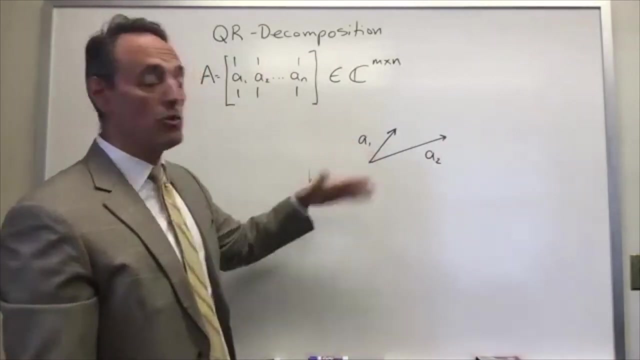 then each one of these column vectors I can use in some sense to define a coordinate space. So let me give you two vectors, for instance. So here's two vectors, A1 and A2.. And let's say I use these as my basic two vectors for defining a coordinate space for a column, So I'm going to say that the column space is going to be some matrix, that is, M by N. Okay, So here's what I want to start thinking about, which is if these are all linearly independent. then each one of these column vectors I can use in some sense to define a coordinate space for a column. Okay, So here's what I want to start thinking about, which is, if these are all linearly independent, then each one of these column vectors I can use in some sense to define a coordinate space for a column. Okay, So here's what I want to start thinking about, which is, if these are all linearly independent, then each one of these column vectors I can use in some sense to define a coordinate space for a column. Okay, So here's what I want to start thinking about, which is if these are all linearly independent. then each one of these column vectors I can use in some sense to define a coordinate space for a column. Okay, So here's what I want to start thinking about, which is, if these are all linearly independent, then each one of these column vectors I can use in some sense to define a coordinate space for a column. 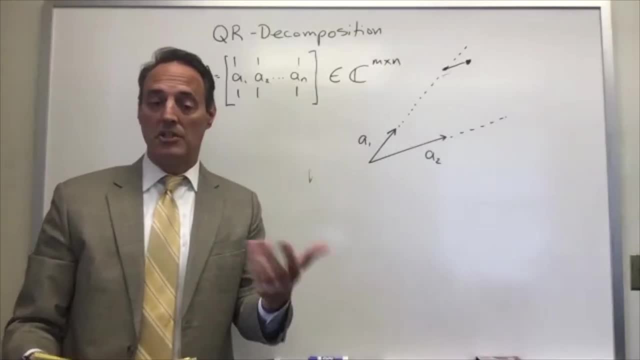 then each one of these column vectors I can use in some sense to define a coordinate space for a column. Okay, So here's what I want to start thinking about, which is if these are all linearly independent systems. this is why we use them routinely throughout all of the sciences is because 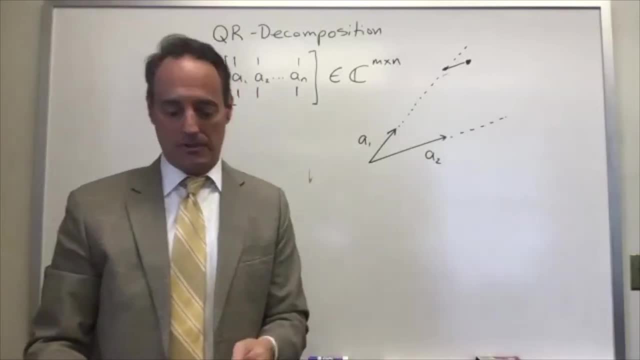 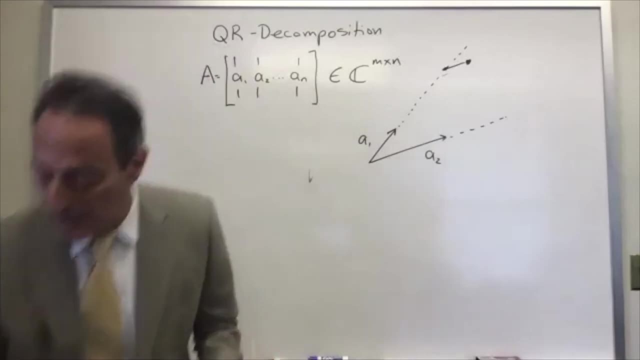 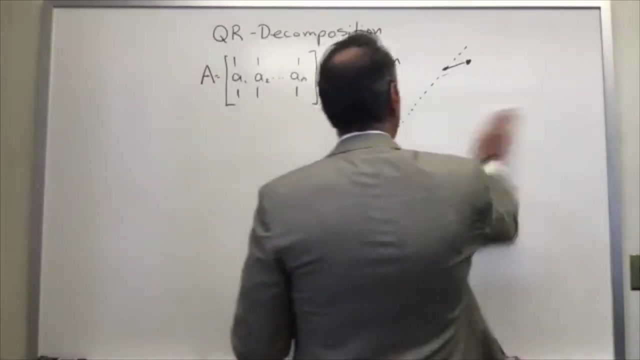 orthogonality really makes things a lot easier, and let me show you how. i'm going to first talk about using non-orthogonal coordinates like this, and then we're going to talk about the advantages of using orthogonal coordinates instead. so this is the idea. is i have an n-dimensional space. 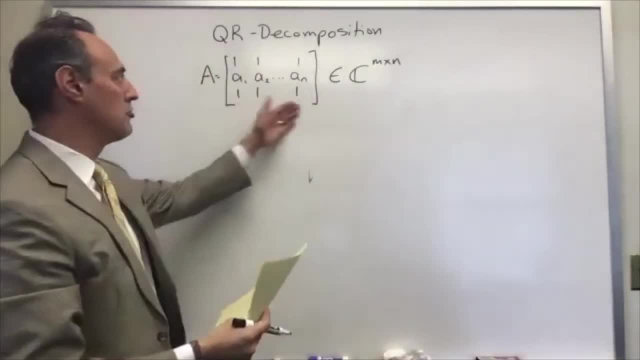 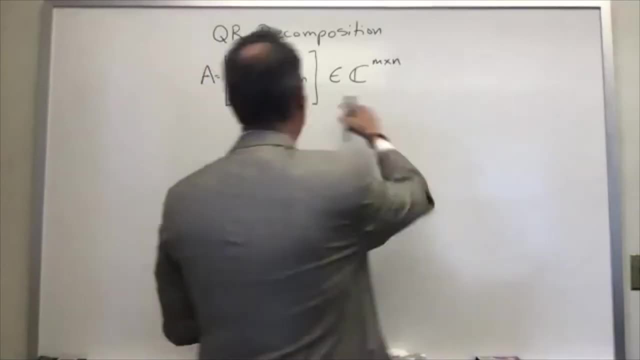 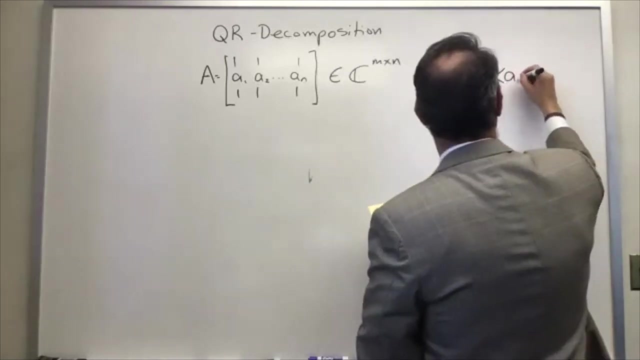 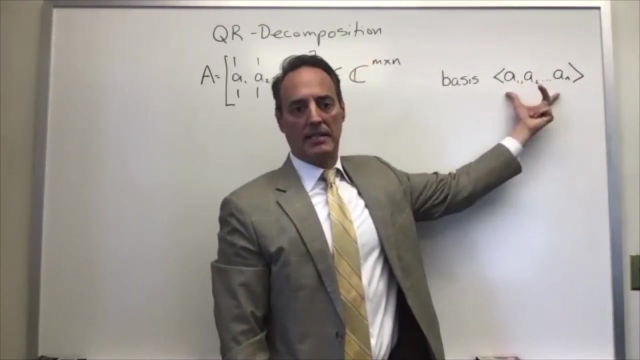 and in this, in an n-dimensional space, i could just use these vectors as as the coordinate system. so i have a given basis and the way i'm going to represent this basis for spanning that space is in brackets a1, a2, all the way to a of n, so this represents the spanning set for the. 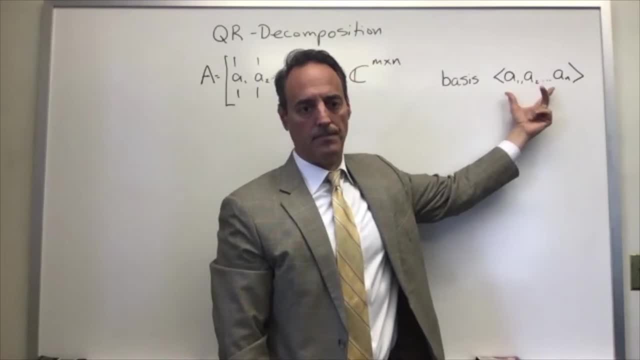 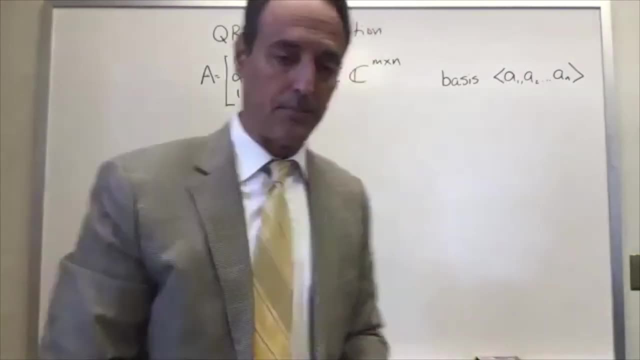 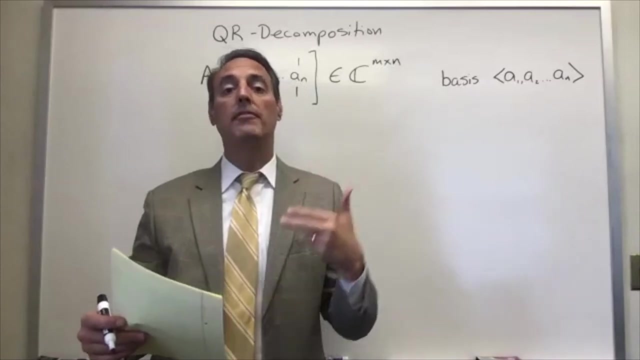 n-dimensional system. okay, all right. so i've n basis vectors, a1 through a of n, and so that's what i'm going to represent with those brackets. so let's take an arbitrary vector and ask the question: how do i represent an arbitrary vector in this coordinate system? right? so the idea is x is equal to. 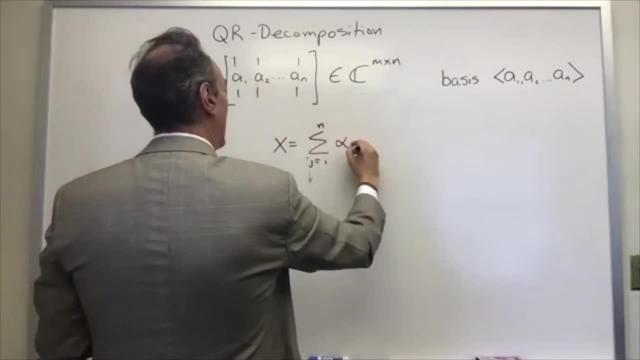 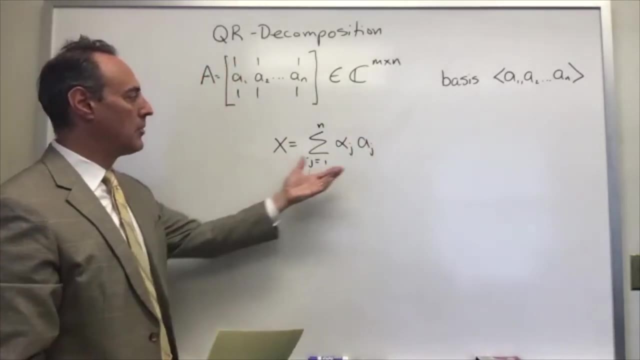 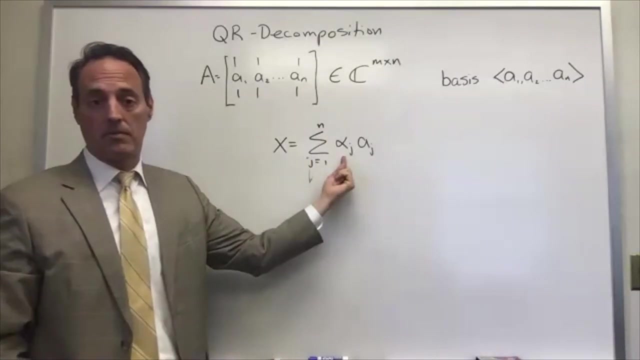 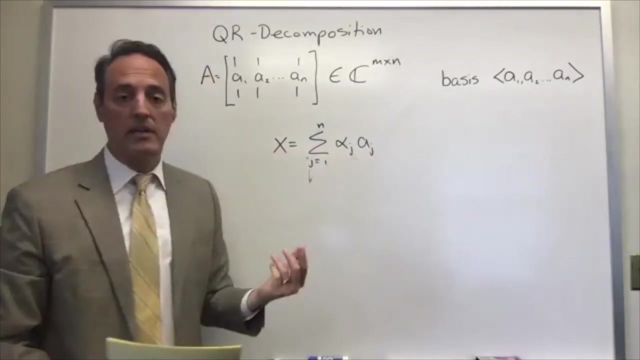 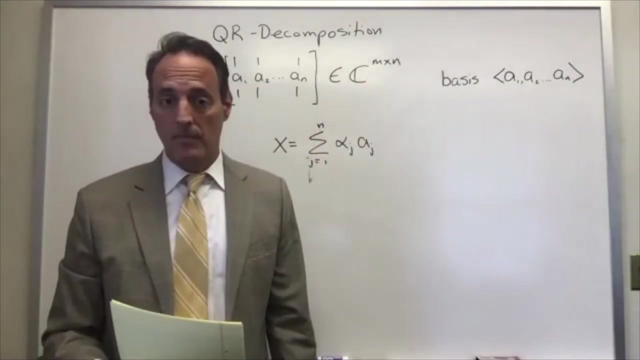 j equals one to n alpha j, a sub j. so in other words, a vector can be written as a sum of all these vectors or these spanning vectors with some coefficient alpha j. so all i need to do to prescribe this vector, given this basis, is determine the alpha j that i would need to uniquely prescribe a point in space. okay, i don't. 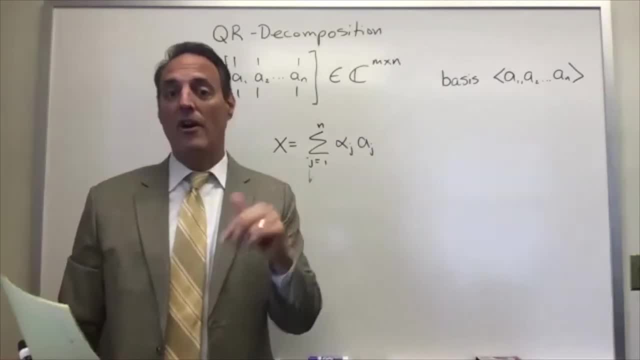 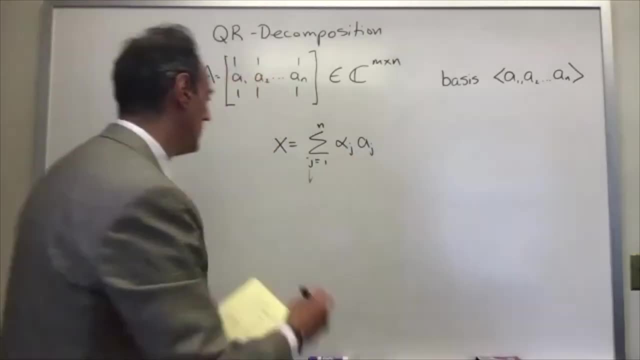 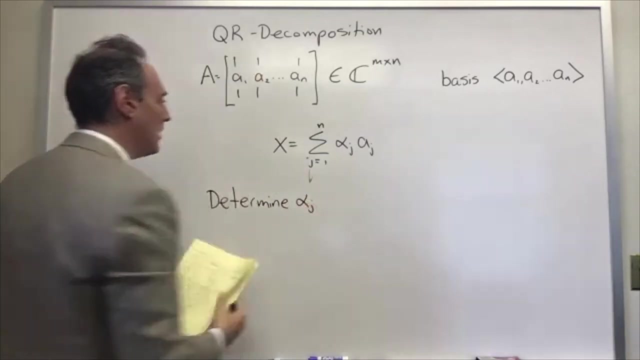 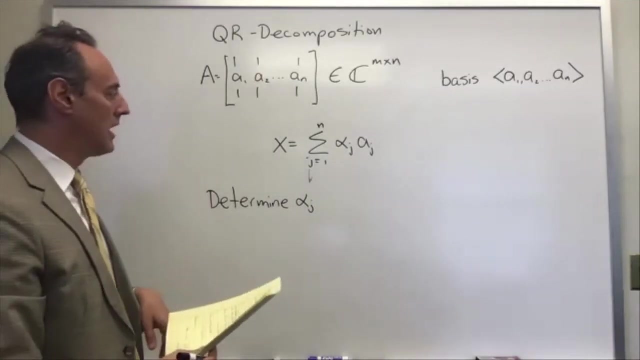 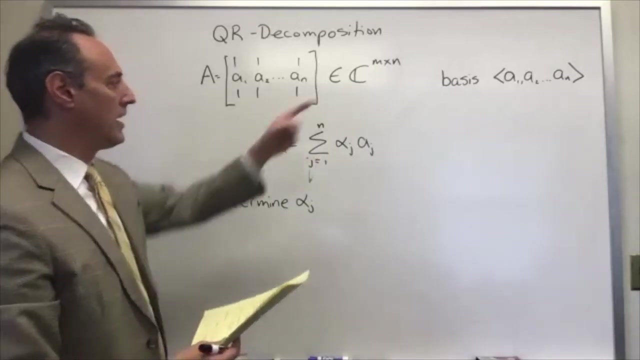 need orthogonality to do this, but you're going to see that orthogonality makes this a lot easier. so let's figure out. how do i determine these alpha? j's okay. one way to do this is basically to take this and multiply each side of this equation by any one of those basis vectors, in other words, 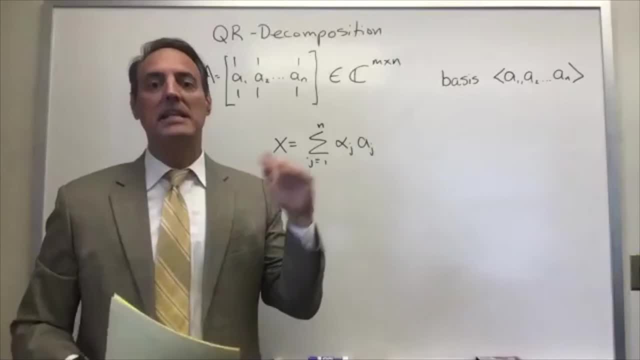 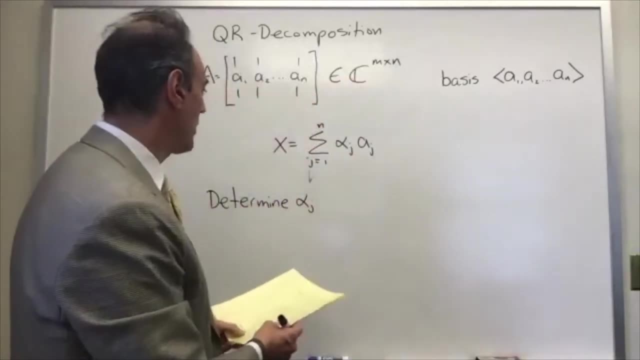 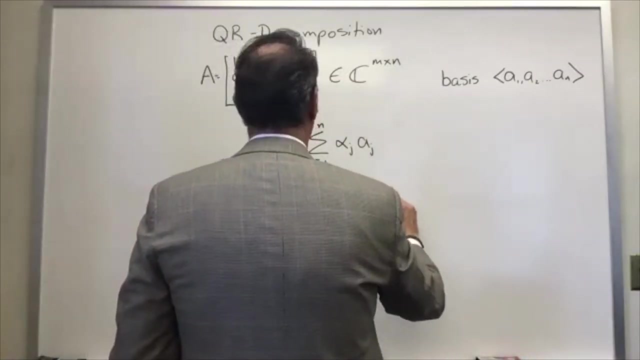 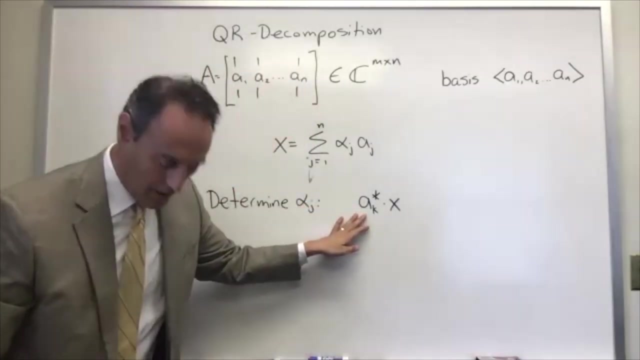 take x and take its inner product onto any one of these basis vectors. okay, so the way you're going to do this is, for instance, let's pick the kth vector, so let's take a of k star dot x. so i'm going to take this, i'm going to transpose it, complex, conjugate it because, in the end, remember this, 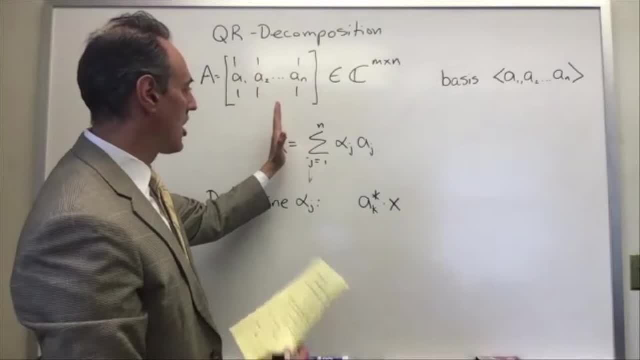 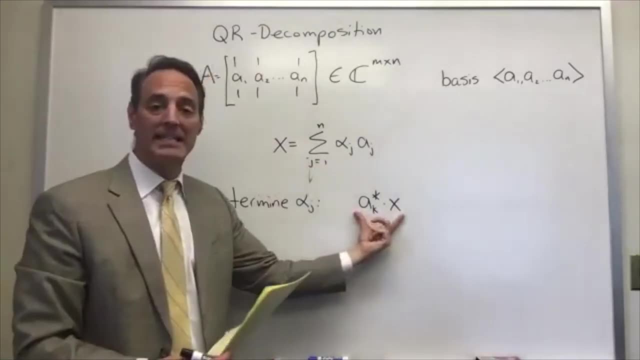 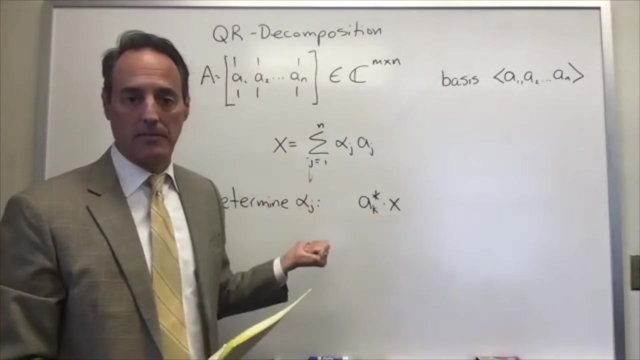 vector x is a column vector, so it's column vector. if i take the dot product, by taking the transpose complex conjugate, now it's going to be a row vector. this is going to be a single number. this is the inner product, in other words the projection of x onto the kth direction. okay, 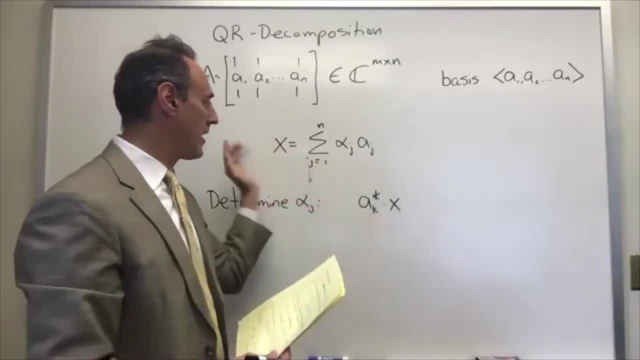 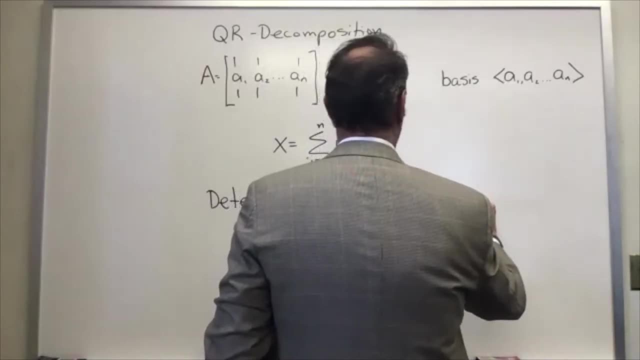 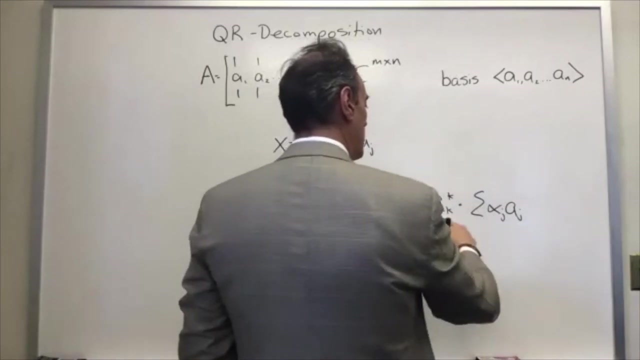 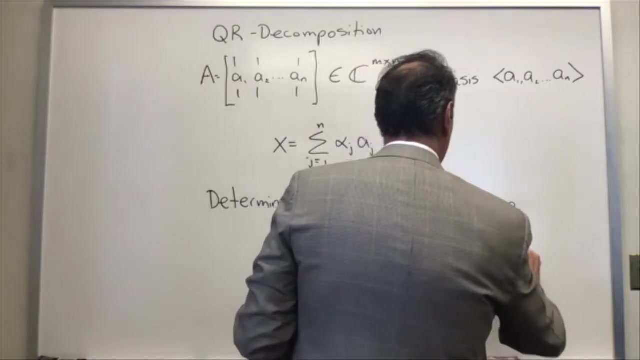 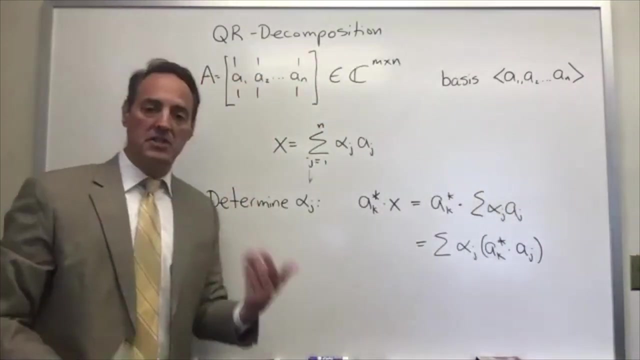 all right. so i take the inner product of both sides equals ak, star dot, the sum of these alpha j a sub j, and so this ak can come in there and then you get a sum alpha j, ak, star dot a of j. so what i just did is i took this x and i took the inner product against one of these vectors. 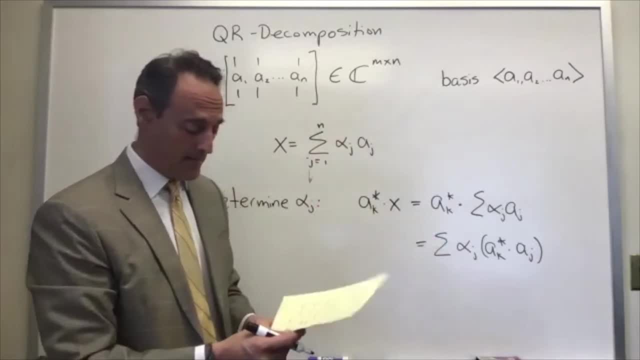 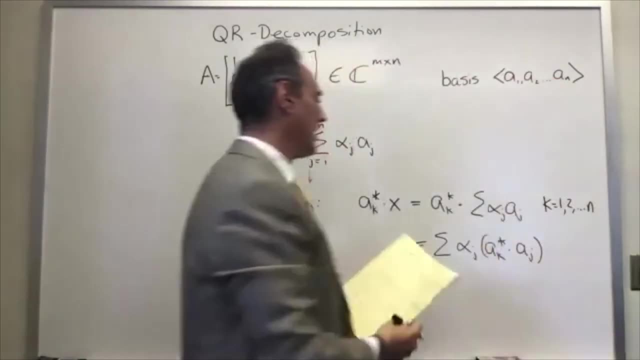 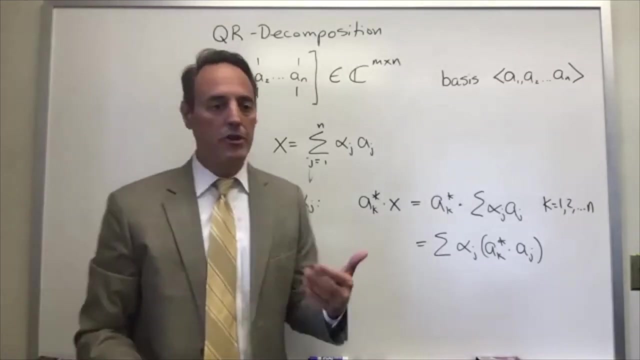 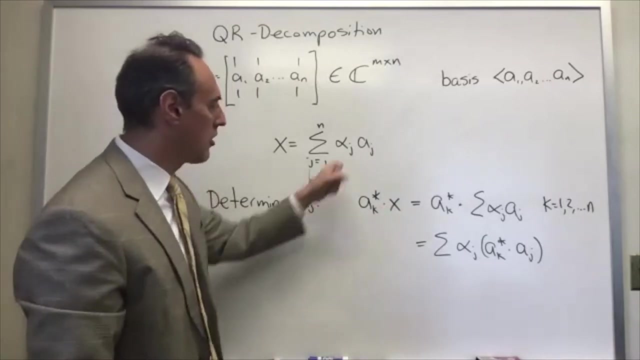 a sub k to produce this. okay, where k is one two through all of the n vectors, all right, and what i'm trying to set up for you is the fact that when i take these inner products against all the k vectors, what it's going to allow me to do is start to determine the alpha j's. 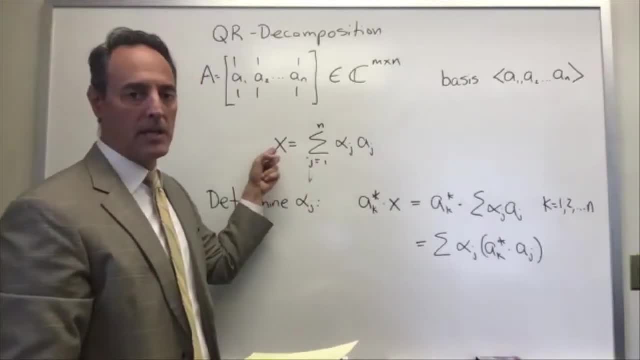 i need to prescribe how to represent x in this basis decirgy. i need to determine the alpha j's. i need to describe how to represent x in this basis setup where k is one, two and four to all of the n vectors. okay, deixae, here's the example: lever k, number 2, and p. and when i have k, 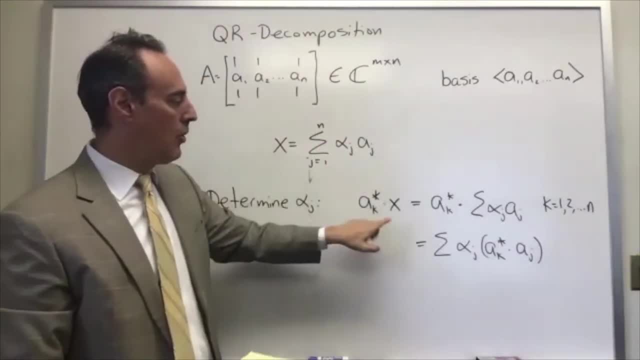 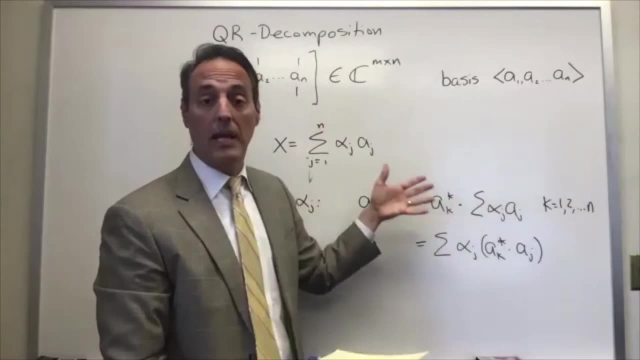 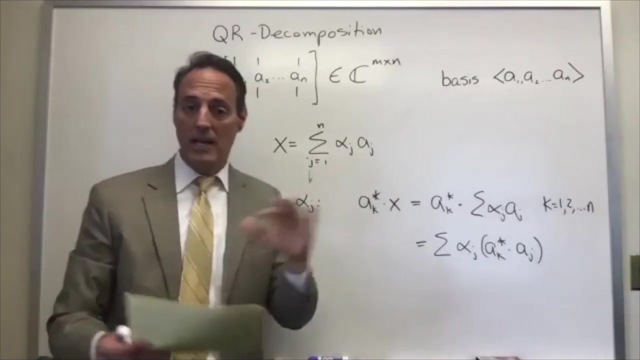 is set a sub, j's okay. so this is one set of equations, but i have for each k and i've n of them. so i'm going to get k. i'm going to get n equations and i actually have n unknowns. so what i'm going to actually get out of this is n equations and unknowns that i'm going to allow. 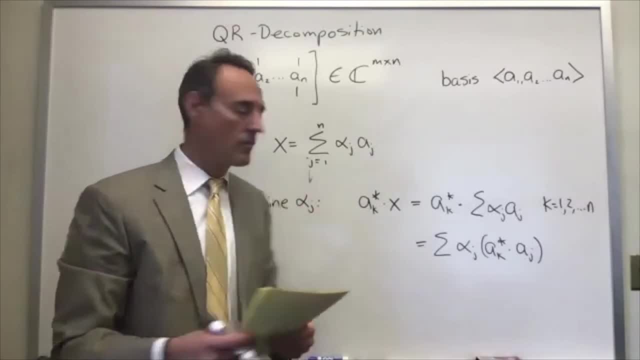 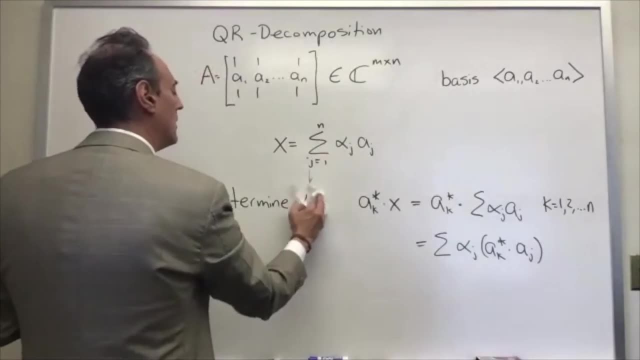 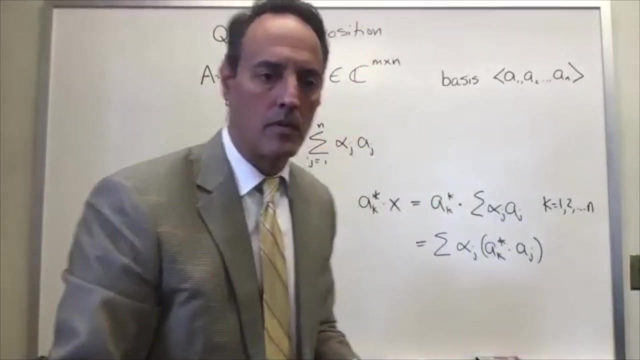 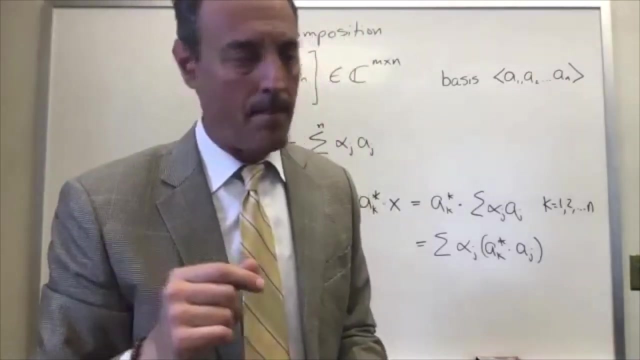 me to solve for each of the alpha j. all right, so let's do that. you're dropping this, all right, um, professor, just a question. yes, uh, so if each ai is of length m, how could n of them spend cn? excuse me, what's your question again? oh, i mean, um, if each of these ai vectors are of length m. 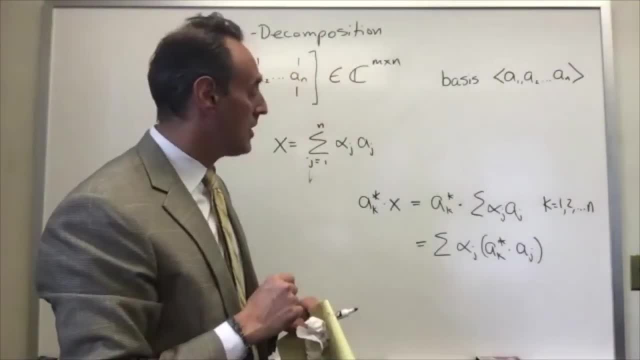 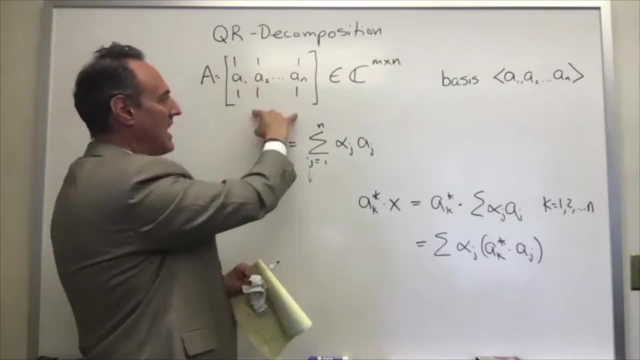 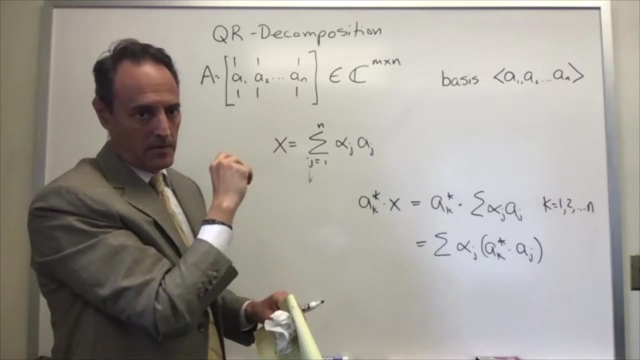 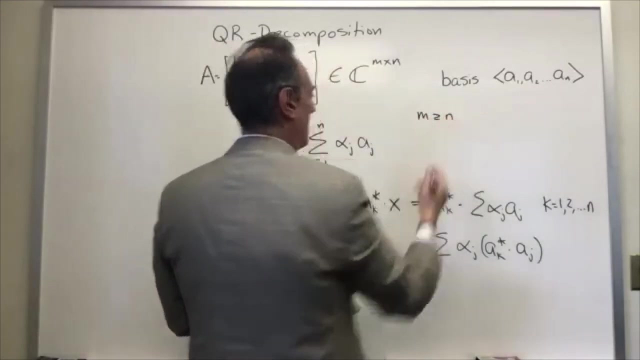 then how could n of them spend cn? um, um, this is m by n, right? so this is length m. there's an n dimensional space. so you're saying n is smaller than or less than or equal to m. yeah, that's right. so so okay, m is bigger than or equal to n. 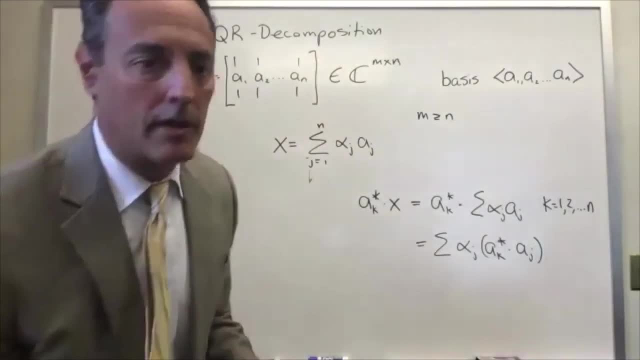 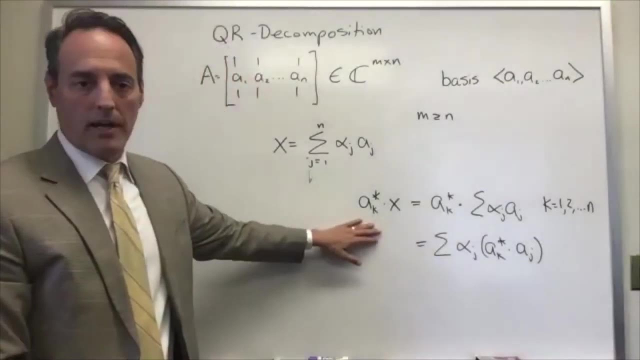 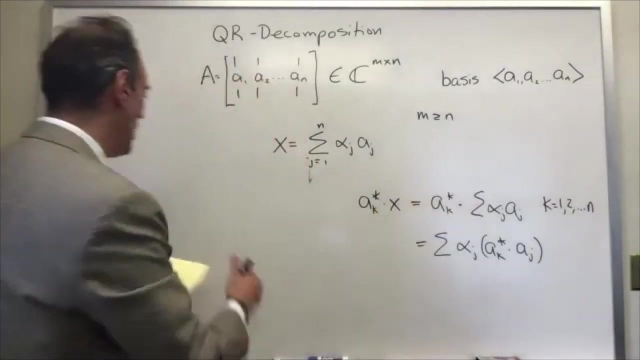 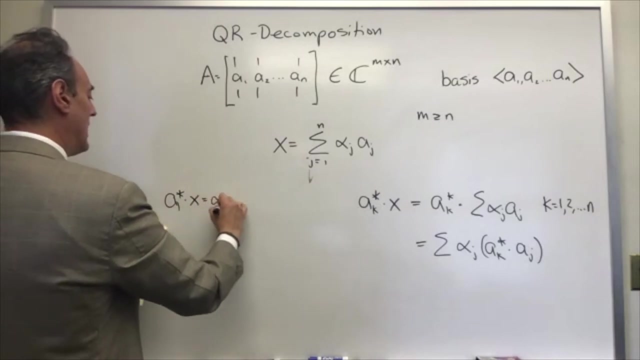 i see, yeah, and what we're going to do. sorry, should have put that up earlier. okay, so if i do this in a product, so for instance, i go and do this instead of afk, i do a of one, let's take a one across here. what you're gonna get is a1 star. time dotted with x is equal to alpha one. a1 star. 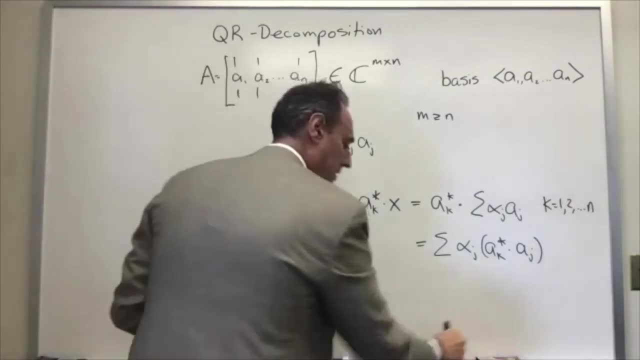 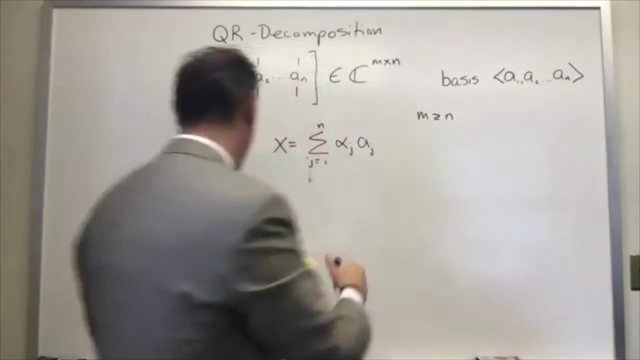 dot a1 in fact. let me just write some of these out. this will be hopefully a little bit more clear as i write all these equations out, just want to make sure you have it very well in mind exactly what we're doing. so let's do an a1 star for a1 star and then, if i do this in a product like 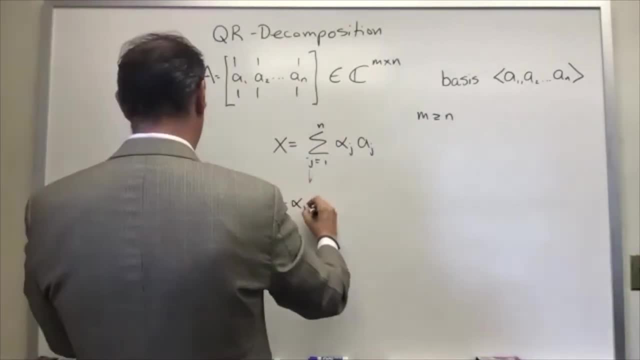 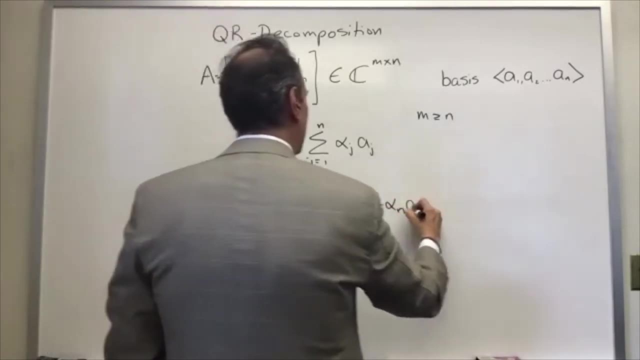 alpha one: a1, star dot a1. uh, alpha a1, that's equal to alpha. i'm going to write some of these out. this will be hopefully a little bit more clear as i write all these equations out. just want to make sure you we're doing: plus alpha 2, a1, star dot a2, plus, plus, plus, all the way to alpha of n, a1, star dot a of n. 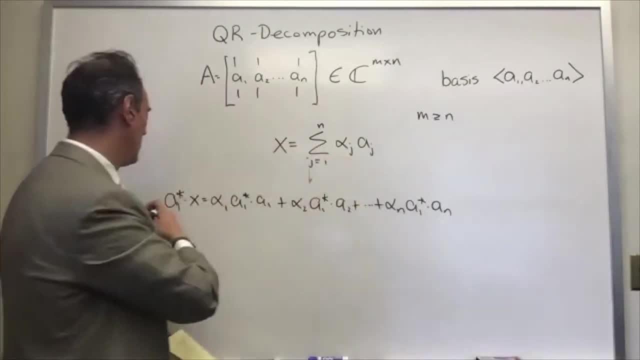 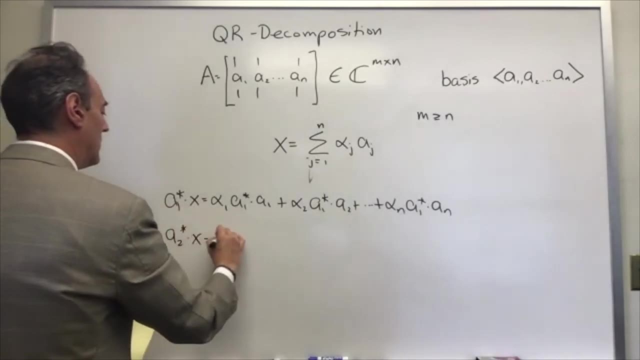 so, in other words, when i take the dot product on both sides with a1- that's the first equation- when i do it with respect to a2 star, i get again alpha 1 a1 star dot- um, sorry, that's a2 plus alpha 2, a2 star dot, a2 plus. 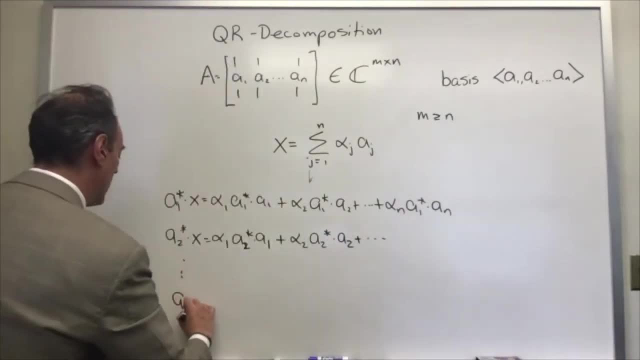 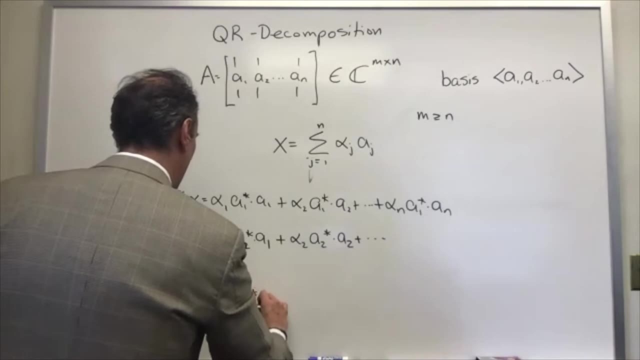 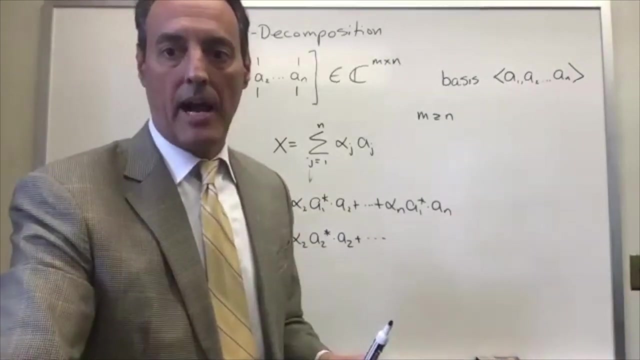 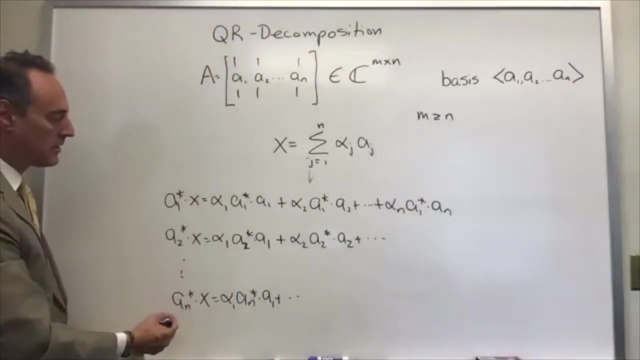 all the way up, all the way down to an star dot x. so you go alpha 1 and star dot a1 and so forth. okay, so that's what we have, uh, going on with this here. so we get n equations with n unknowns. i could write all of this in matrix form this: n equations, n unknowns. so this is going to be. 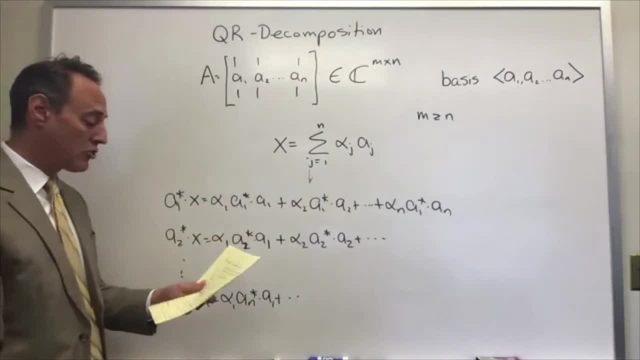 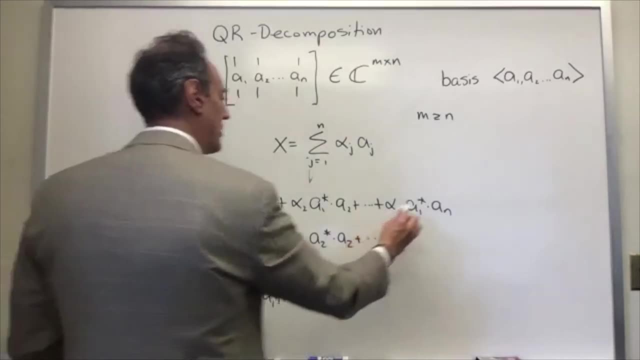 an ax equal to b problem by itself, and so let me try to write this out. so if you write this out in matrix form, you're going to get an ax equal to b problem by itself. so if you write this out in matrix form, then here's what it's going to look like. let me shrink this down a little bit here, because i need 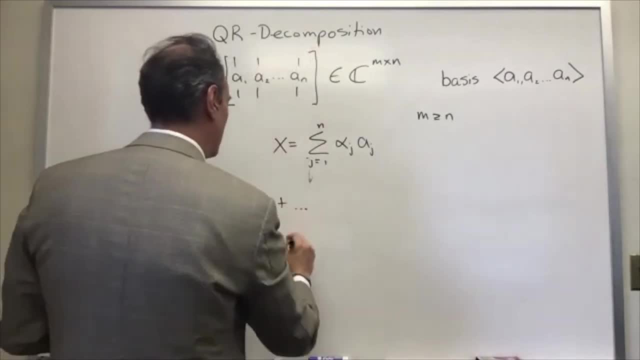 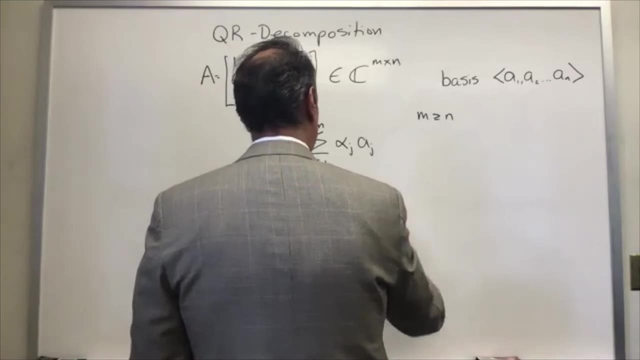 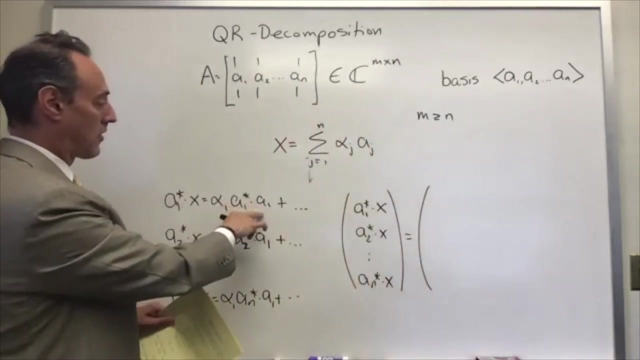 some space. these are all dot dot dots, so what you're going to get, then, is the following: a1- star dot x. a2- star dot x. all the way to an star dot x is equal to the matrix that you construct, and here are the terms of the matrices: 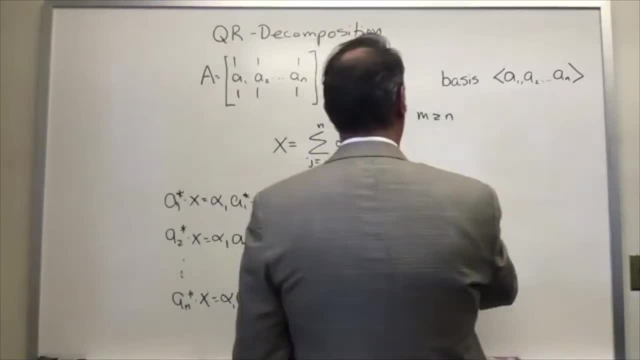 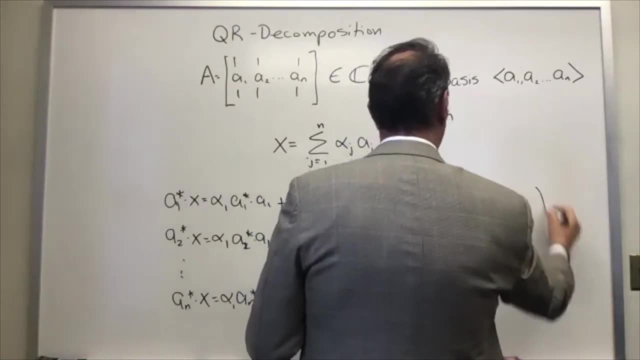 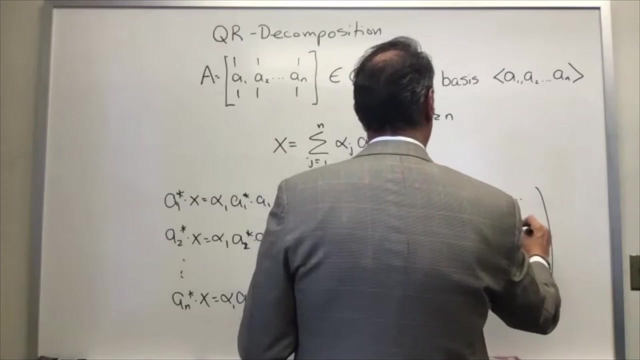 they're, they're all these inner products. so you have a1, star dot a1, a1, star dot a2, and so forth, then a2, star dot a1, a2, star dot a2, all the way to an star dot a1, and so forth. 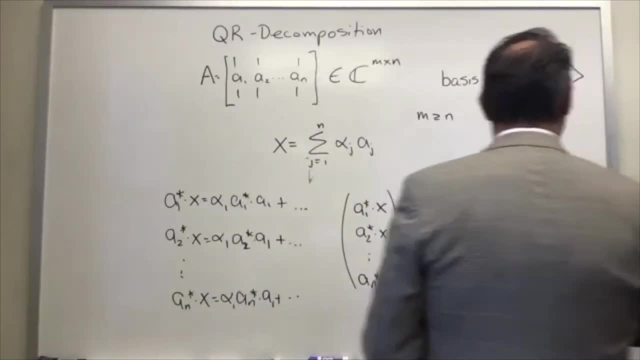 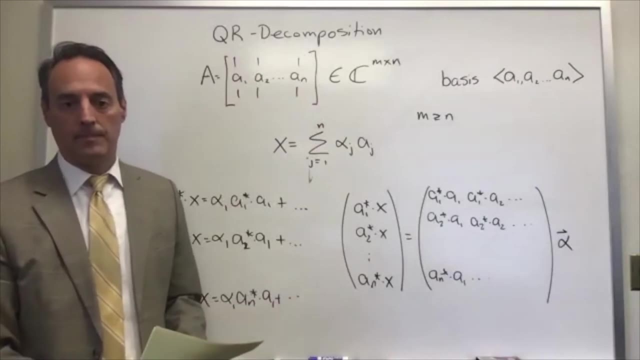 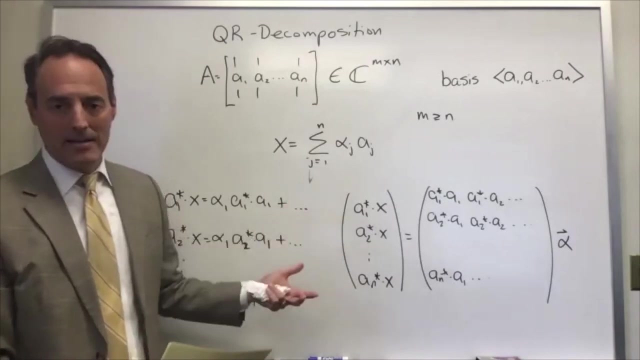 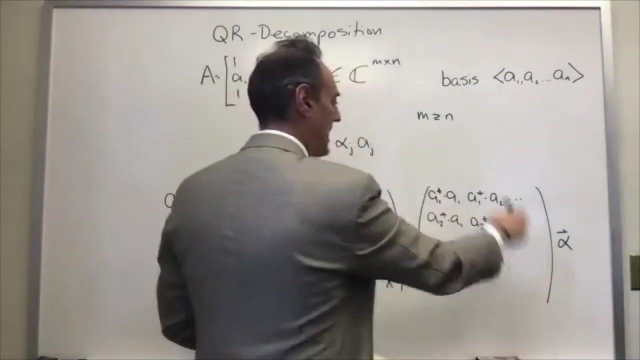 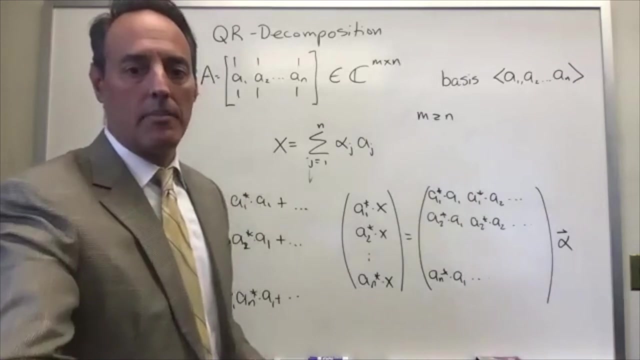 and then here you get the vector alpha. the vector alpha is the alpha of the vector alpha one, alpha two, all the way through alpha n. so this is a linear system of equations which is an n by n, whose solutions are the alpha vector. okay, so this is how i determine the alphas: is, through this set of n, linearly independent? 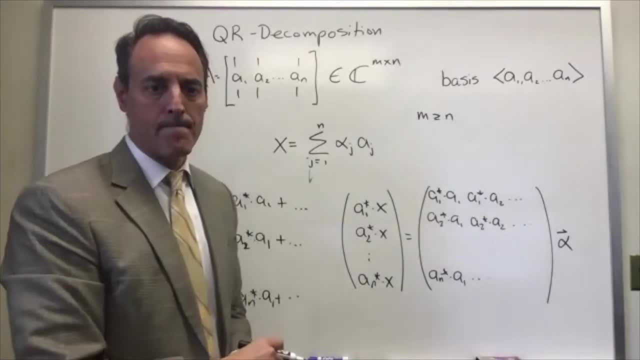 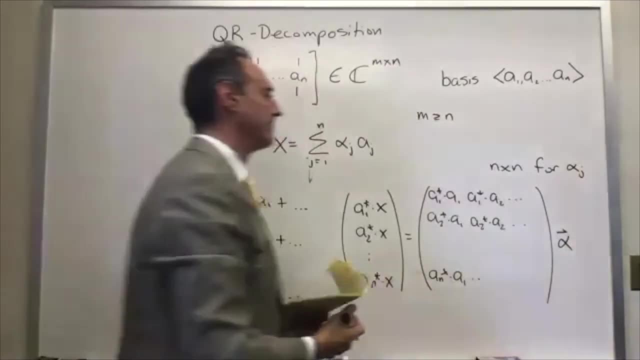 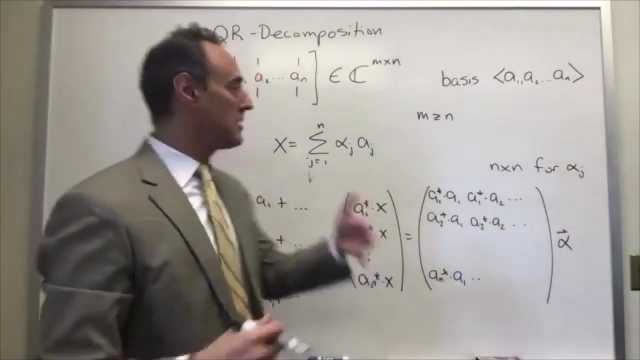 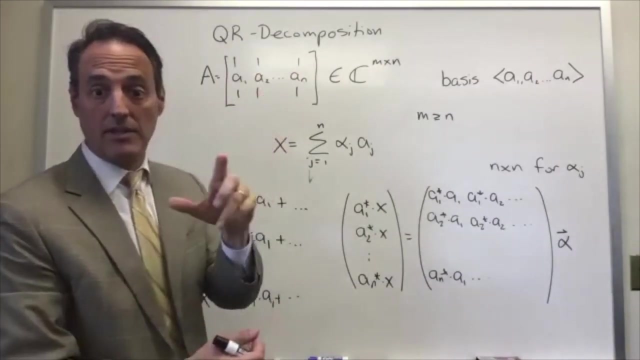 equations. okay, so this is n by n ーン. this is m by m. this is the first set of n, so we're saying that i get that from the back Gong. what is the position of the vector then? we can't get the sum of this by one. 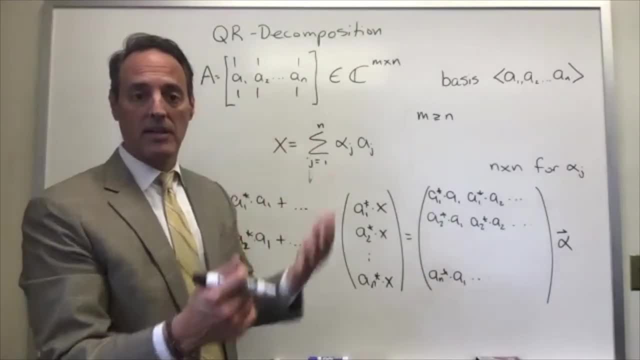 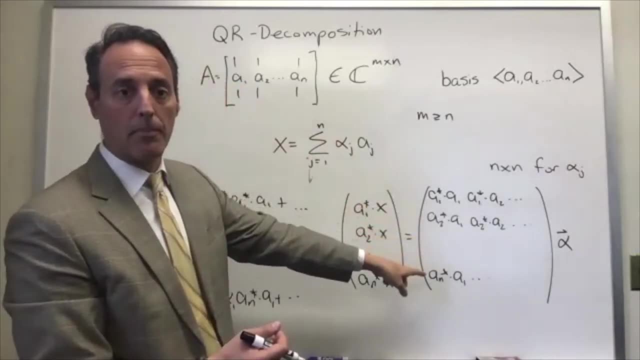 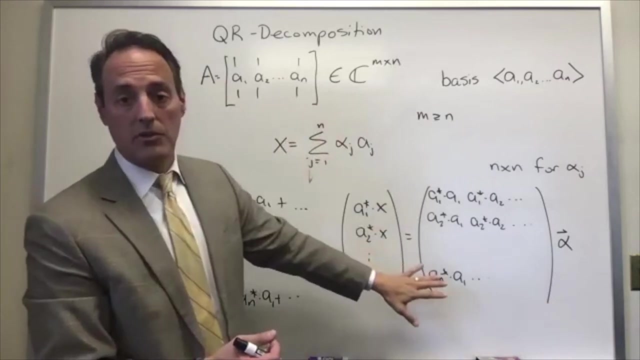 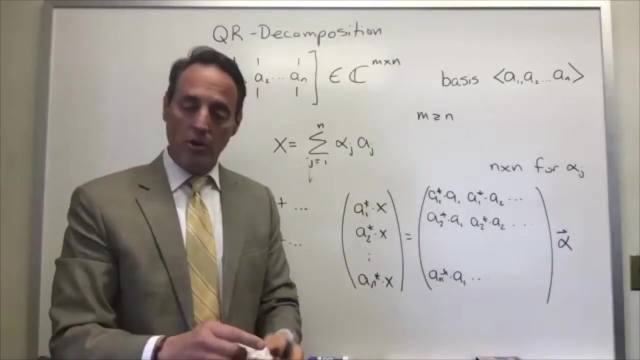 which is b, xr has root, 2 is v into n. in this space you can determine its location uniquely by solving this ax equal to b problem right there. and since, in fact, these are linearly independent, this will always have a solution. okay, now notice what i've done. i've just used any column space i want. right, if i do this here. 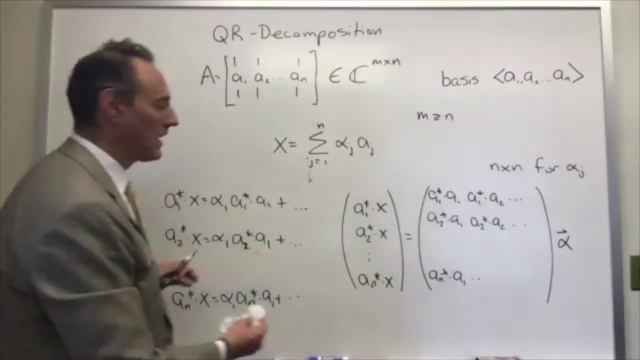 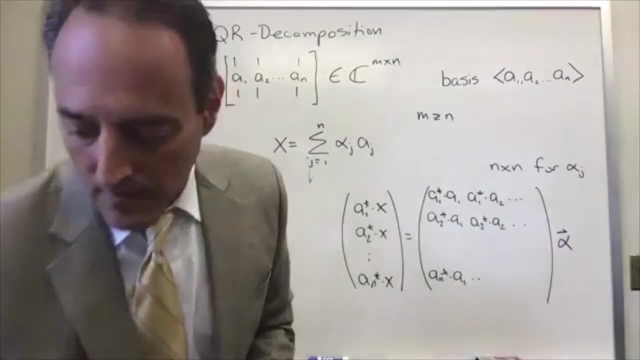 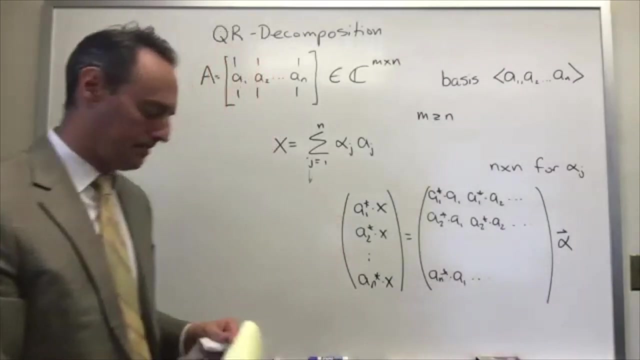 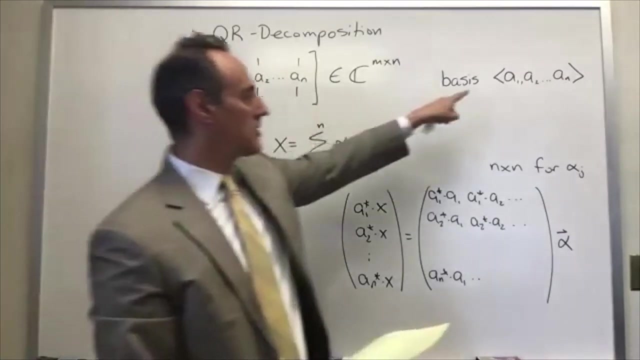 the column space is n dimensional. i just did this calculation out. i get this, but i want to highlight something very special that happens if i start to be a little smarter about what i'm doing in using bases in particular. here's what i want to do: what if, instead of using the basis a1 through a of n? 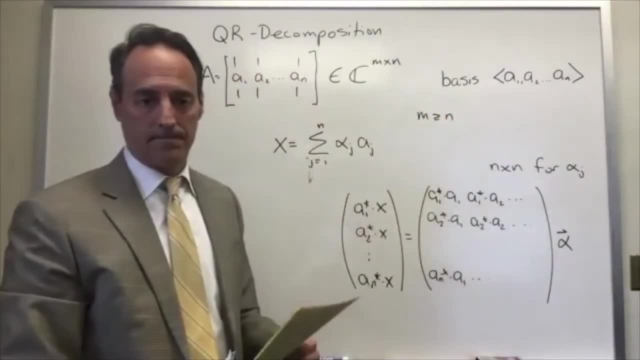 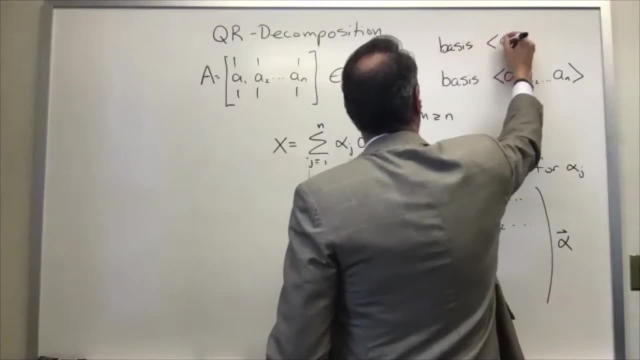 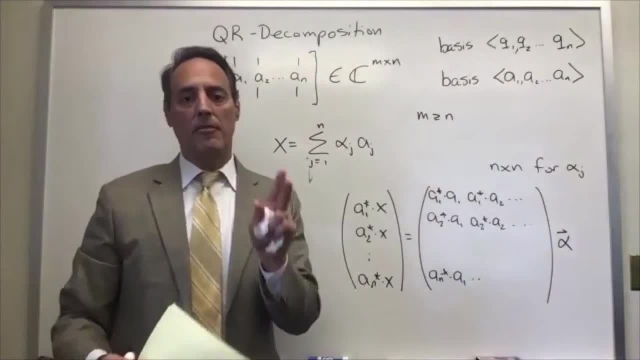 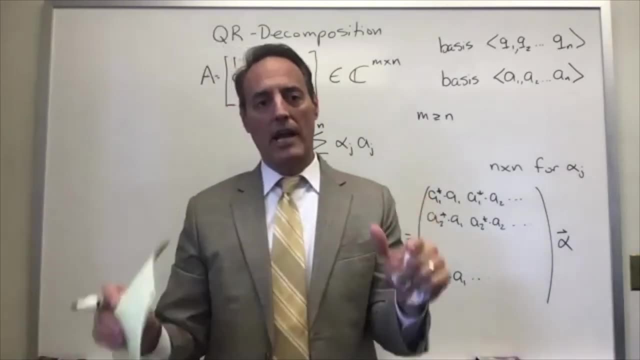 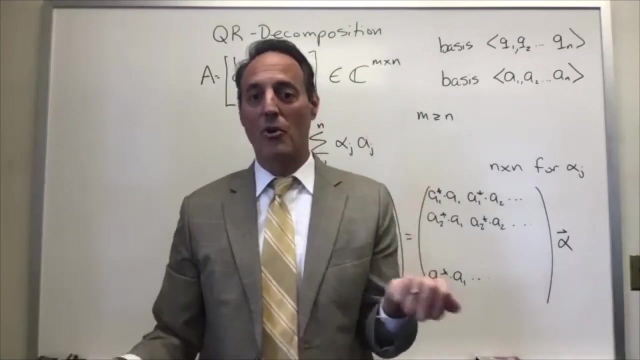 in other words, i want to pick a different basis, and here's what i want to have happen. in this basis: i want orthogonality. okay, so oftentimes in physics, this is why we use orthogonal coordinate systems- is because there's a great advantage of using an orthogonal coordinate. 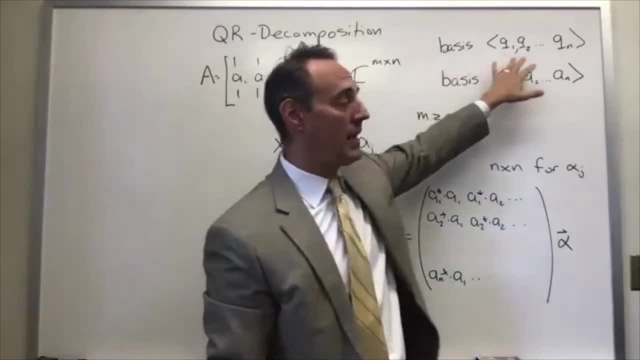 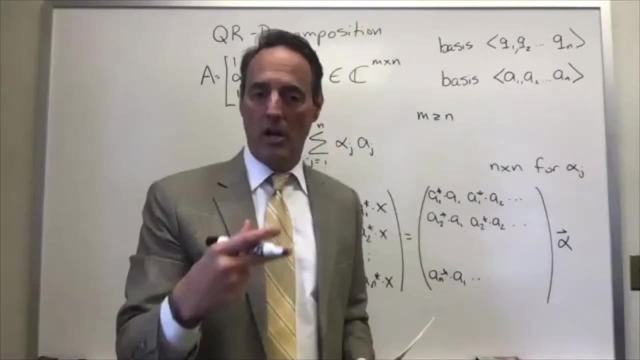 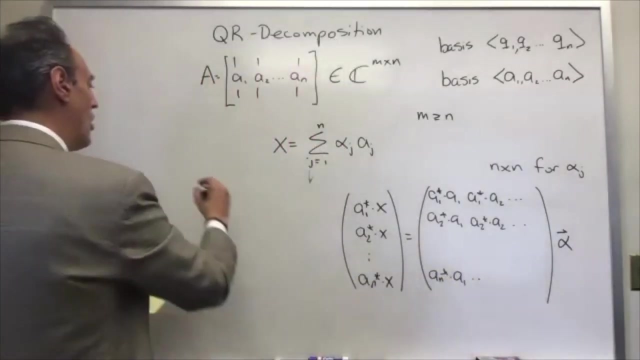 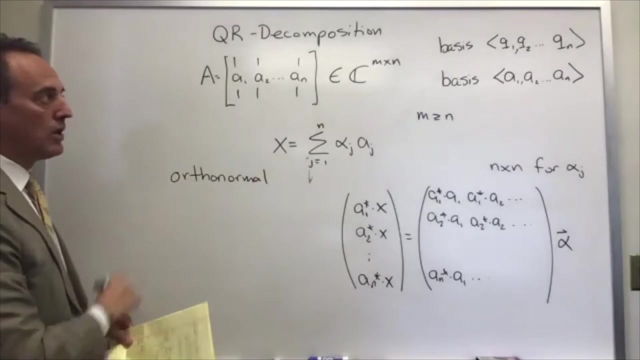 system, and so what i want to do is figure out what if i picked an orthonormal set- not just orthogonal, but orthonormal, so not only they're orthogonal, but they're unit length. so here's what we're going to do: we're going to think about an orthonormal set q1 through q2. 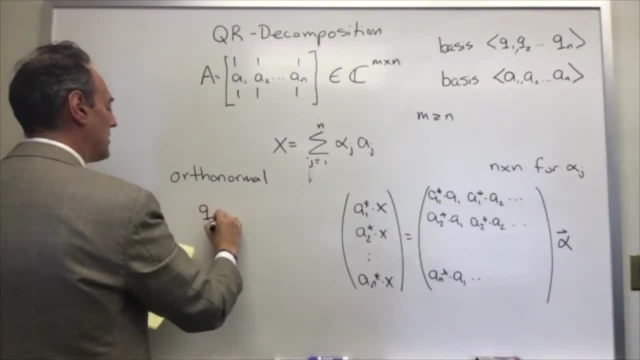 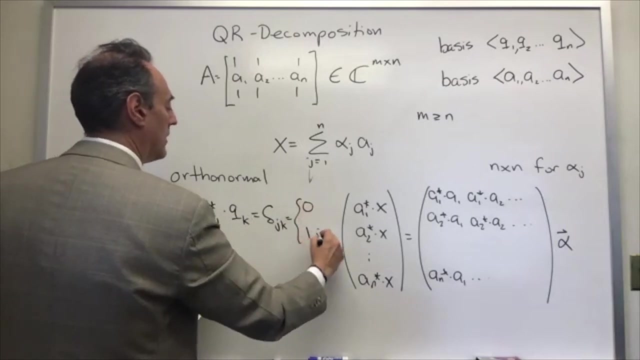 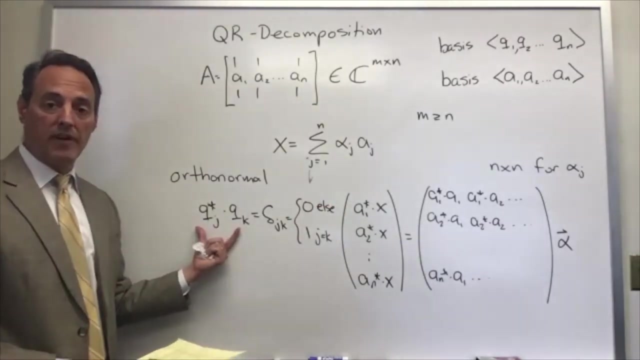 of n. in other words, what this means is: q of j, star dot q. q of k is equal to the dirac delta function, which is zero or one. so in other words, the inner product between any of these two vectors is zero when j is not equal. 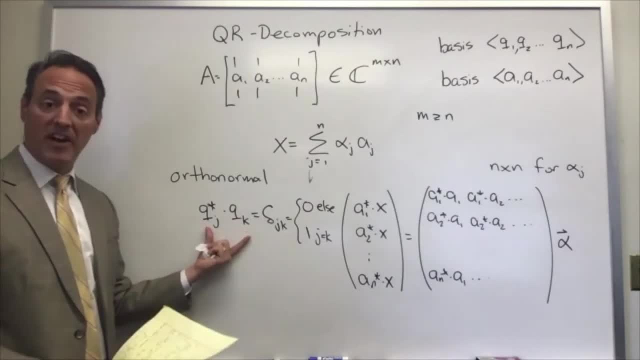 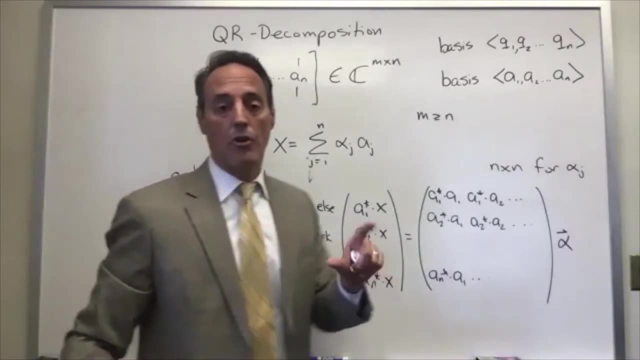 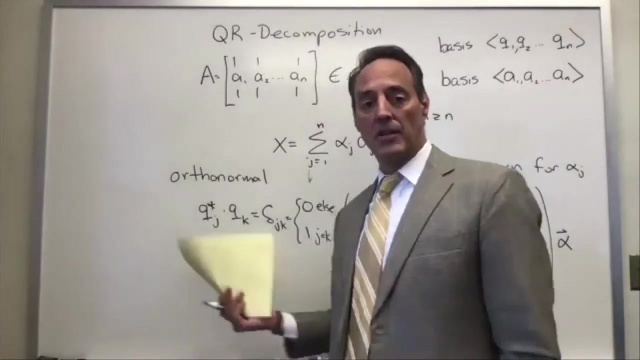 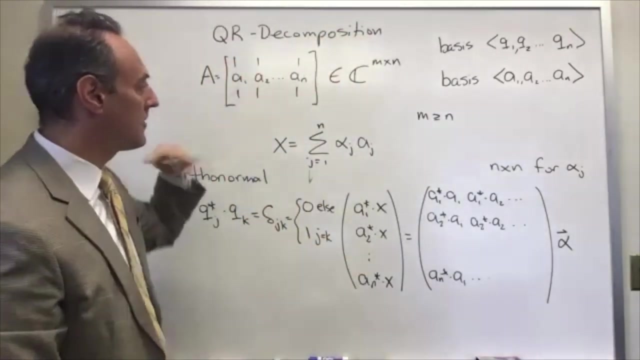 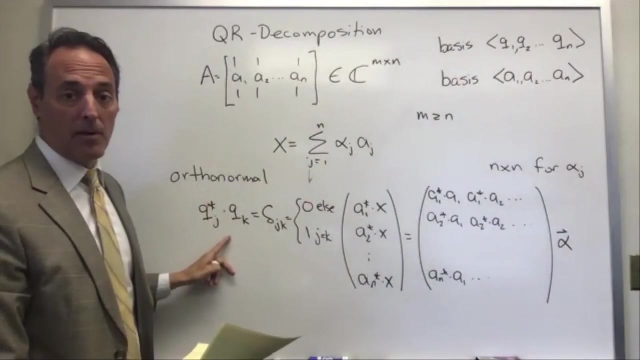 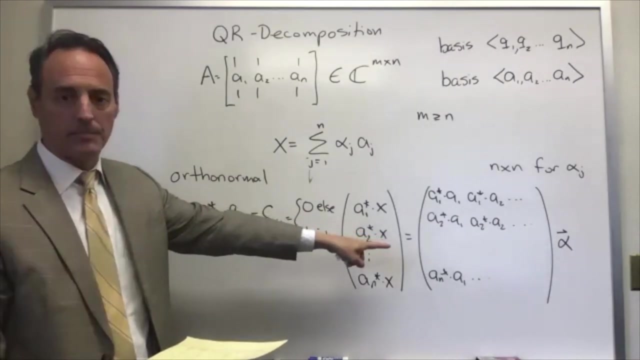 to k, but when j is equal to k, it means only someone else is equal to q mark. only someone can know that who they are. so the tool itself is a finding, the. The question then becomes: what would happen to a calculation such as this. OK, let's talk about it. 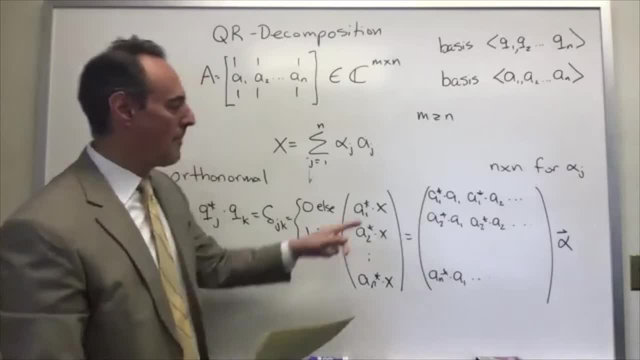 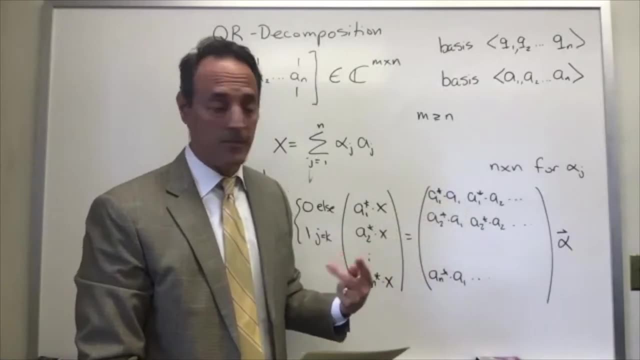 There's great things that would happen. So imagine, each one of these A's- A1,, A2, so forth- are Q1,, Q2, and so forth. OK, so in other words, instead of A1 here I have Q1.. 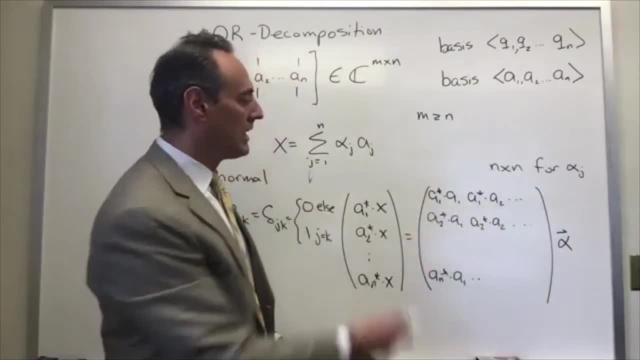 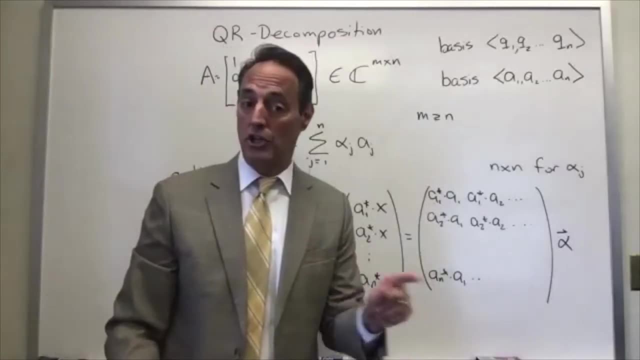 Instead of A2, I have Q2.. So first of all, let's look at this matrix And on the diagonal I have A1 star A1. In other words, this would be Q1 star Q1 if I use those as a basis. 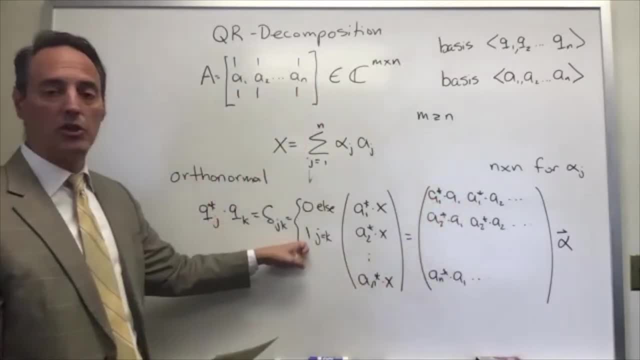 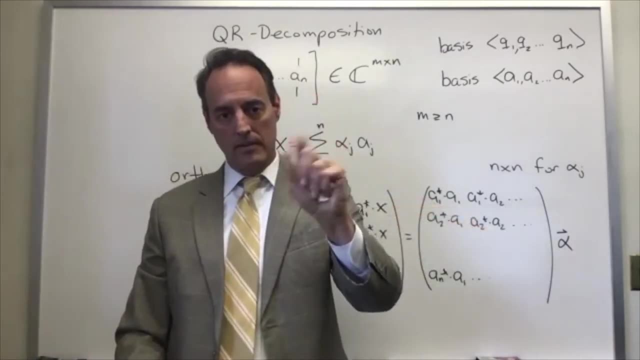 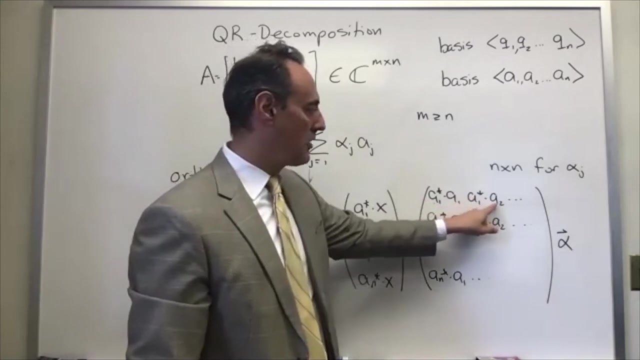 Well, Q1, star, Q1, that would just be unit length. In other words, all the diagonal terms would be 1.. What about the off-diagonal terms? if I was using this orthonormal set, I have A1, star, dot A2.. 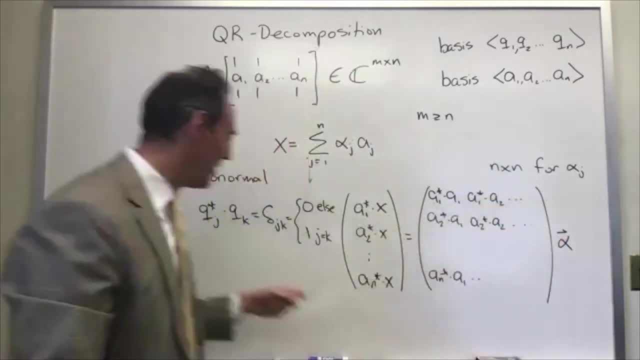 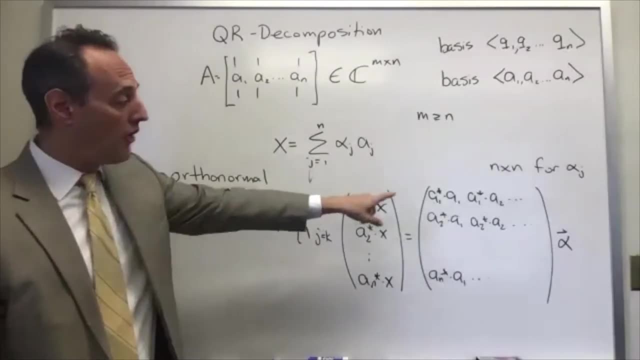 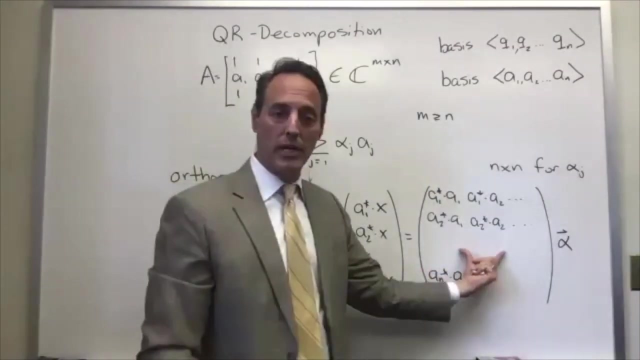 And then A1, star dot A3, and so forth. Well, when j and k are not equal, the inner product is 0. So all the off-diagonal terms would be identically 0. So this entire matrix collapses to the identity matrix. 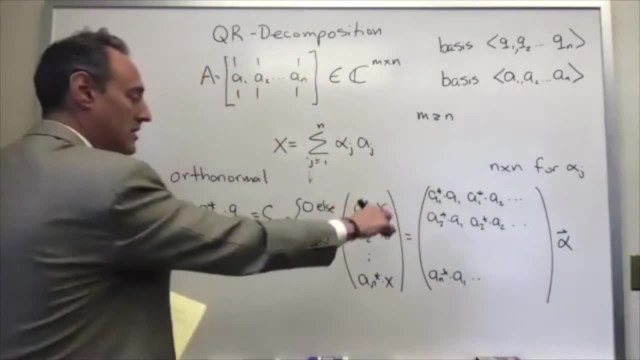 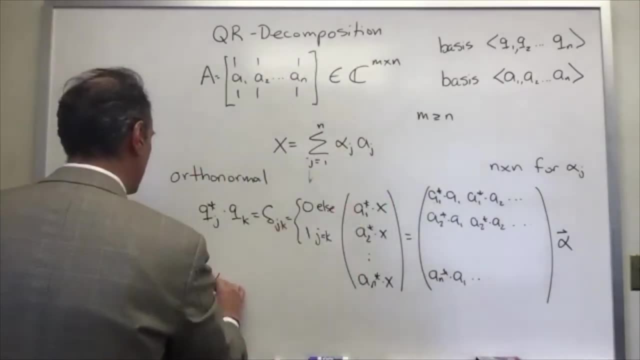 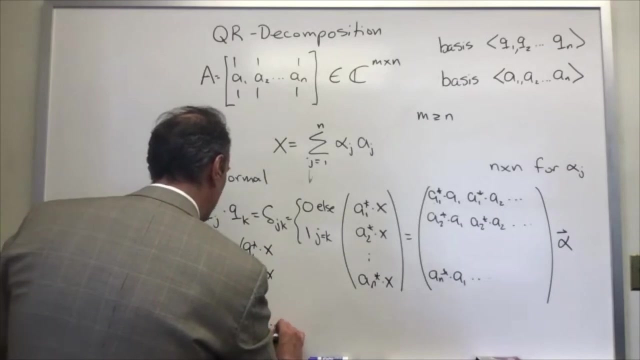 So let's write this out: If you're using this coordinate system, this matrix right here becomes identity times, the vector alpha, And on the right-hand side then you have Q1 star dot x, Q2 star dot x, all the way to Qn star dot x. 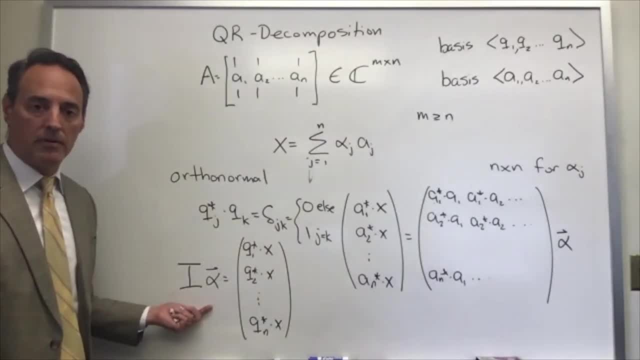 But this is trivial to solve, Because now what you have is because of this structure, you'd have alpha 1.. And alpha 1 is equal to this, Alpha 2 is equal to this, Alpha 3 and so forth, And alpha n is equal to this. 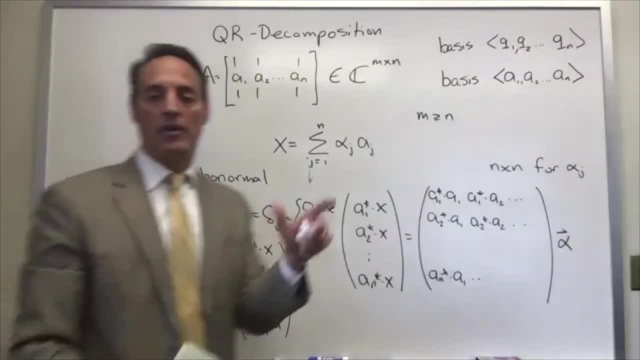 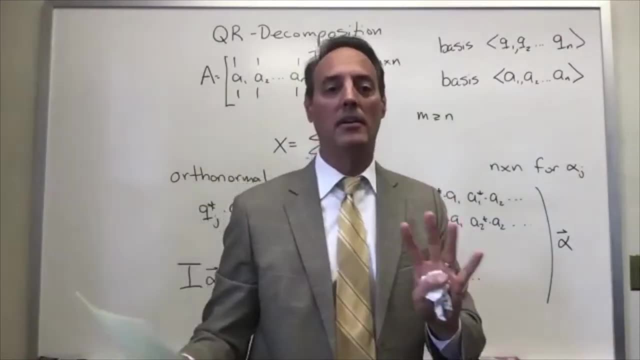 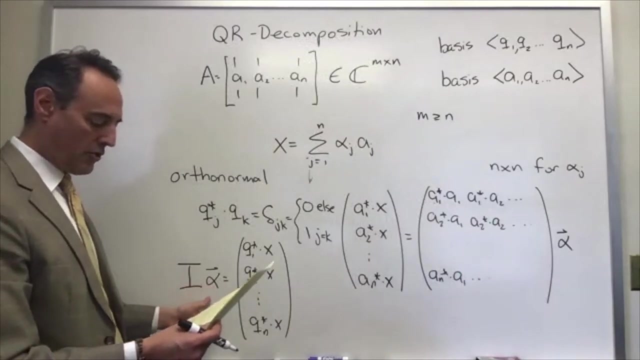 Because it's a diagonal matrix, trivial to solve. Diagonal matrices are fantastic. If you can reduce things to diagonal matrices, usually somehow you've won and you've done a great thing for the problem, okay. So that's what's so important here. 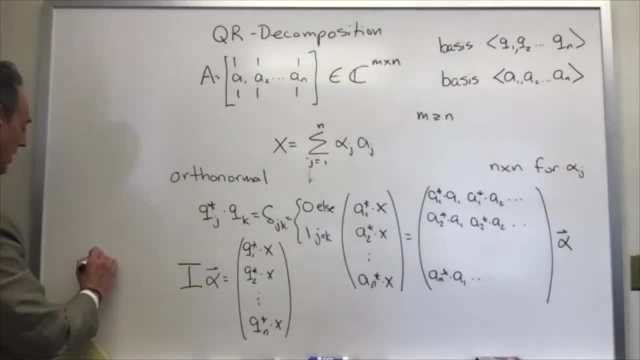 In fact, once you do this- let me write this over here- you'd find: alpha 1 is equal to q1 star dot x. alpha 2 is q2 star dot x, all the way to. alpha n is equal to qn star dot x. 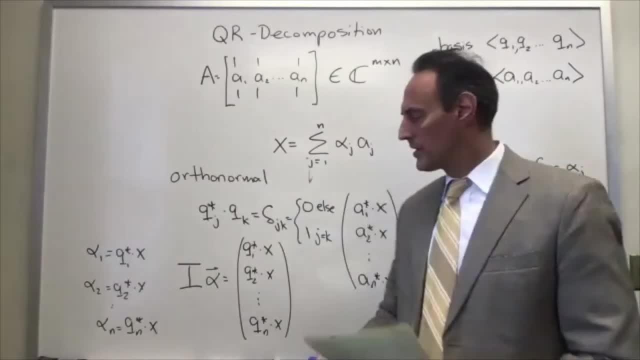 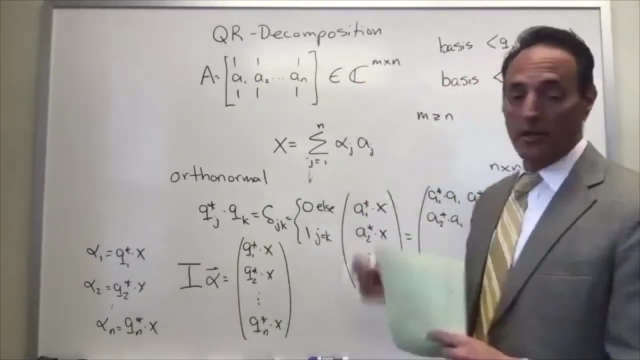 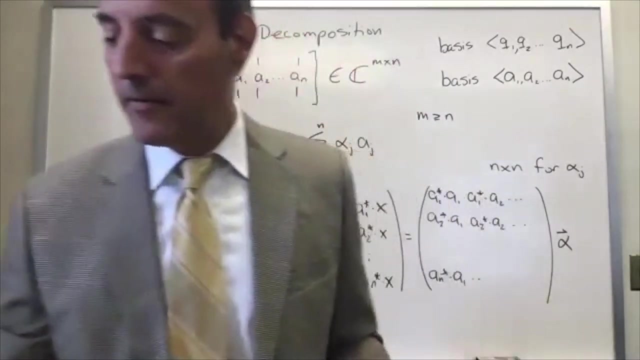 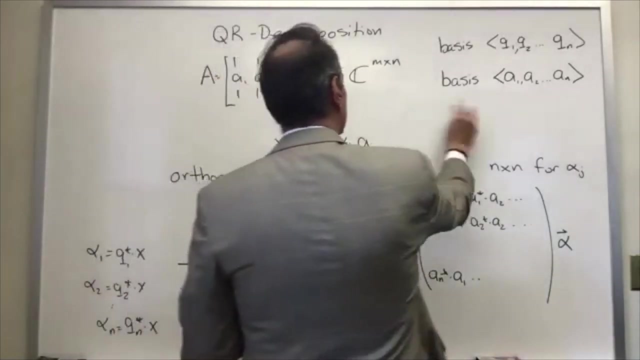 So now, if I have an orthogonal coordinate system, it's very easy to figure out how to represent a solution in a coordinate system. Okay, so this is why we love orthogonality. There's all kinds of nice properties to it In particular. let's come back to this representation here. 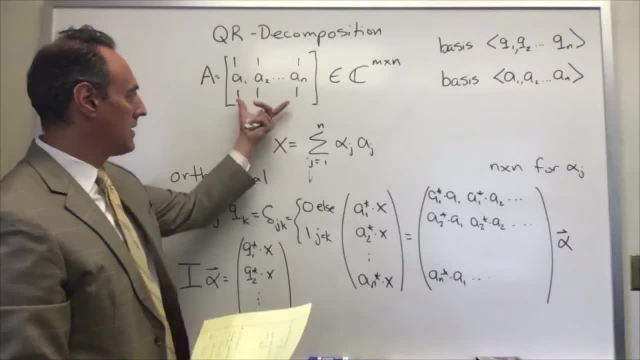 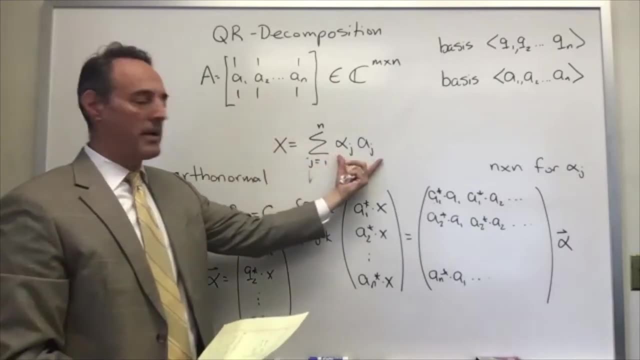 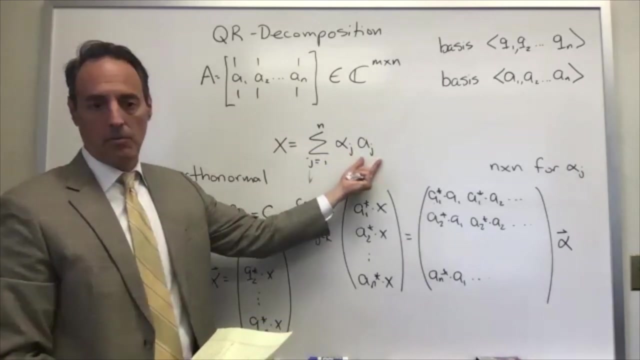 I can represent any vector x in this, in this space, with linear independent and linear independent vectors as a sum given by here, which is just basically some parameter alpha and a projection onto each of the different directions And, of course, if they're not orthogonal. 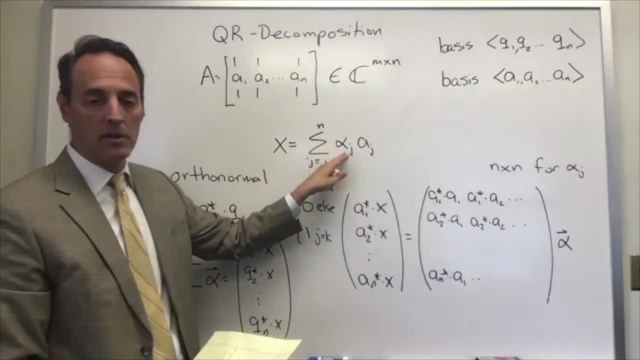 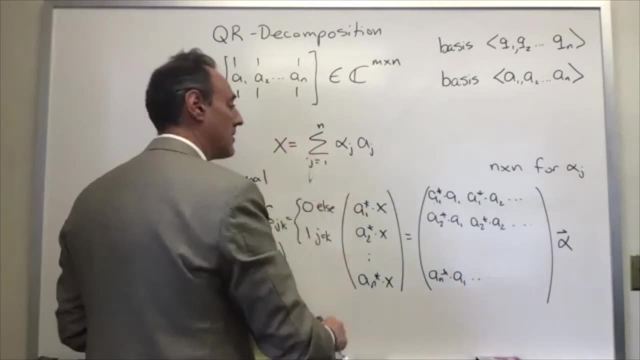 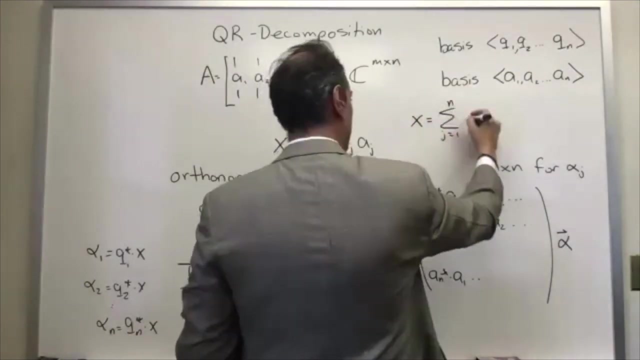 I got to go calculate this n by n system to produce these values of alpha. However, if instead I said: how about? if I represent x in terms of an orthonormal basis, I get alpha x is equal. to notice what I'm doing now? 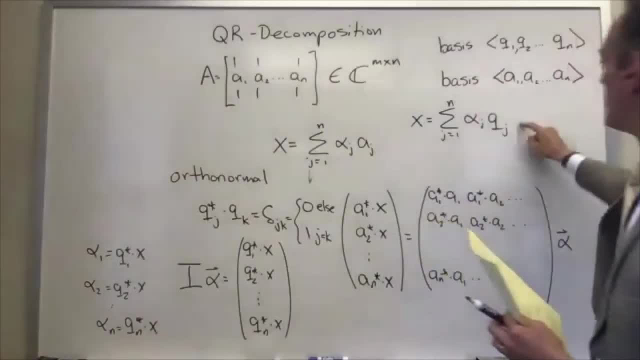 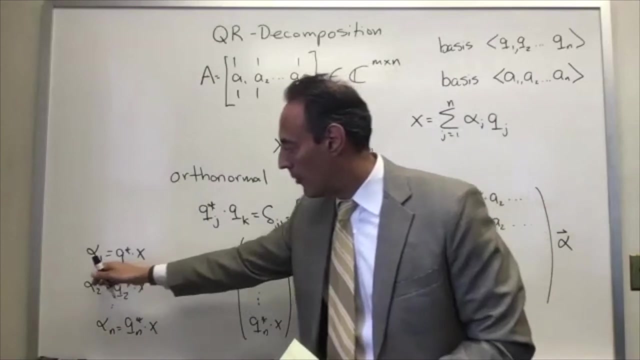 I'm representing these in terms of these new basis vectors q of j, And these are orthonormal And what I just showed you is the alpha j in this basis are given by here. Look at them, There they are. Alpha 1 is q1.. 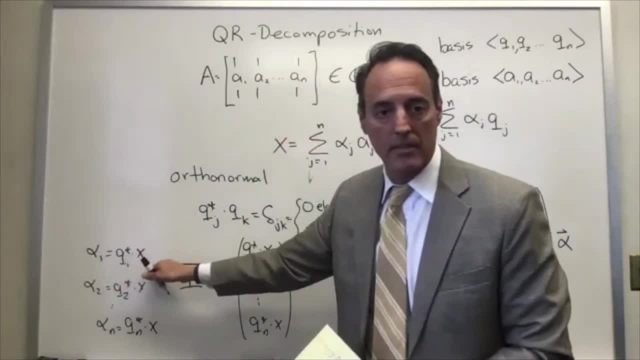 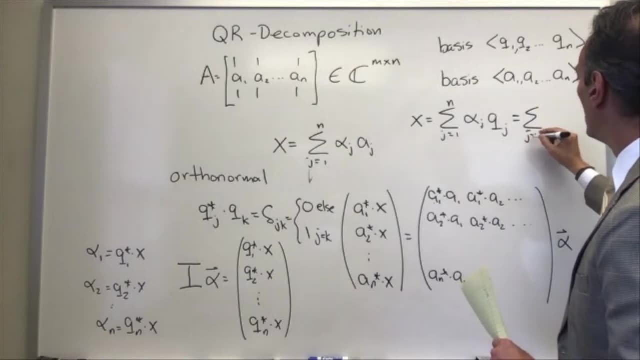 So alpha j is equal to q1.. 2j star times x. So really this is very easy to work out. which is j equals 1 to n. The alpha j right are given right there: q sub j. star dot x. q sub j. 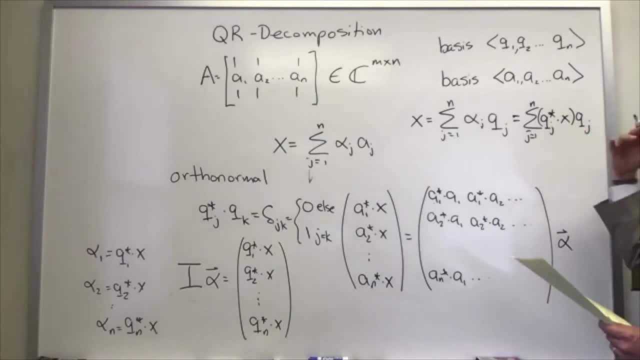 That is my expansion. This is the way I'm going to move from a non-orthogonal coordinate system to an orthogonal, and instead of solving an n by n system of equations for the alpha j here here, all I do is project that vector x into each of the different directions. 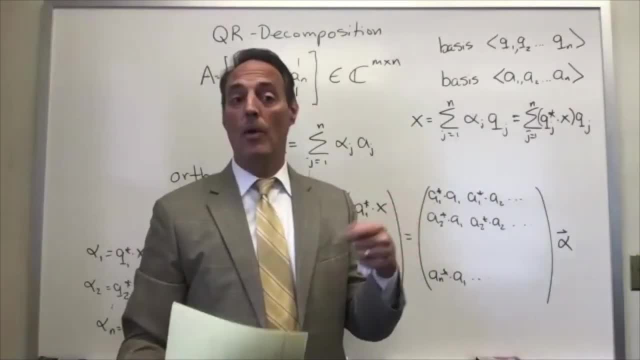 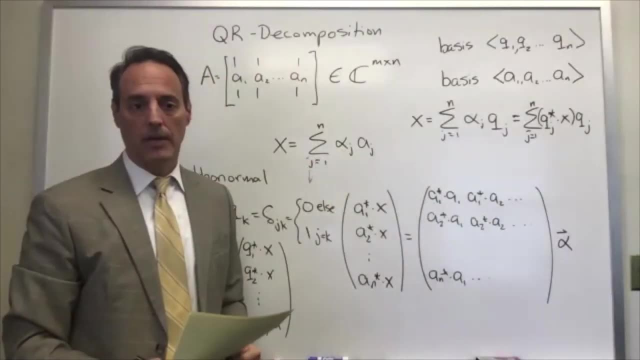 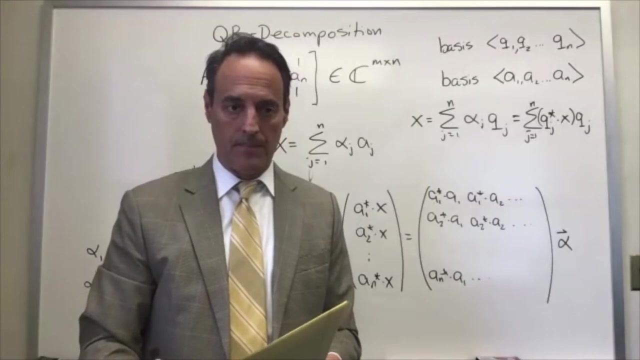 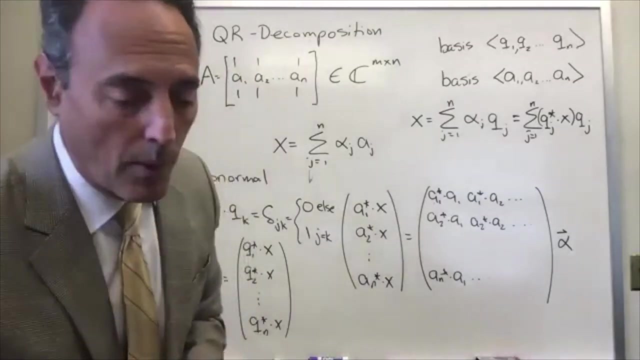 I solve a bunch of one by one problem. I solve n one by one problems to get the solution versus an n by n problem. Okay, So that's what orthogonality is going to give you All right. So this is starting to set up what we want to start thinking about with the QR decomposition. 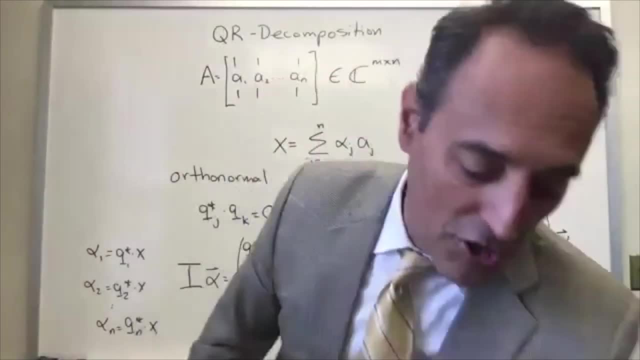 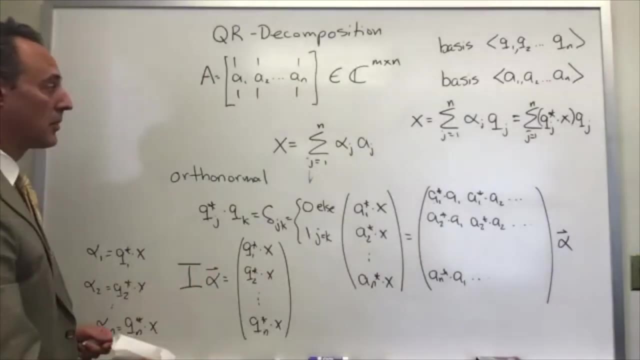 And the QR decomposition. many of you have seen a version of it through Gram-Schmidt's orthogonalization, So I'm going to keep developing this method, but I'm going to go ahead and erase this and we're going to continue on. 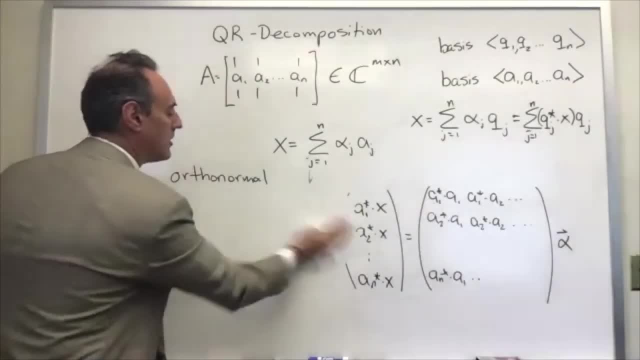 Okay, So that's the sort of math. Okay, So that's the sort of math. Okay, So that's the sort of math. All right, Let's go ahead and erase this. Let's go ahead and erase this, And then we're going to take the math around orthogonality and projections onto basis. 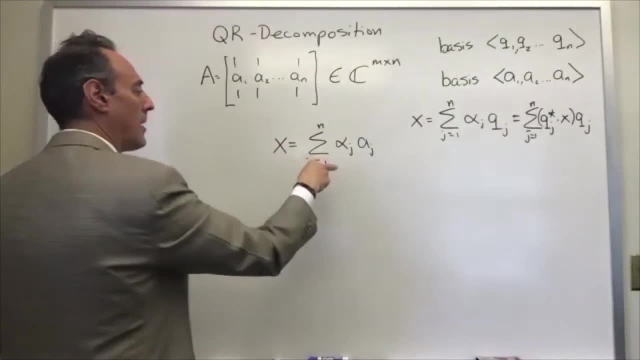 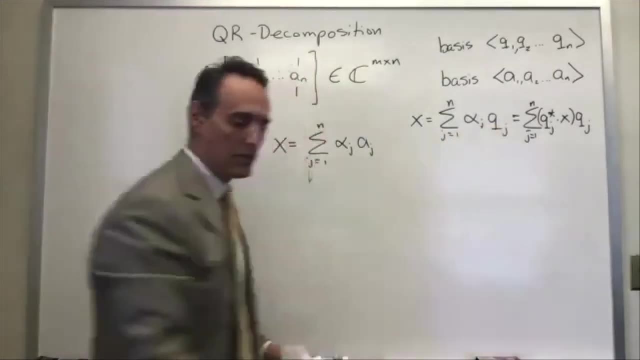 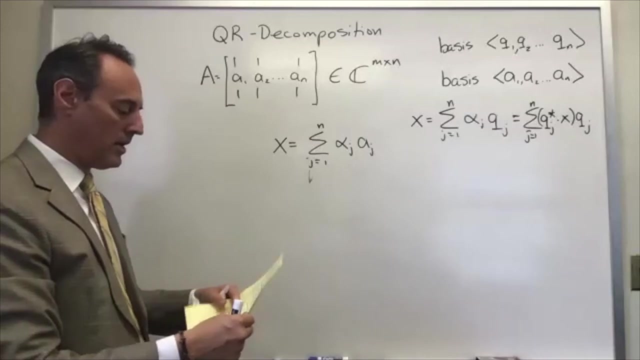 And what we showed here was exactly. you can either represent it in the original column space or an orthonormal coordinate space, And this is a much more attractive way to represent things. So let me go back to that original example. If you remember, is if I take 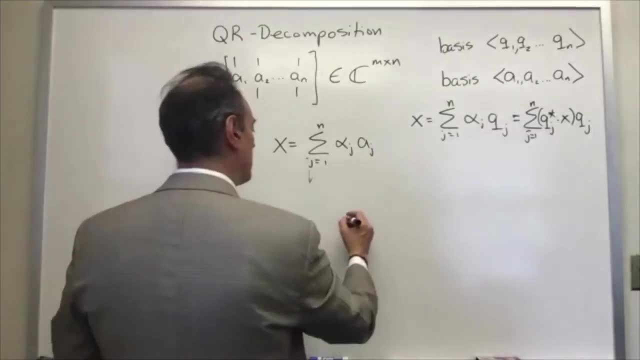 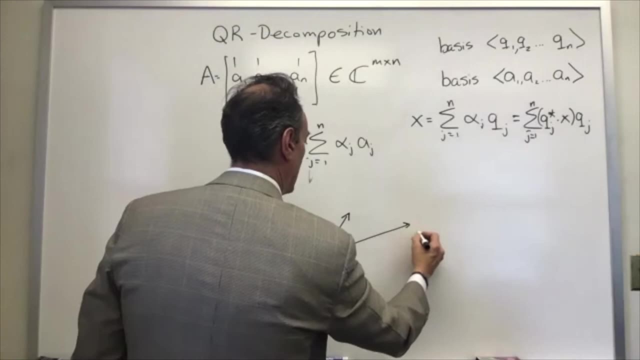 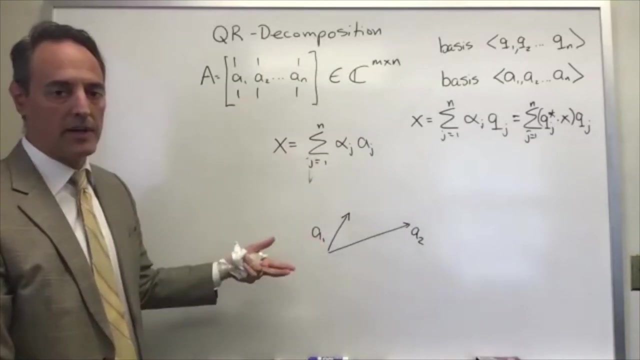 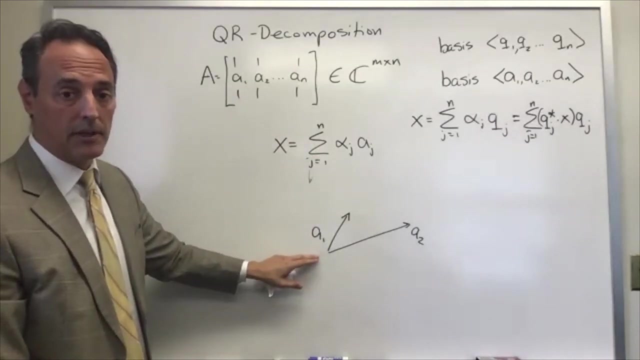 two vectors, a1 and a2. that's what i represented things with here. they're not even normalized, they're just whatever these vectors are, and i can just say, well, that's fine, this is a perfectly valid coordinate system as long as they're linearly independent. and these two vectors 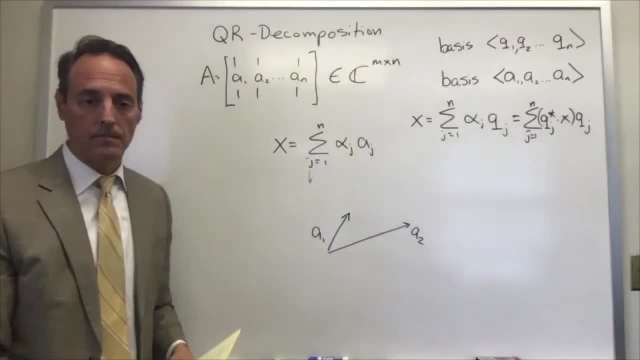 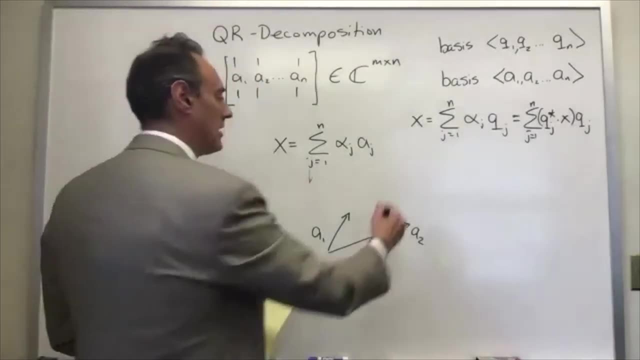 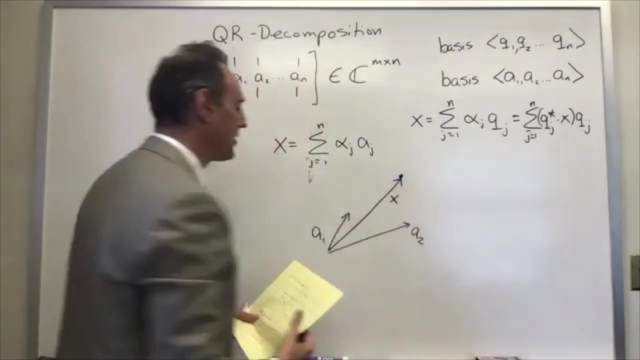 can span the entire r2 space. but now what i want to do is start thinking about: okay, but if i- and so let's take a vector i want to represent, let's say, x- is right here, so i can definitely represent this vector x in a1 and 2 using this kind of formulation. 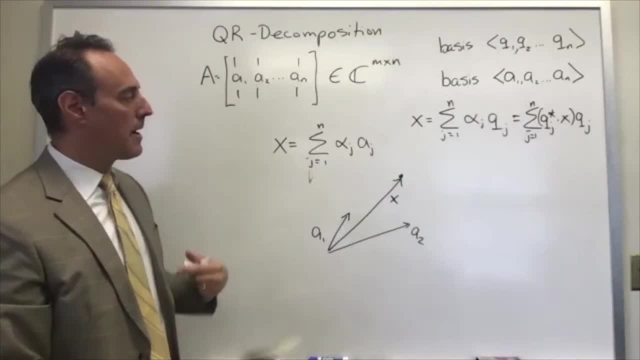 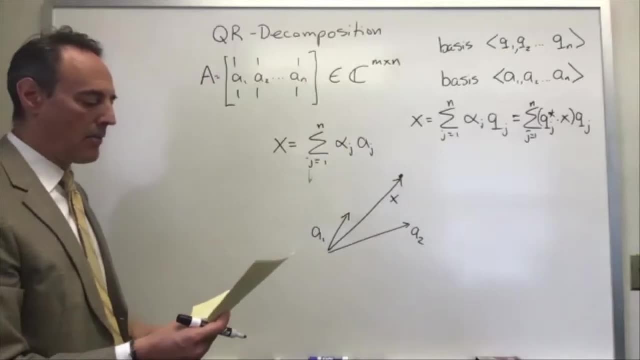 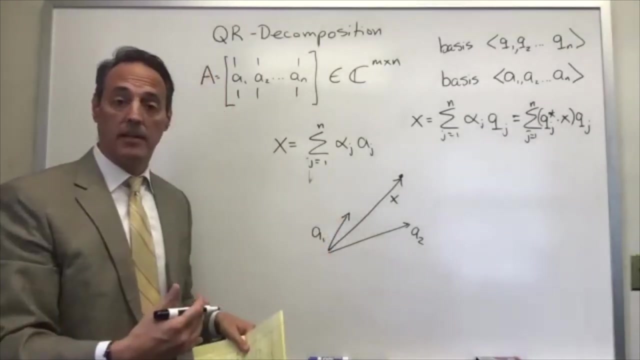 i could also think about building an orthogonal coordinate system with this. and how would i do it? well, let's, let's think about how we might do this. so the first thing i might do is say, well, let's pick a1 and just say that a1 is one of my, is one of my unit vectors, okay. so in other words, 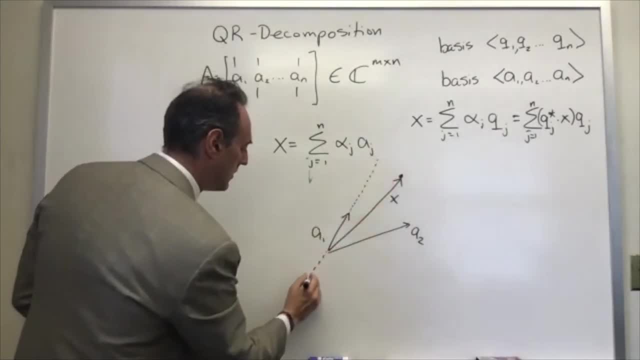 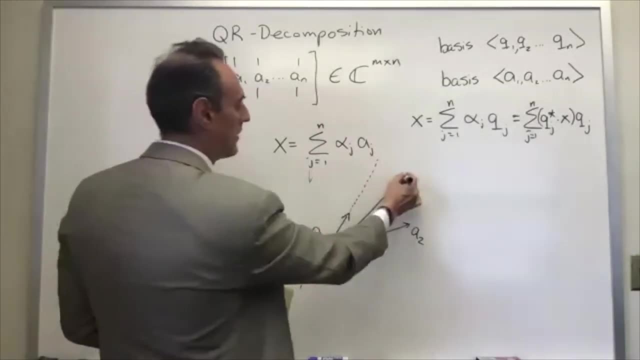 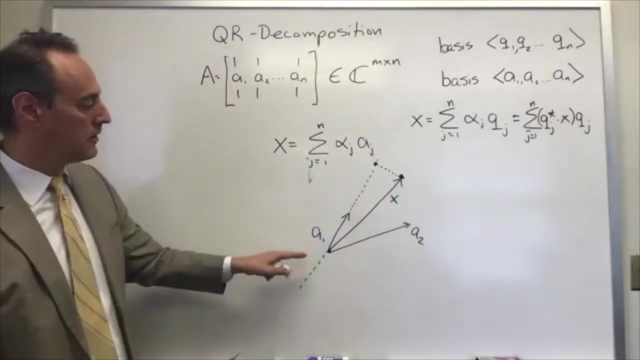 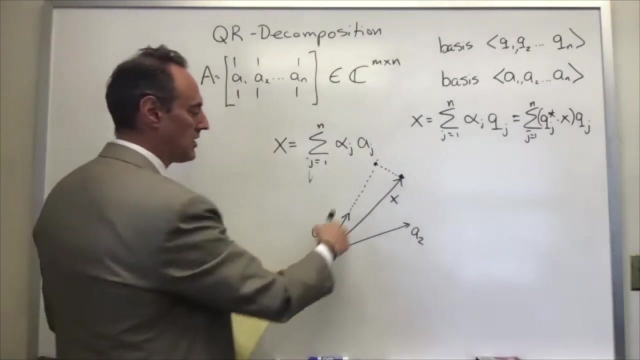 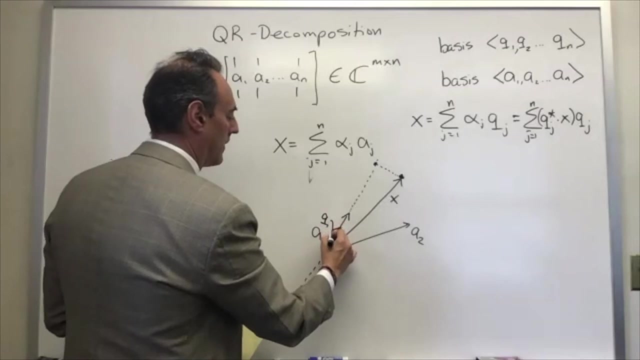 this direction here represents the a1 direction. so right away this point here has a projection along the a1 direction. so in other words i could make a unit vector- let's call it q1- along that direction. so let's say this has some length. let's say q1 is actually of unit length, that's q1 there. 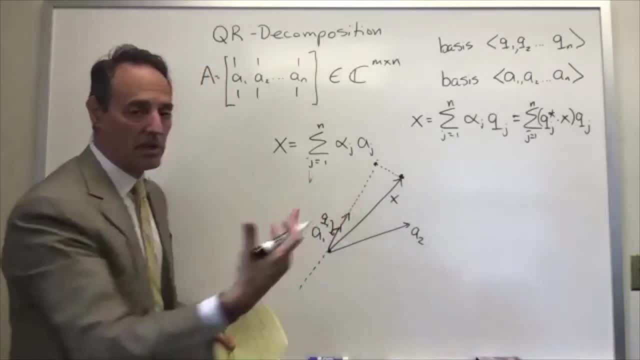 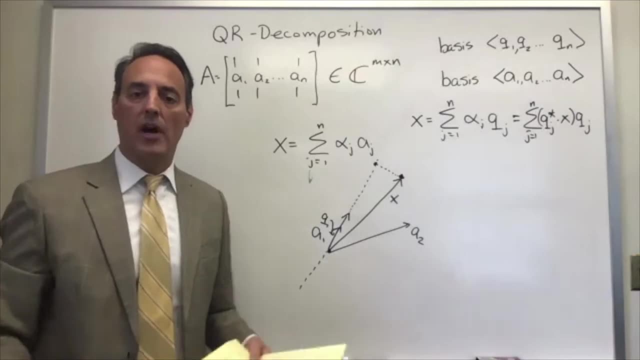 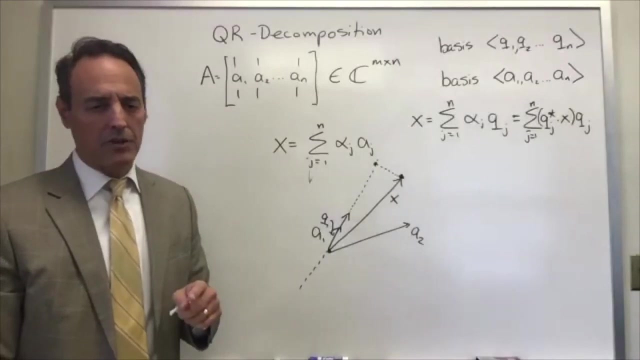 so that's length one, whereas a1 can be longer. now what i would like to do is say, well, i've got q1, but now how do i get an orthogonal direction to this? well, what i can start with is say: well, i have this a2 direction, and the a2 direction is kind of interesting because part of a2 is along. 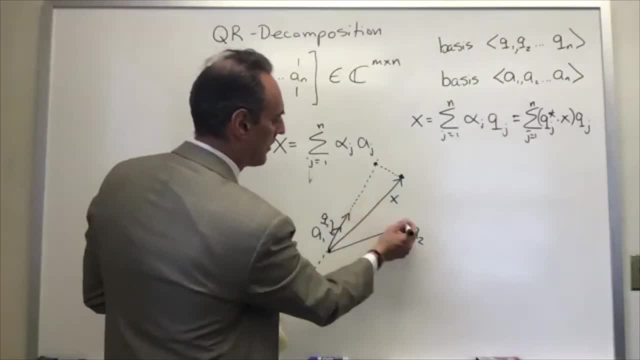 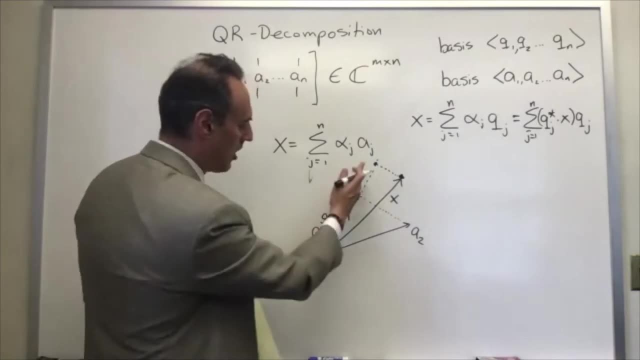 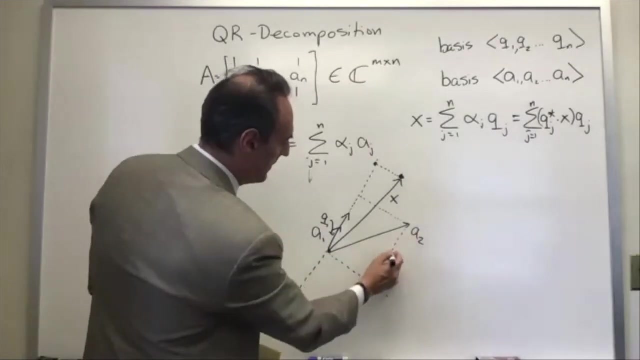 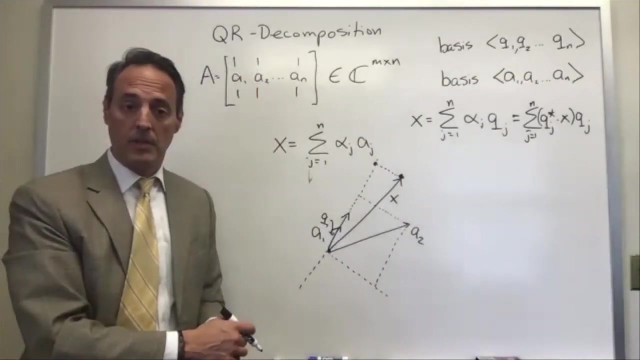 a1 right, which part? well, this right here. if i do a projection or a dot product between a1 and a2, this much of the vector a2 lies along the a1 direction. however, this much of a2 lies along an orthogonal direction. so i could take this a2 vector and say: you know what i really am interested in. 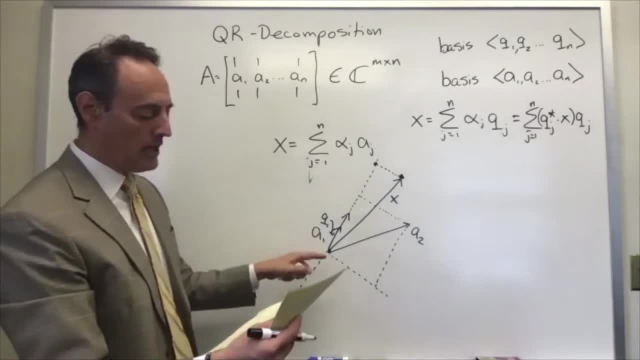 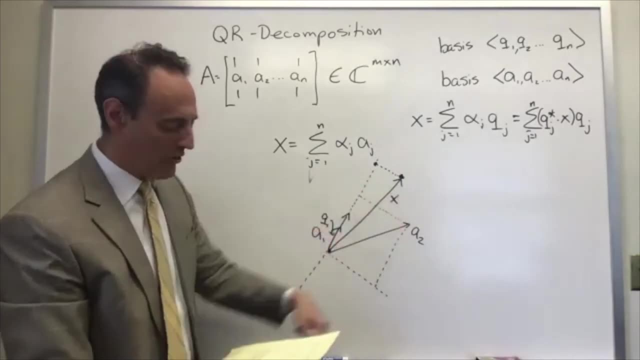 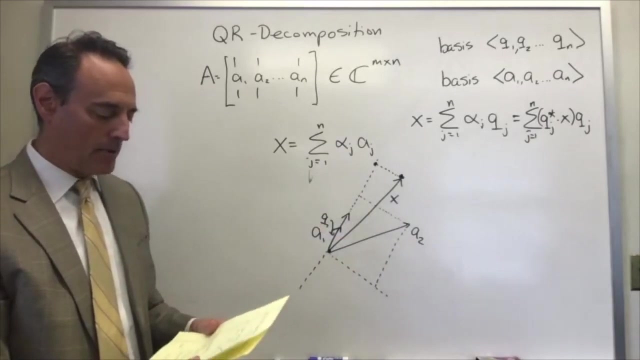 is. i'm i'm just really interested only in the projection of the vector a2 in the orthogonal direction to the a1, and so part of what we want to get at is: how do i represent that and i can start talking about what direction this is here. 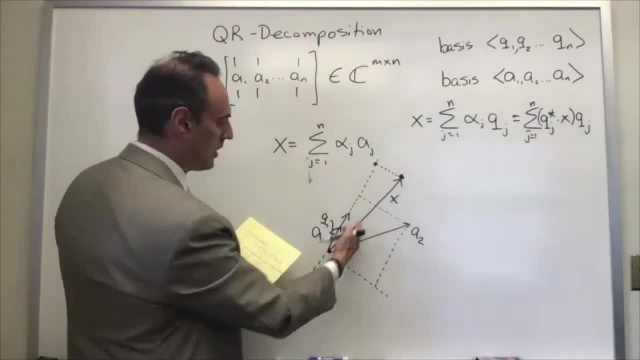 right, uh, so on the a1 direction. so i can project x onto this direction over here. and if i project x into the a1 direction, this is going to be x dotted with q1. is going to be this length, okay, so x dotted with q1. so in fact, i want to take 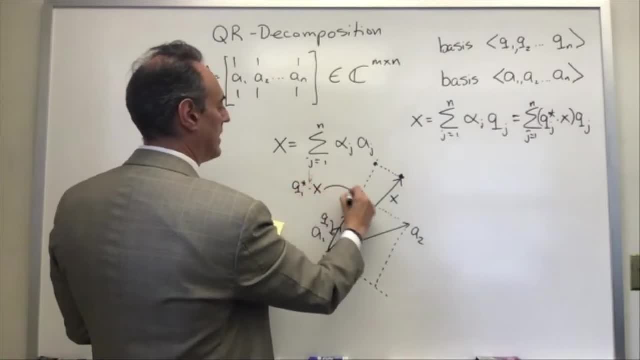 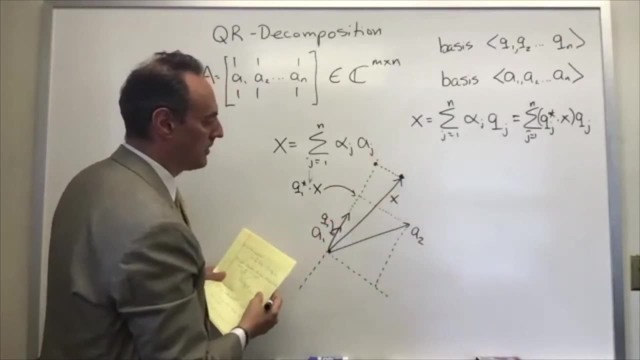 q1 star dotted with x, and this is this projection right here. that's, in other words, the length of the vector i want to get to, and this is the length of the vector i want to get to, and this is the length of the vector i want in this direction. and then let's talk about what this direction. 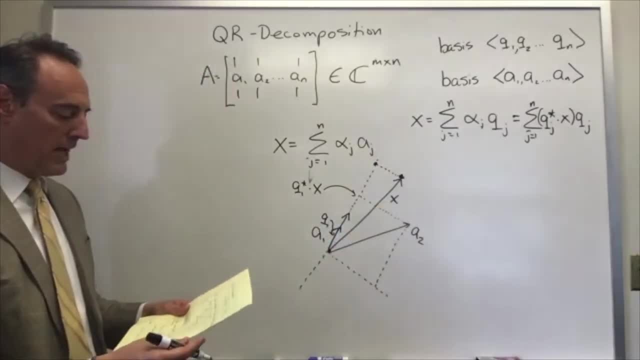 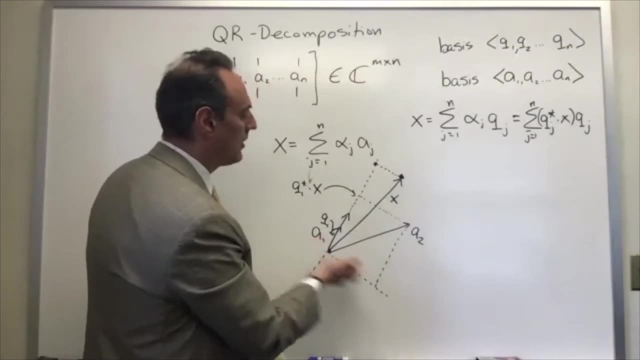 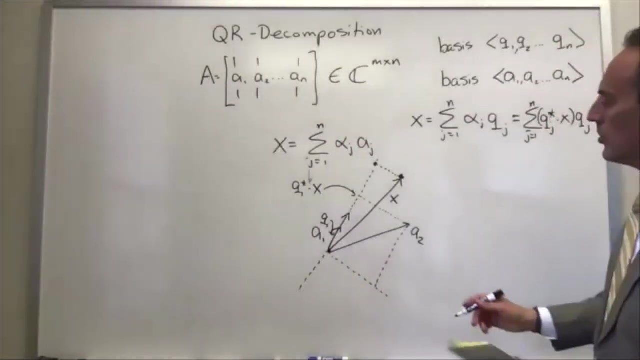 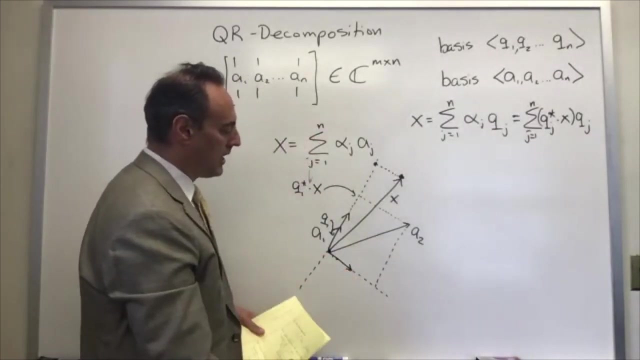 orthogonal to it is. so that's the next piece we have to build out. what we have to say is that i want the component of a2, only the component of a2 that's orthogonal to this component. so how would we build a vector q2? and so i want q2 to be unit length that direction. so what i'm going to do is i'm going to start thinking about. 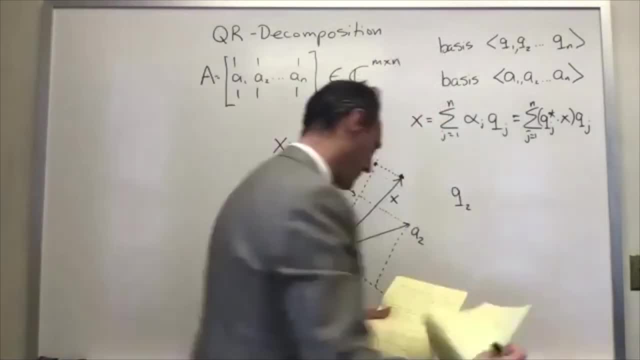 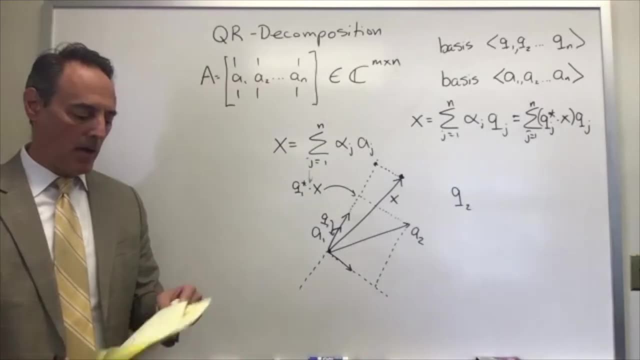 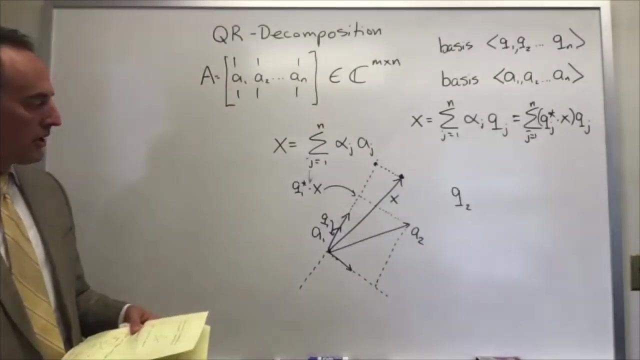 building q2 in the following way. i want to first of all say i'm going to pick a2 as the vector i'm going to start with and what i want to do with that vector a2 is i want to project out the direction. so part of a2 is along q1, part of it's along this q2. 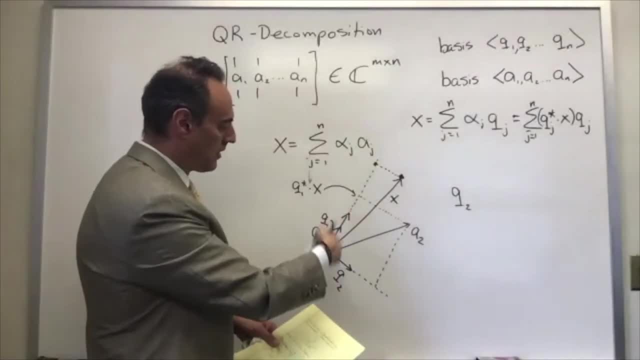 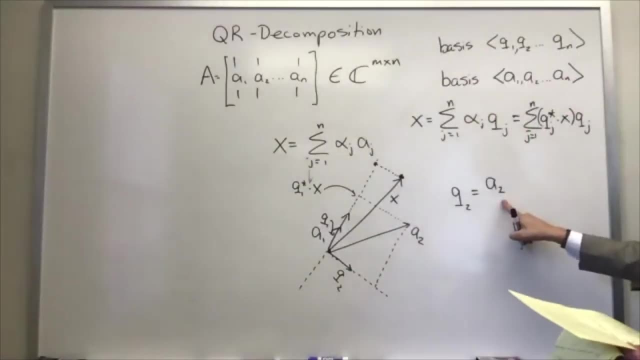 so what's the portion of the vector along a1 and along a2? so what i want to do is say, take q2 and b, take the a2 vector, and what i want to do with this is subtract the portion of this vector along that q1 direction, which is the following: 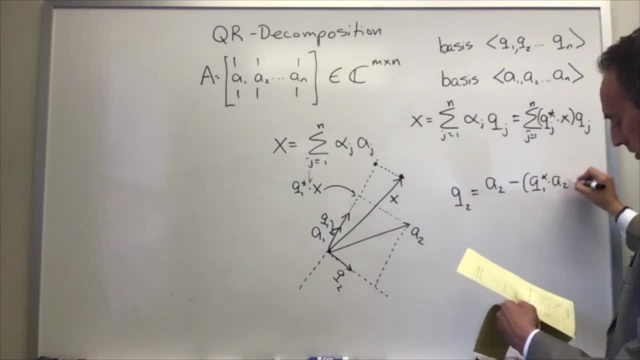 q1 star dot. a2, q1. okay, so a2 vector. so what? this is right there. q1 star, q2- this is the length of this component along the q1 direction and i'm going to subtract that vector off from the a2 vector total, so in: 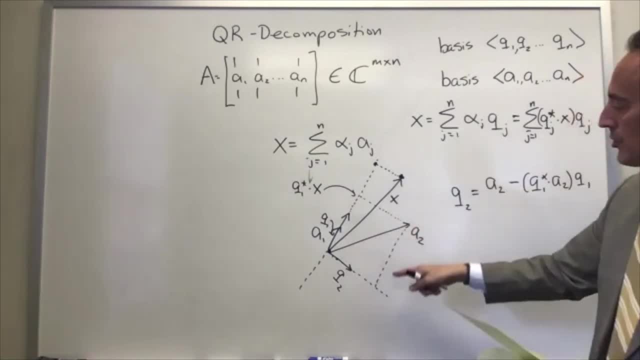 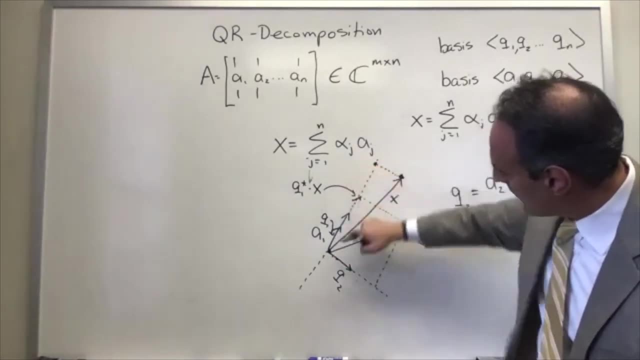 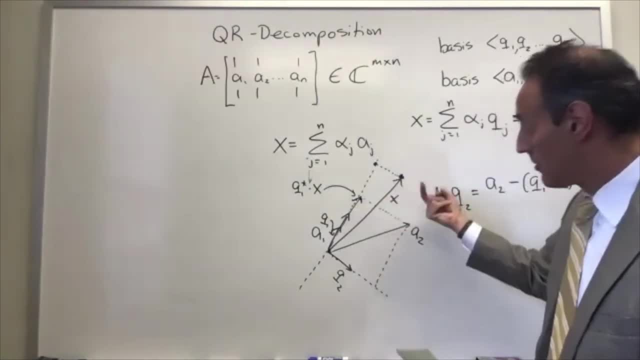 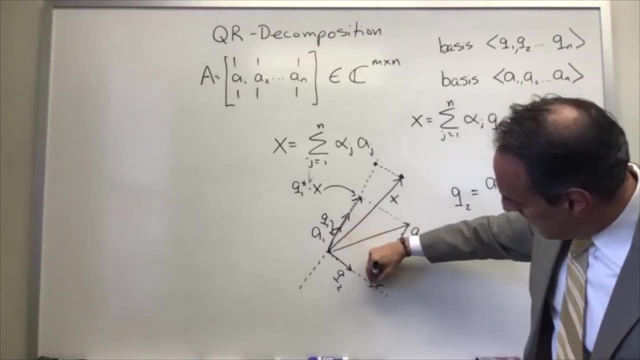 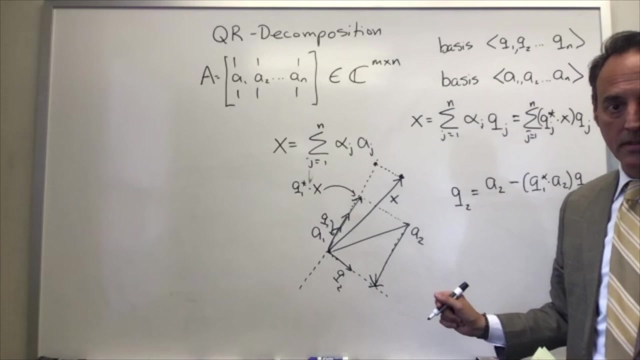 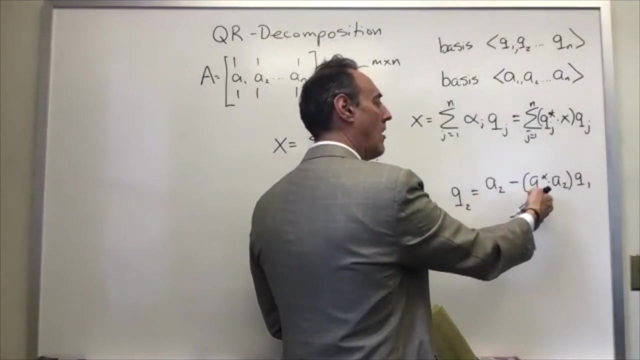 subtract that from it. so this vector subtracting that. now take the minus of it, it's this vector, right there. so this vector minus this vector is that vector. okay, so that's how you would think about this. so what i've done is i've created a new vector, starting from a2 and subtracting it out of. 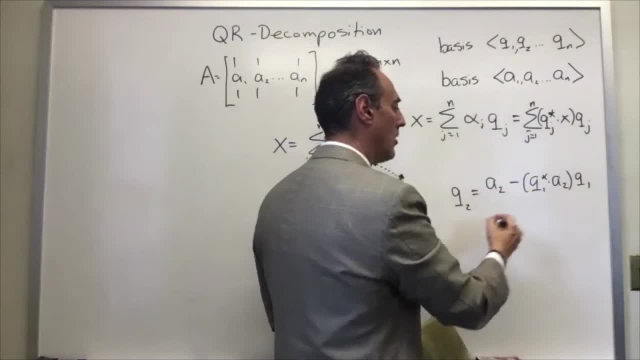 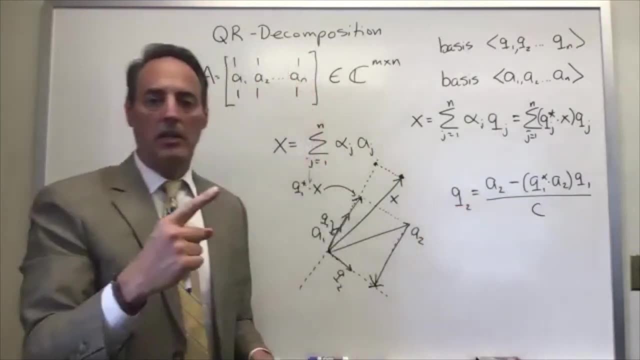 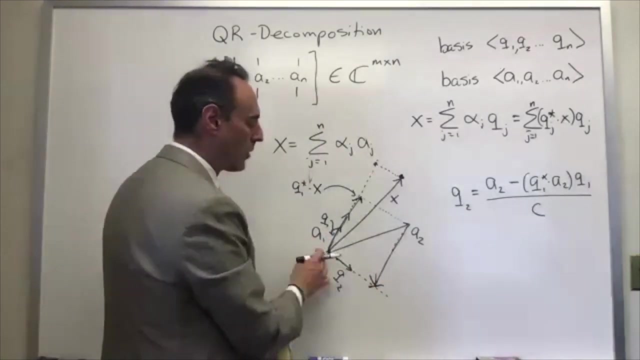 the a1 direction so that i make sure it's orthogonal. and then i'm going to divide by some constant c, which is a normalization, so i can make q2 be length one. so hopefully you can convince yourself of exactly what i did here, which is i need the orthogonal direction to this. 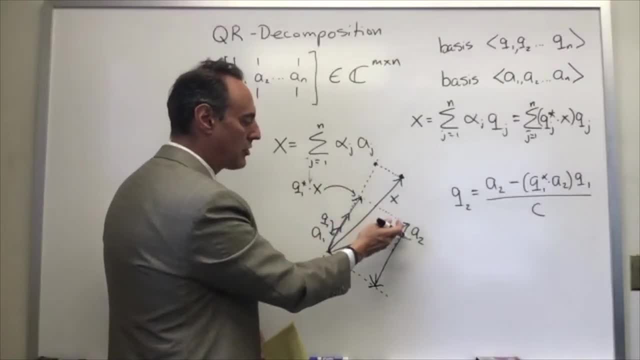 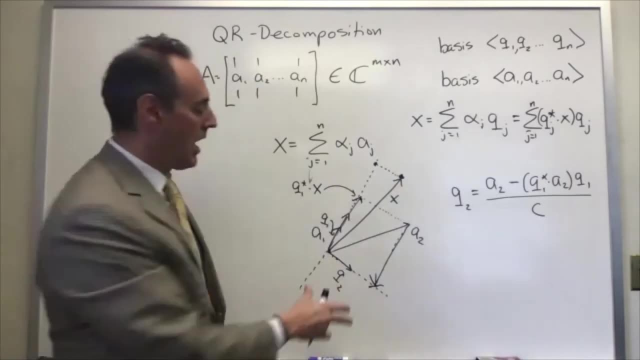 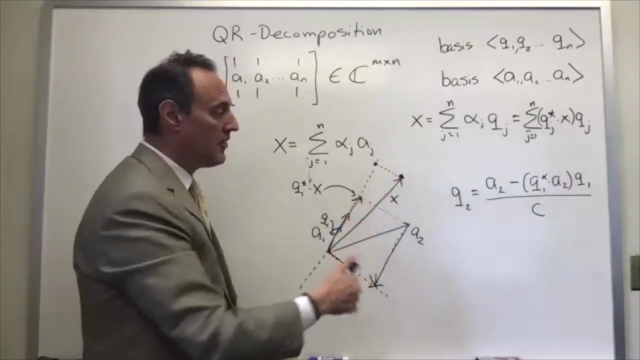 a2 is not orthogonal, but i can take a2 and subtract out the component along a1, and that gets me now on orthogonal direction. now on orthogonal direction, and whatever i get here, i have to now normalize it to make it length one, and that's the idea. this is the idea behind graham-schmidt. 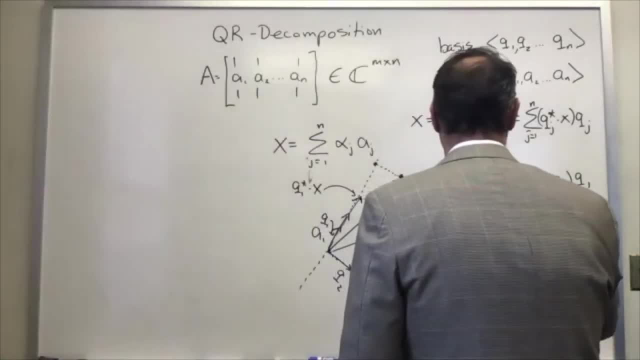 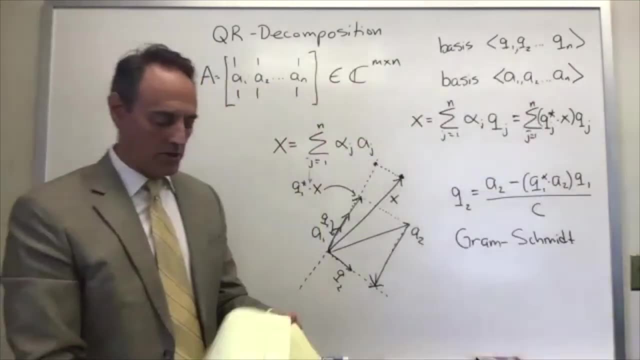 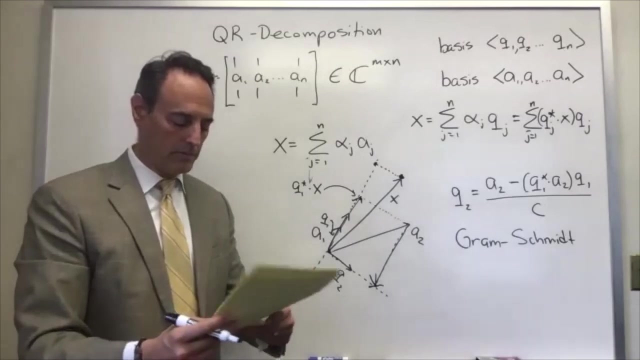 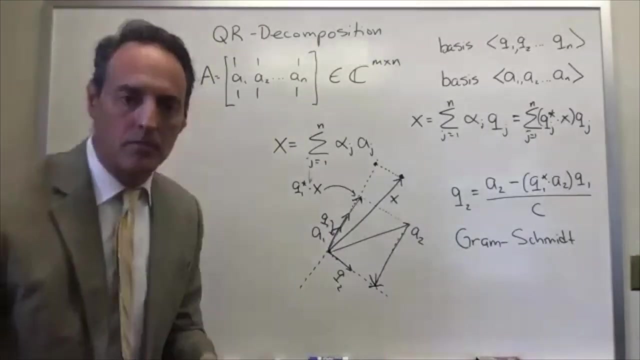 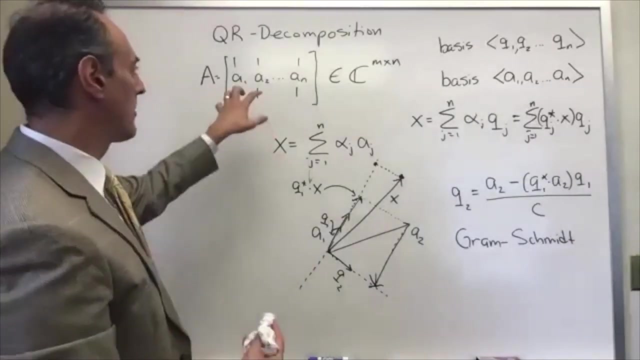 or orthogonalization. so it's one of the standard linear algebra tricks that we use out there for doing orthogonalization. okay, all right, so this is where we're going to go with this. this is a, but my hope is this is sort of the picture of how we're going to move from a coordinate system like 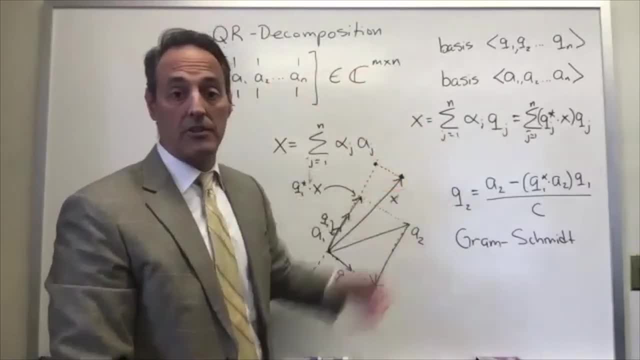 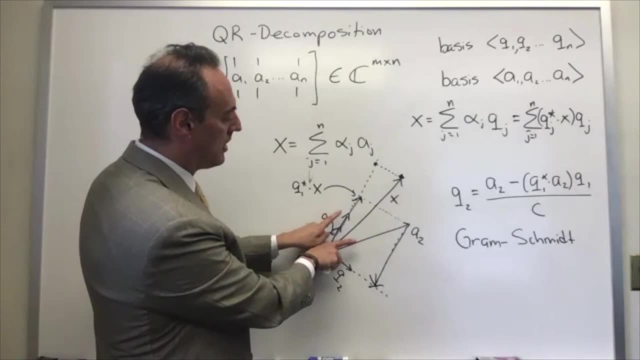 this to a coordinate system that, in fact, is orthogonal. okay, and that's the like. this is the picture. i start with a coordinate system that's not orthogonal. i pick one of the directions and i take the other vector which is not orthogonal, and i just say: take this vector and 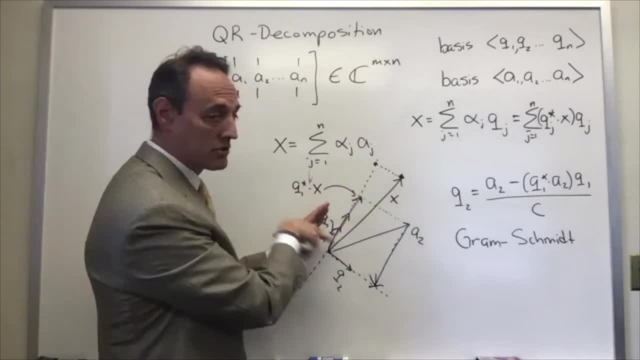 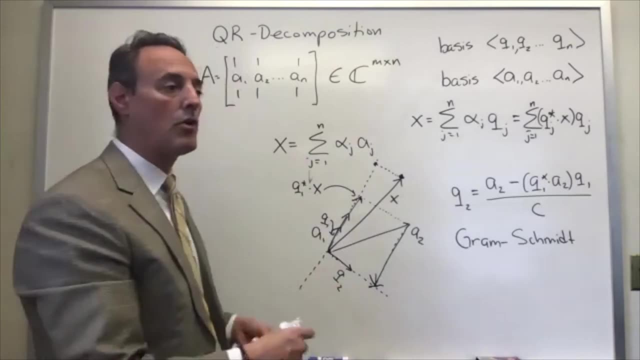 subtract out the component along this direction, so the only thing left is the component orthogonal to it. you make that a basis vector, and if you go to n dimensional spaces, you do this recursively. now you say: okay, now you've got two orthogonal vectors, make a third that's orthogonal to those two and 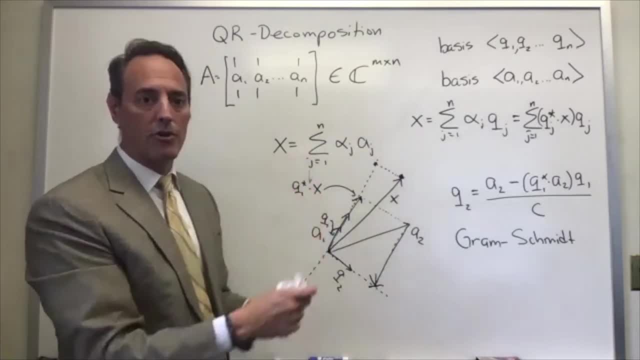 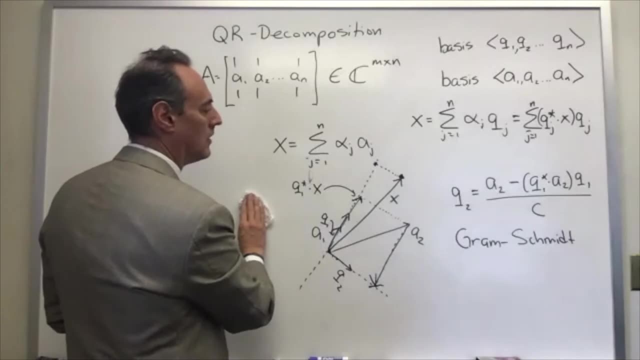 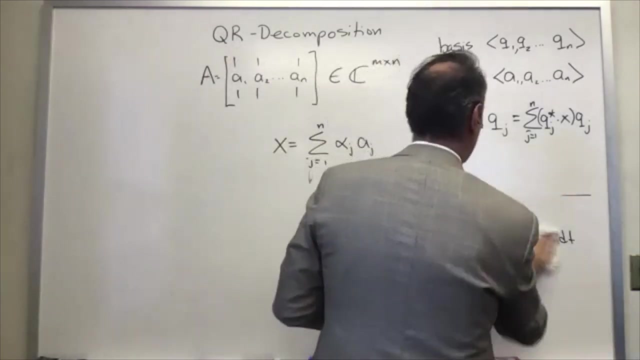 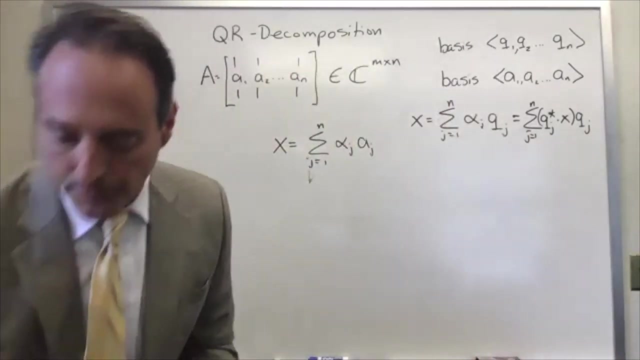 then make a fourth that's orthogonal to those three and so forth, and you start building it out until you span this n-dimensional space. okay, we'll come back to that in a moment. all right, so let's talk about what q factorization then is. qr factorization is: 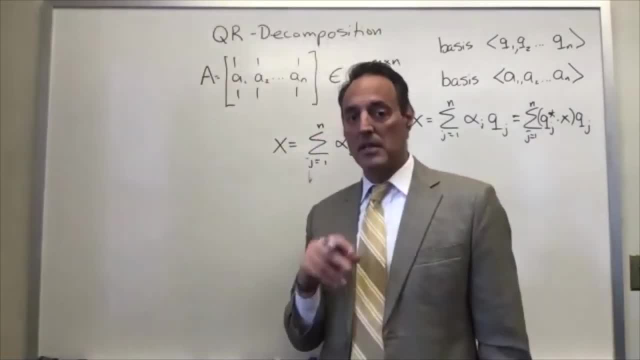 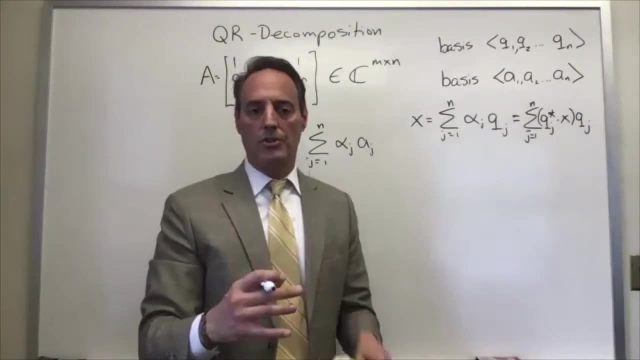 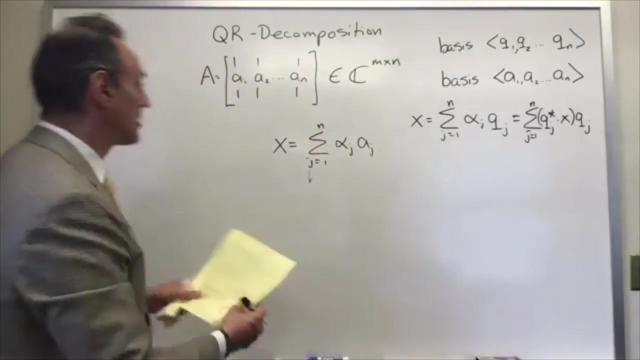 so qr factorization, then you're starting to see, hopefully- is nothing more than some formal approach to graham-schmidt orthogonalization. so what i want to do with this is consider some data matrix a, which is m by n, with m bigger than n or equal to n. 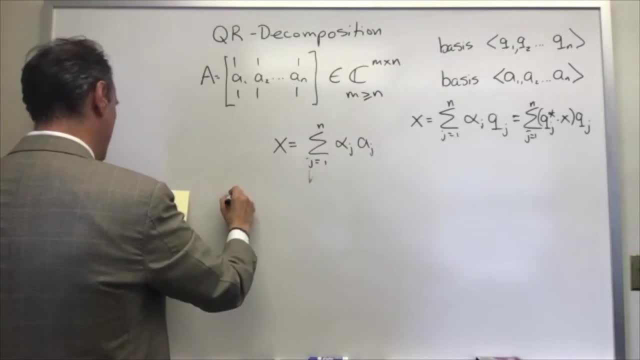 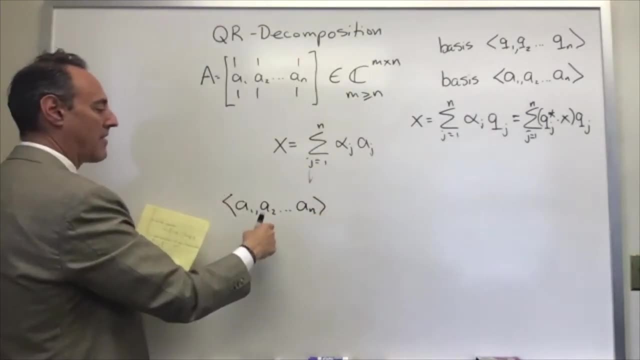 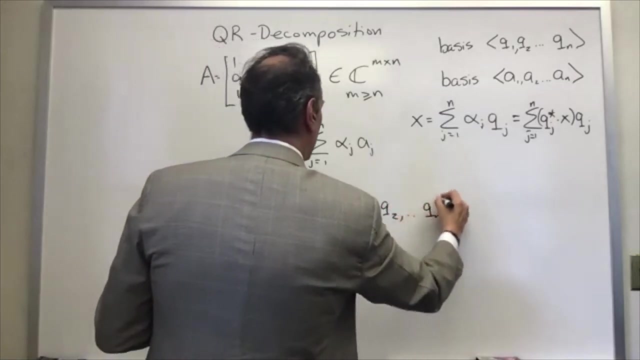 and what i really want to think about is taking this basis set and i think about the span of this basis set and i want that span of that basis set to be equal to the span of that matrix set, to be equal to the span of that basis set. 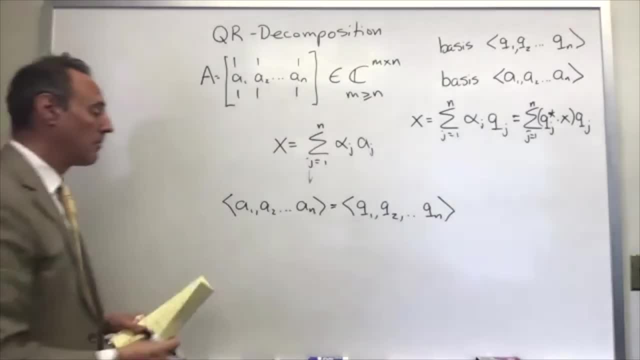 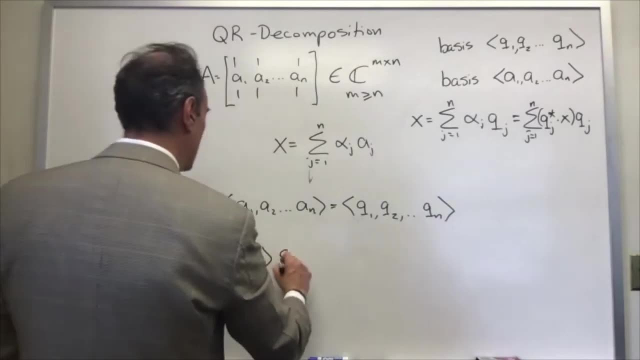 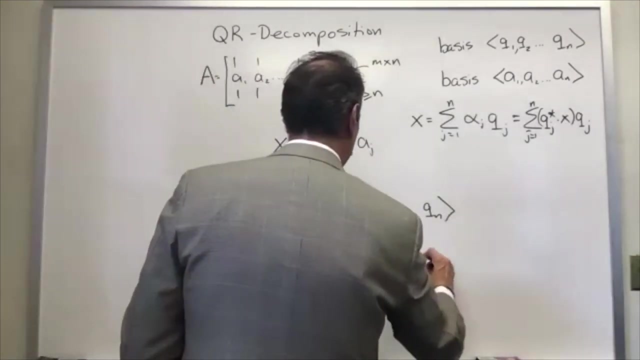 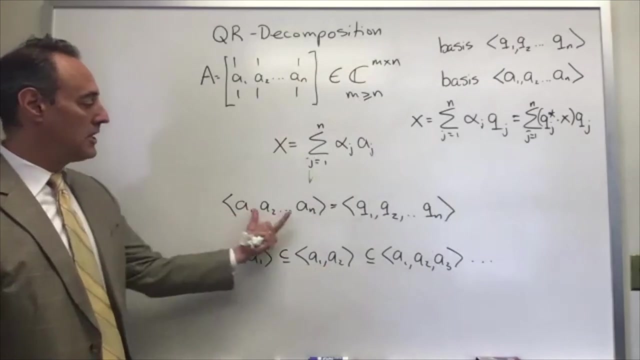 okay. something to notice- by the way i'll write this out- is that one way to also think about this is: a1, which is one of the vectors, is contained within the subspace of a1, a2, which is contained in the subspace of a1, a2, a3 and so forth. so remember that these are linearly independent. 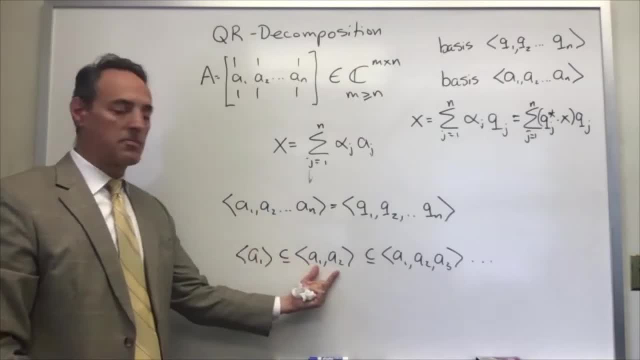 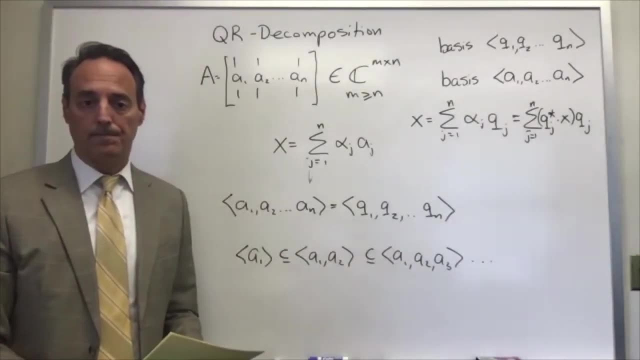 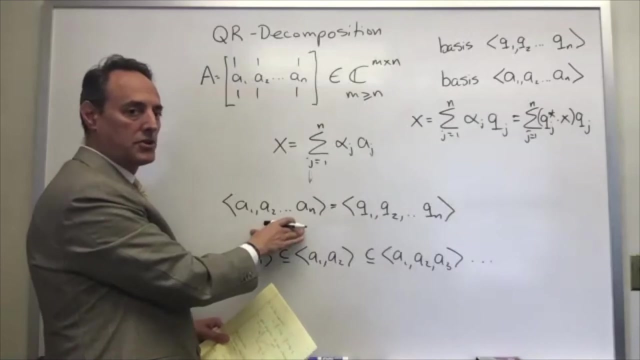 vectors, which means every time i add a direction, the span gets bigger and bigger and bigger until i contain the entire n-dimensional subspace. okay, so this is the idea. i want this equivalency. i want to move from this coordinate system which spans this n-dimensional space. 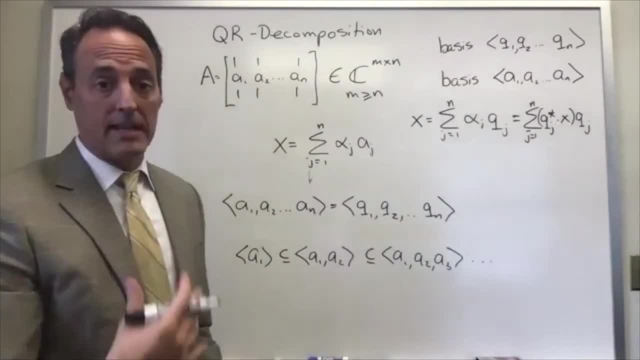 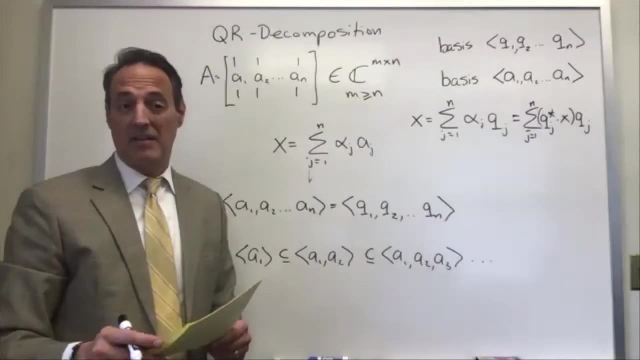 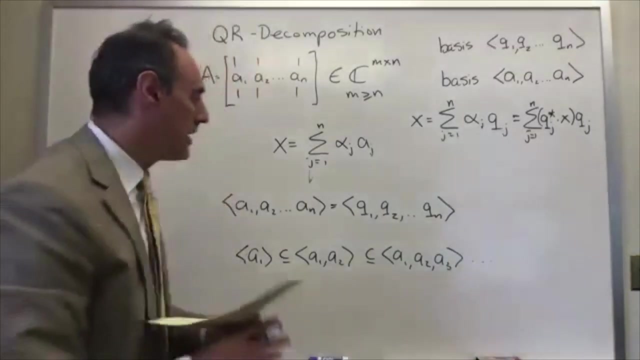 to this coordinate system which also spans that same space, but i have all the advantages of orthogonality available to me, because I actually have a great coordinate system with orthonormal vectors. So the way to do this, so that's the concept of the subs, of spanning spaces. 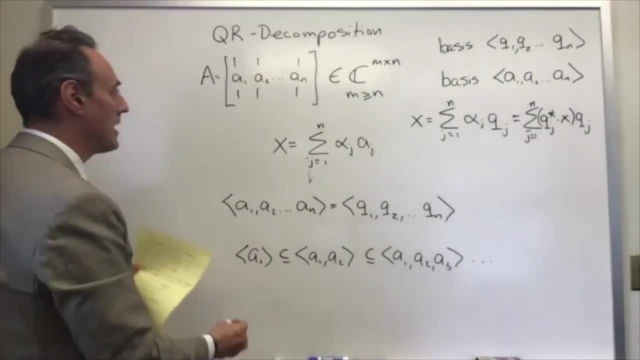 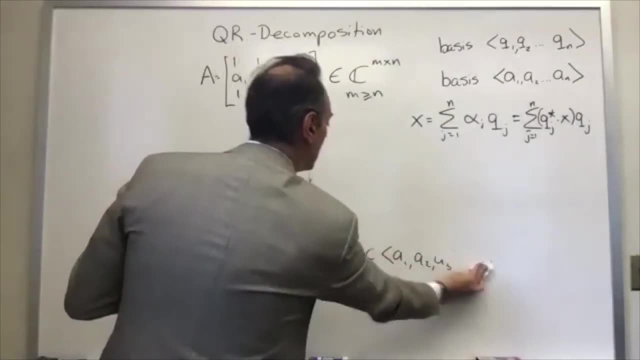 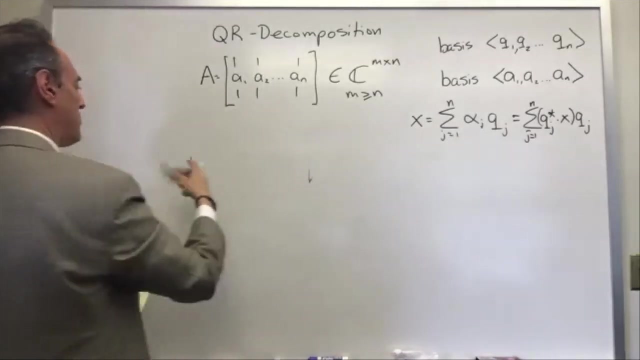 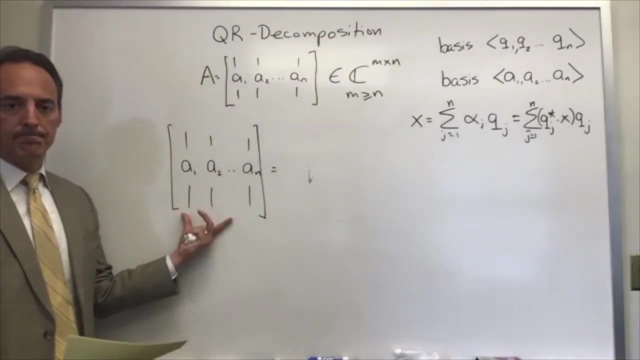 and the way that the QR does this is: let's draw it and write it out, and then you'll see how this all works out. Okay, so here's my matrix A. It has n columns, and my goal now is to make a linear transformation. 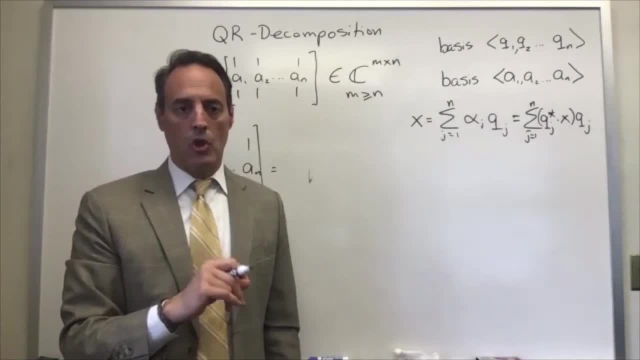 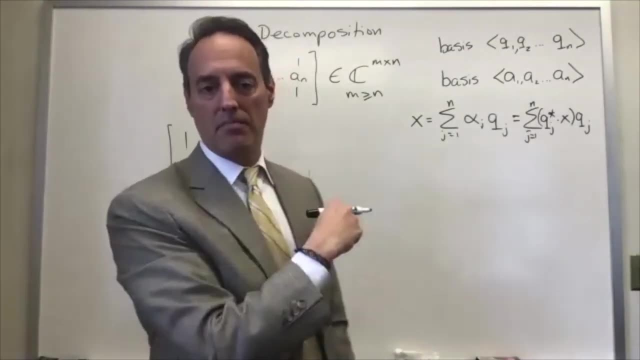 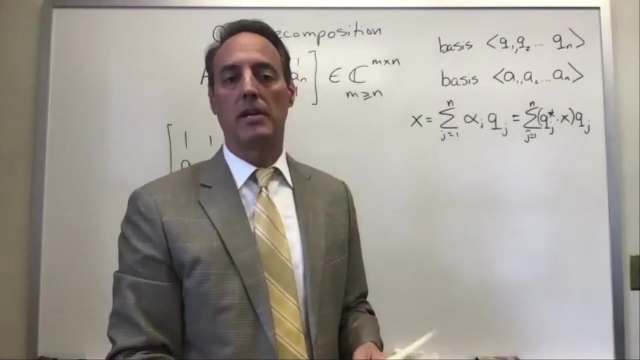 A linear transformation to a new coordinate system. When I say a linear transformation, that means I'm going to try to find a matrix to multiply this by to get me or to make a sorry. I'm going to try to find a matrix that makes this transformation happen. 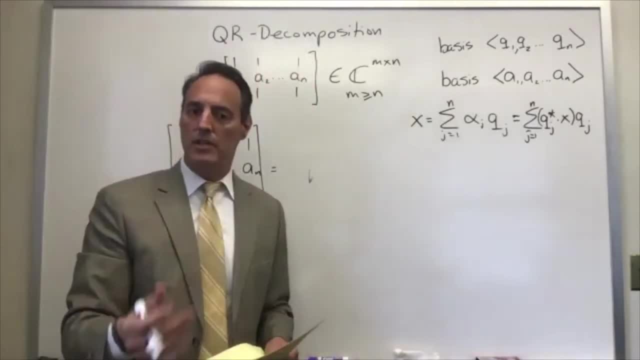 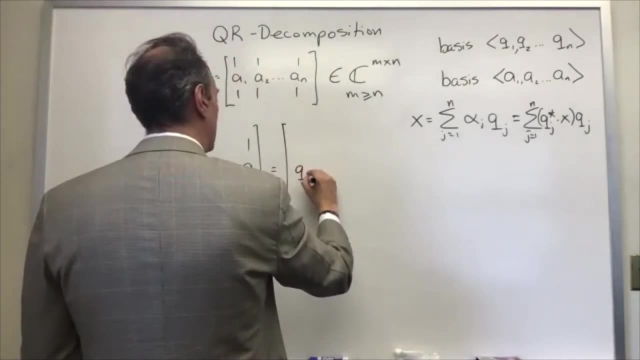 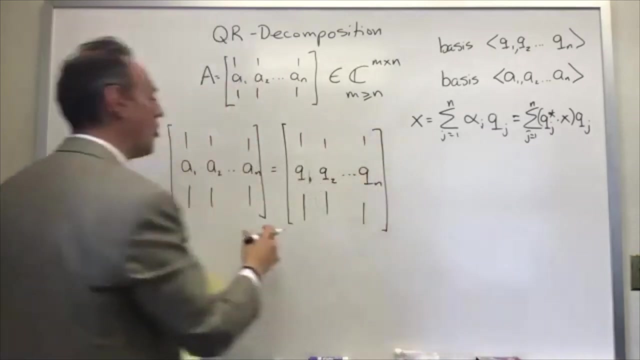 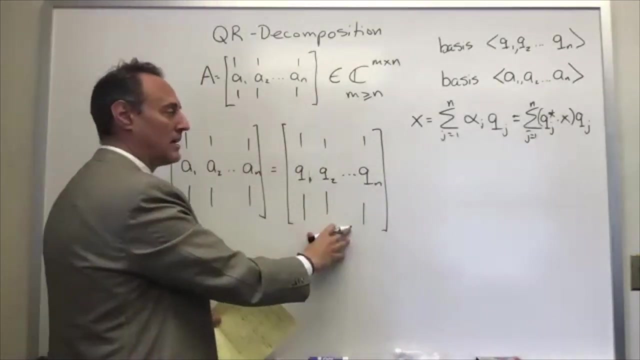 Okay, that's so. matrices are linear transformations, And what's the linear transformation I'm looking for? I'm looking for this one. What I want to do is go from this set of n-dimensional vectors to this n-dimensional orthonormal basis set. 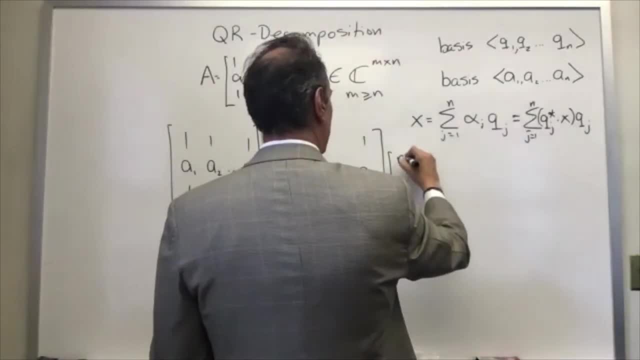 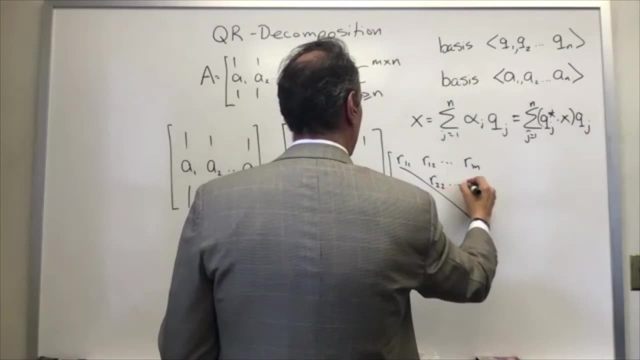 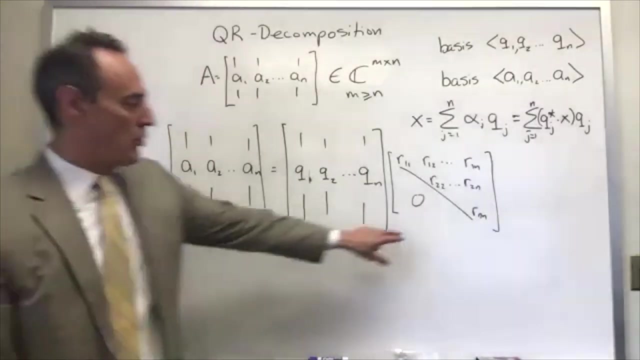 and the way I'm going to do it is through this matrix right here, An upper triangular matrix Of this form, So the matrix R. one way to think about it, it's a linear transformation. That's what the matrix R is. 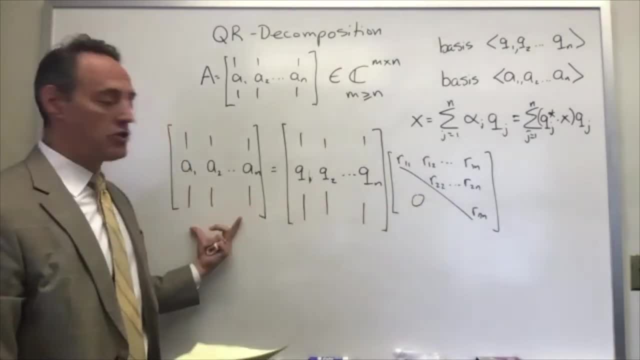 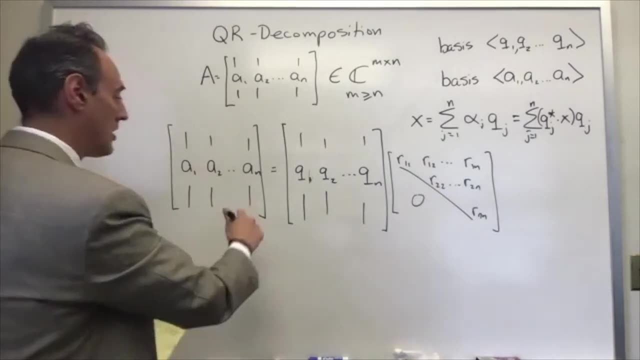 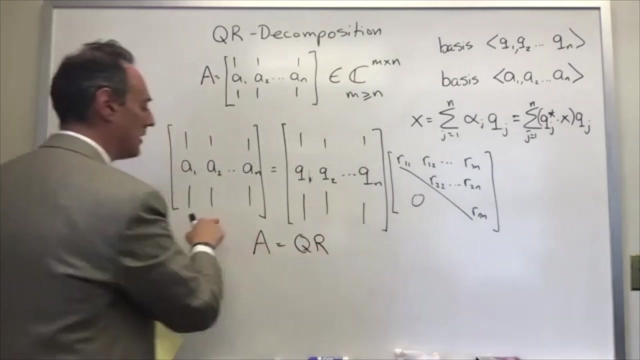 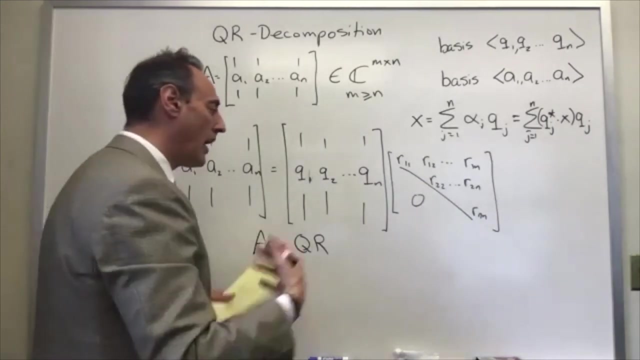 Linear transformation from an orthonormal basis to your column space or to your original data vectors: A. Okay, so this here is the. A is equal to QR. Unitary matrix- upper triangular. here's your data matrix. Okay, Or, if you want to draw it like what we did in the SVD: 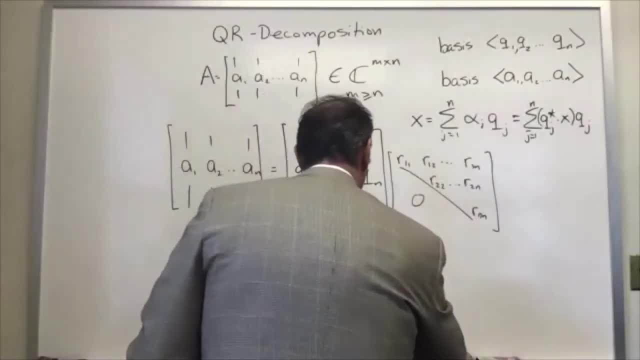 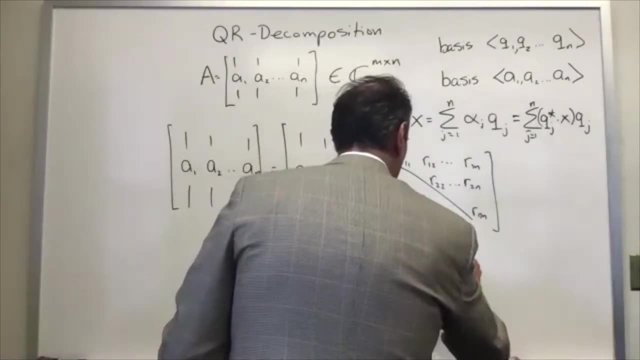 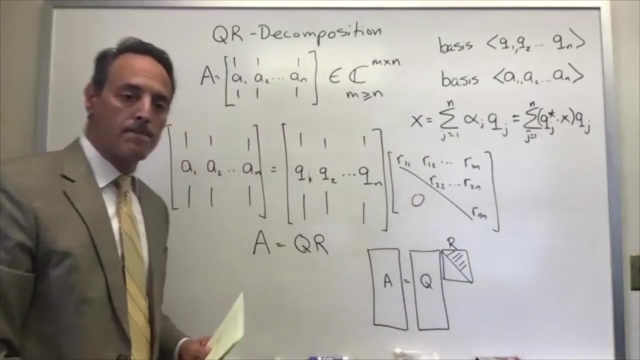 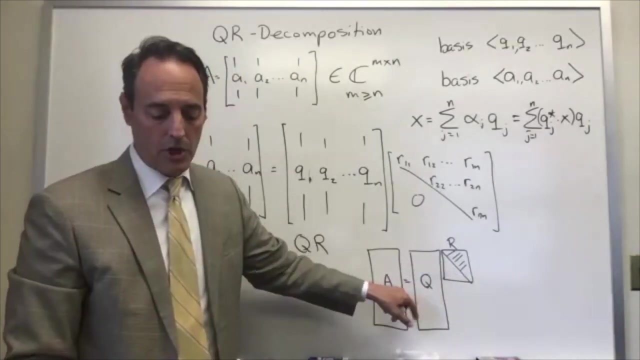 you can draw this in the following way: Here's your matrix A and the decomposition is creating for you some matrix Q times R. Okay, so that's the decomposition product of two matrices, where this has destruction. that's structure, that's orthonormal. 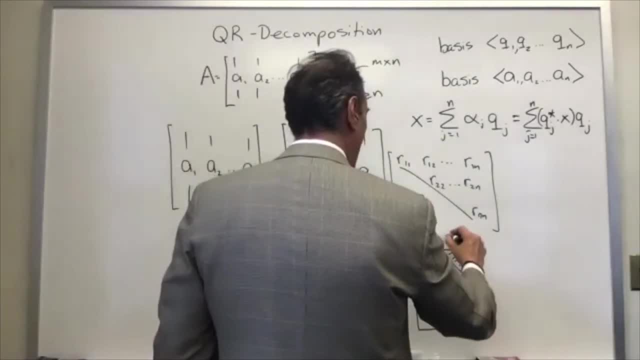 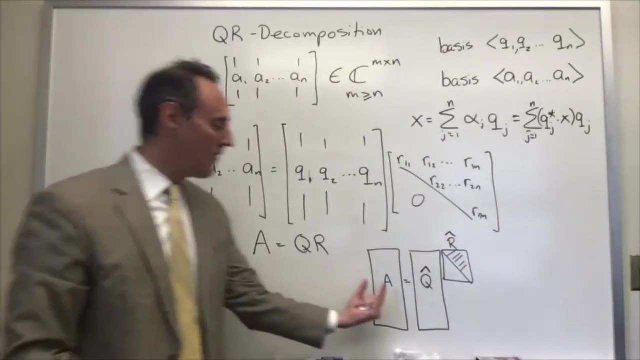 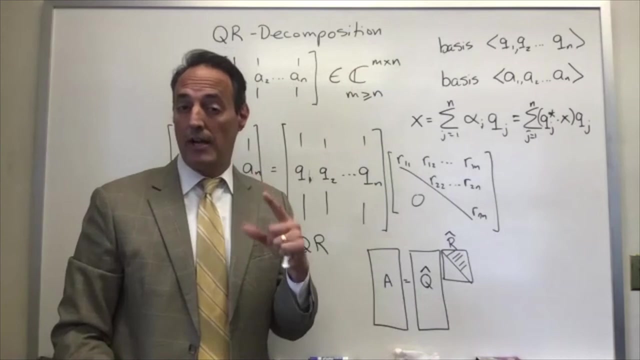 So I'm actually going to put this here in this picture, as Q hat R hat. This is often called the reduced QR decomposition. In other words, if I have n columns, this is n columns, The full QR decomposition, just like the full SVD. 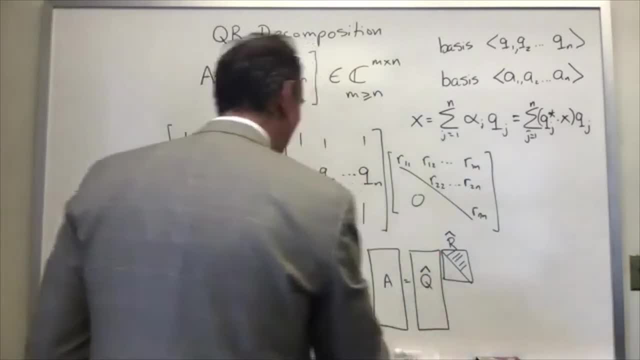 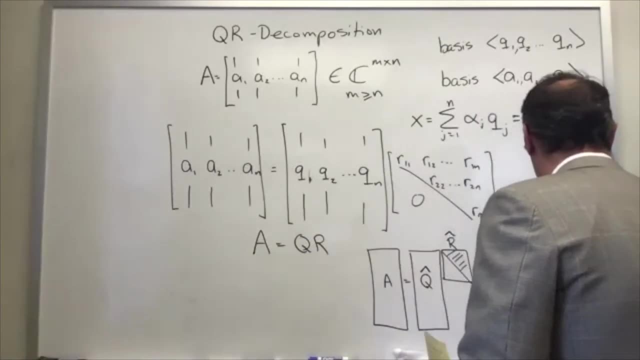 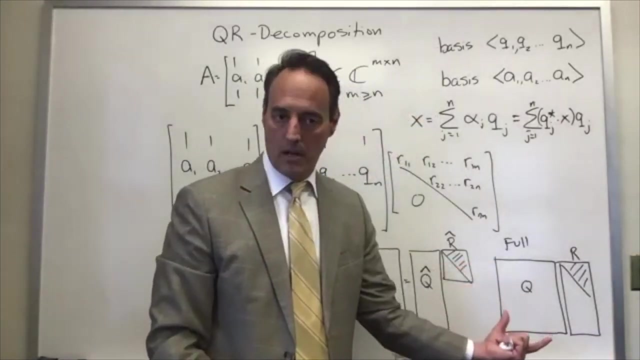 is, instead of going down to a matrix like this, the full SVD or sorry, the full QR is equal to Q R. In other words, instead of this thing having n columns, it now has m columns, And, in fact, a lot of these columns over here. 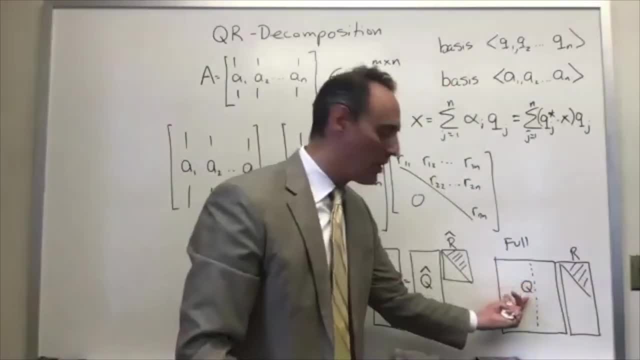 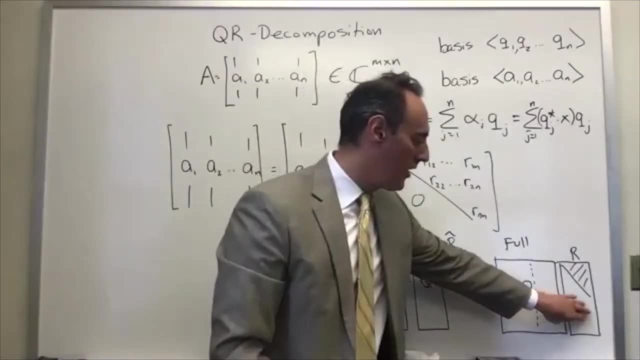 are often called the silent columns. They're orthogonal to these, but they're just added on to make it a square matrix. Okay, So they're silent because they're getting hit by zeros, So they don't play any role. This is the actual spanning subspace of your data. 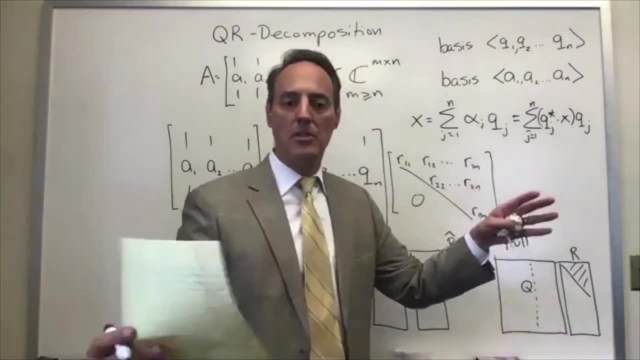 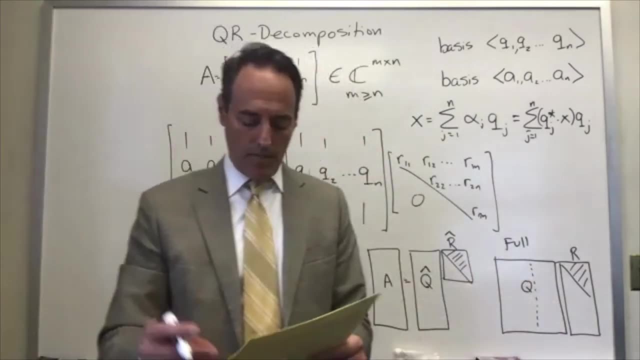 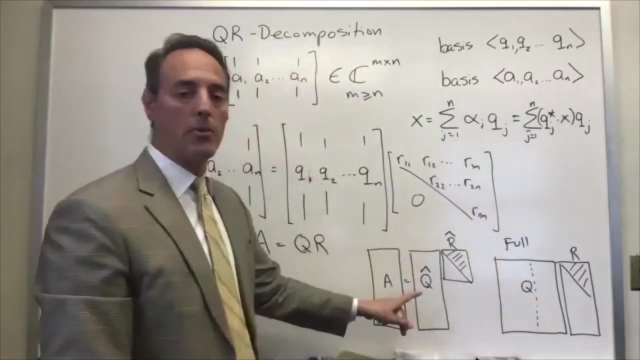 These are just being able to span an m-dimensional system, where these are spanning the n-dimensional system of your data. So, by the way, so I just want to make sure you understand: the formal QR is the full QR. This is the reduced QR. 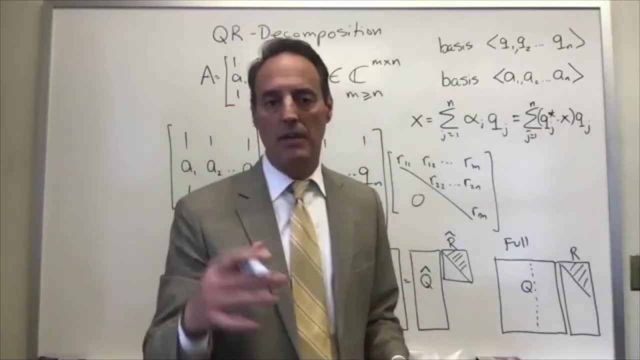 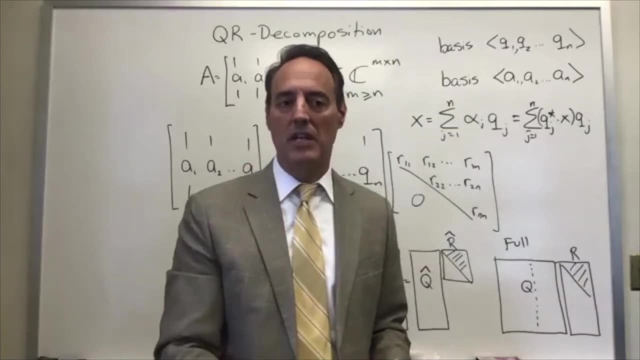 And oftentimes when we did the SVD- if you look at those lectures- what we really wanted was a low rank approximation, So we wanted some reduced SVD. We did not want the full SVD. Okay, So just keep that in mind in what we do this. 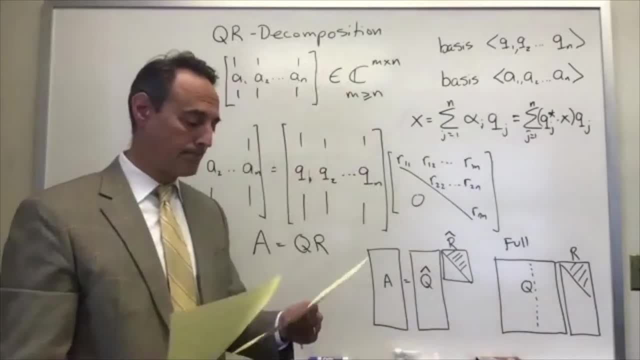 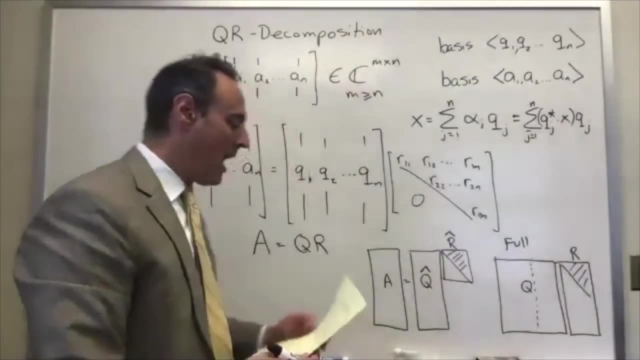 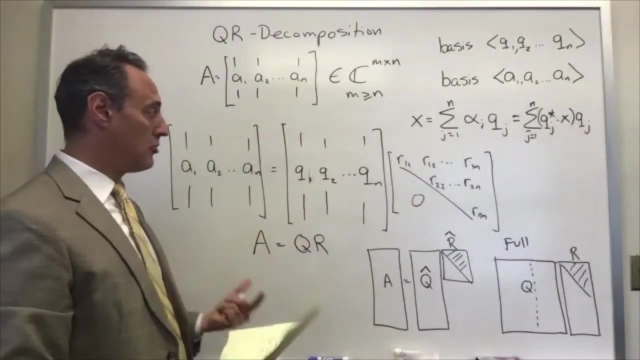 because it's going to play out. the same thing is going to play out here. Okay, How can we accomplish this? Basically, notice, I want to be able to do two things. Then, if I do this, I obviously have a. this is what I'm given. 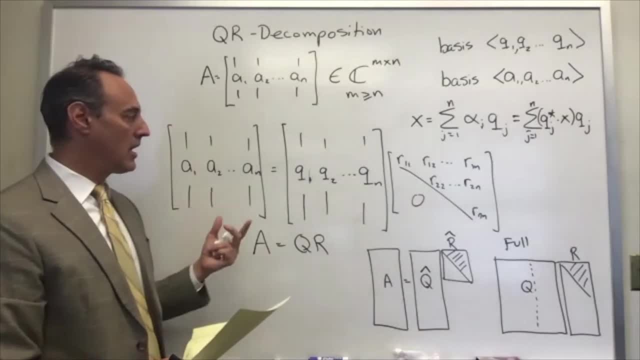 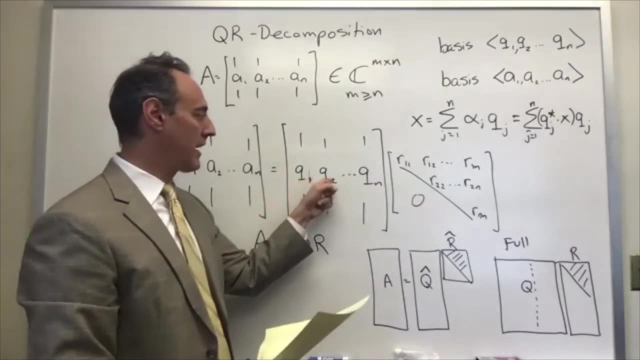 And when I look over here, there's a number of things I have to compute. I have to compute each of these vectors. I have to make them orthogonal to each other, I have to make them unit length, And then I've got to compute how I add them together. 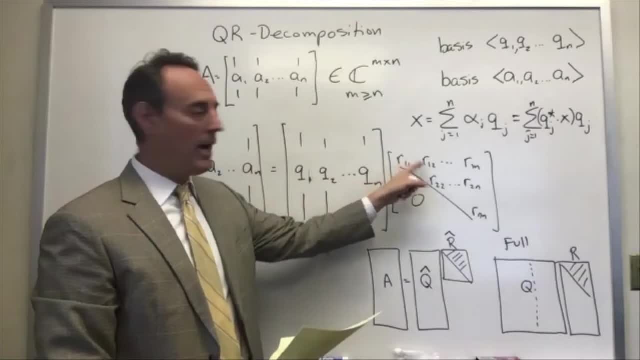 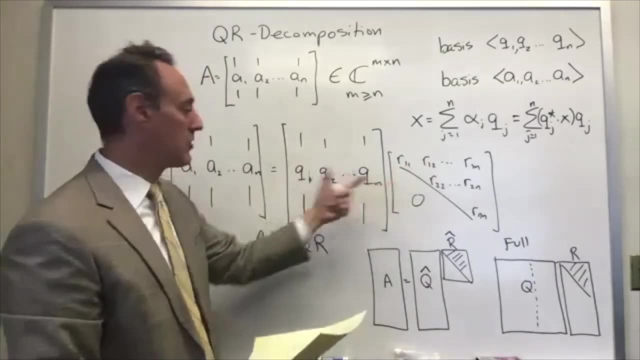 And then I've got to compute how I add them together. Okay, And then I've got to compute how I add them together here. to make this Notice: I have to compute this linear transformation and these and these vectors as well. So the question is: 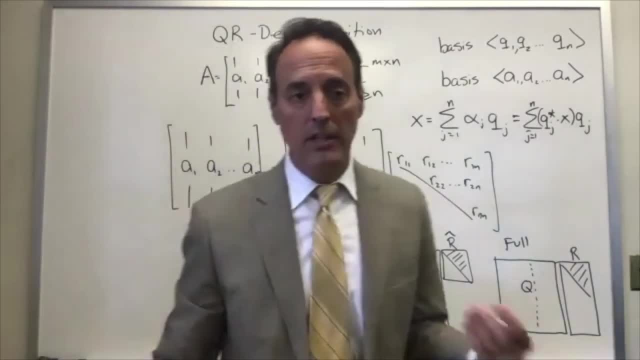 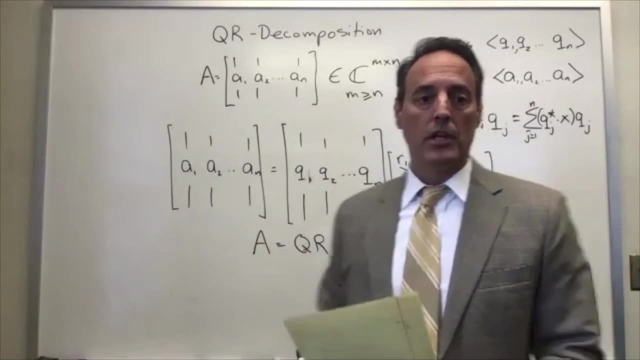 how are we going to do that? And this is where we're going to directly use the Gram-Schmidt orthogonalization procedure to produce exactly this. Because, if you remember, in Gram-Schmidt, Gram-Schmidt says: takes any N dimensional spanning set. 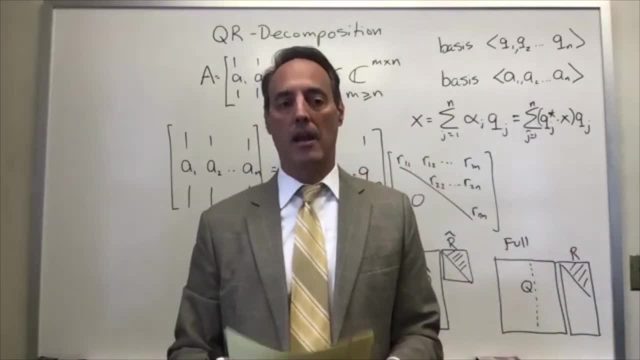 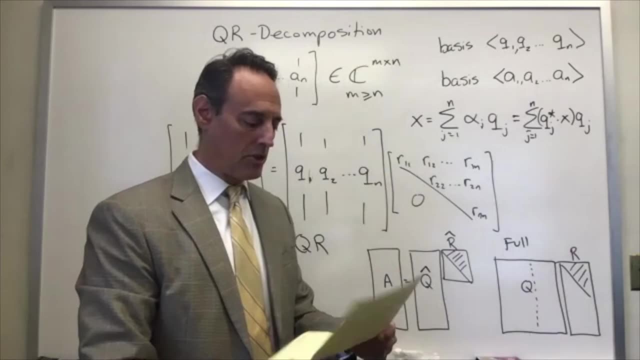 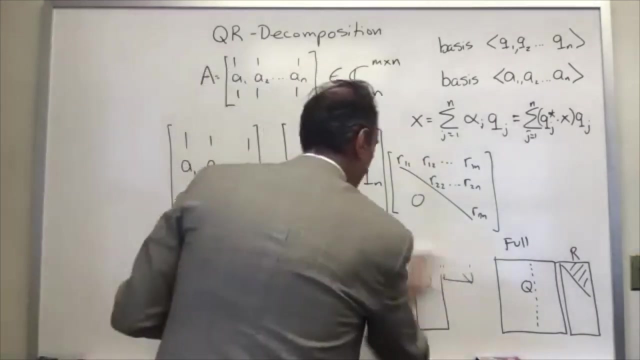 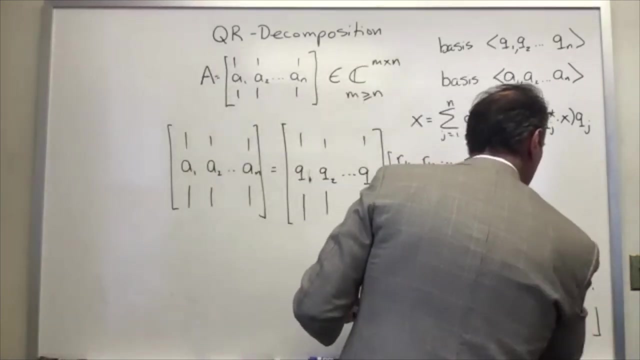 and then makes an orthonormal set for you out of them. Okay, That's exactly what I'm doing here now. Okay, And so we're going to figure out what is the algorithm to do such a thing. All right, So let's talk about that algorithm. 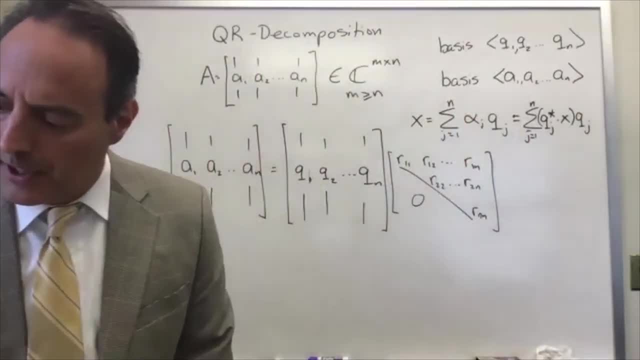 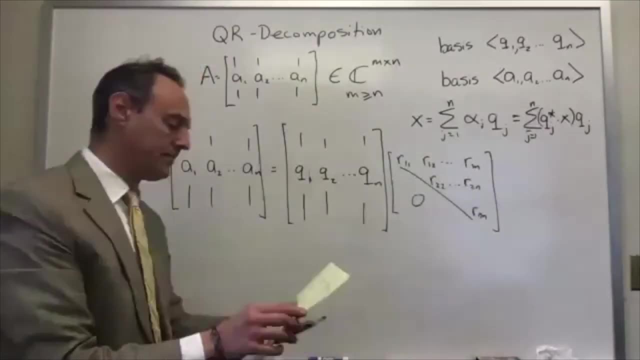 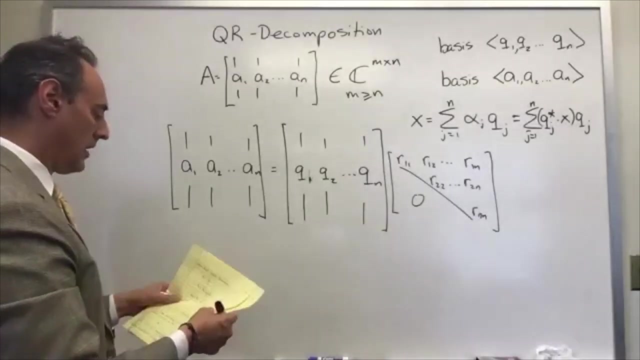 And also I do want to highlight here. I think: let me see, did I write any of this out? Nope, Okay, All right, So let's, let's figure out how to, how to write this out. So, first of all, 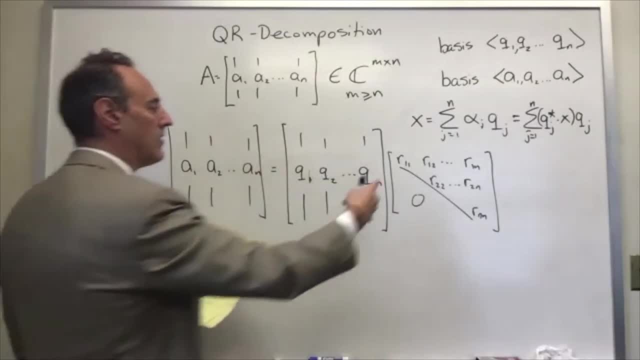 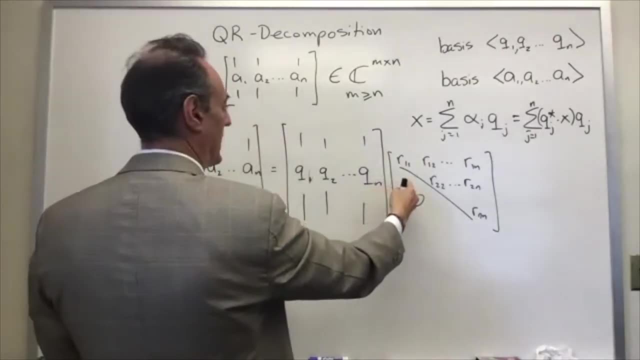 let's look at the sets of equations I have here. right, I have this. multiplied by this is equal to this, right, And there's a lot of zeros here, which is great, Okay. But if you do this out, what you're going to find is the following: 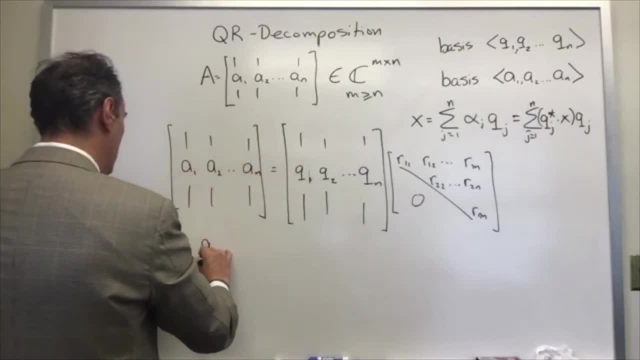 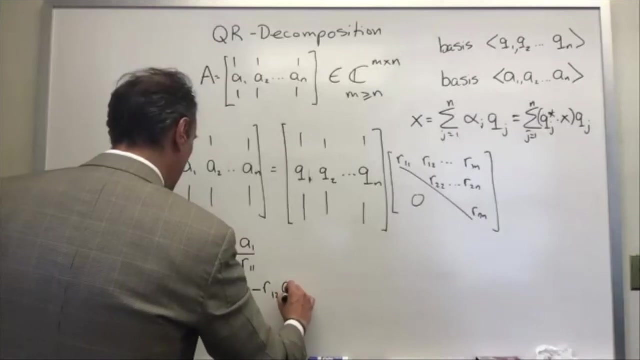 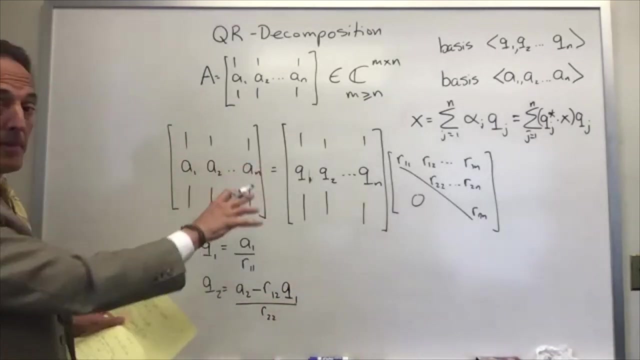 The first equation that comes out of this is that Q1 is equal to A1 over R11.. You're going to find that Q2 is equal to A2 minus R12, Q1 all over R22.. So this is just by doing the math here. 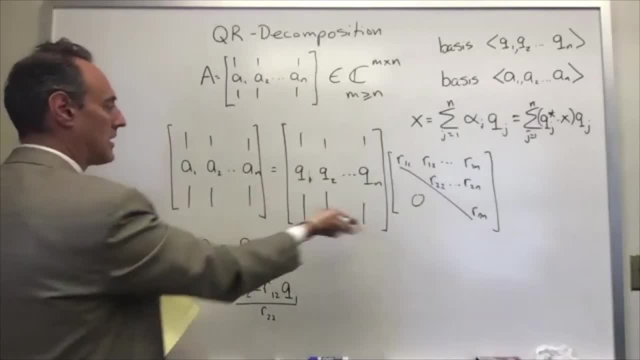 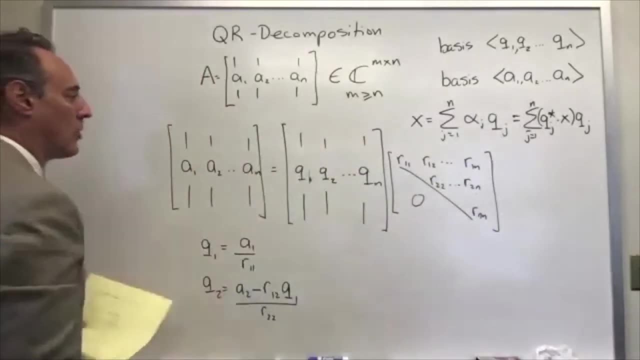 like: take the first equation, see what you get: It's that one. And then the second equation. right, You're going to hit this times this, this times this, this times, this and so forth to get out these sets of equations here. 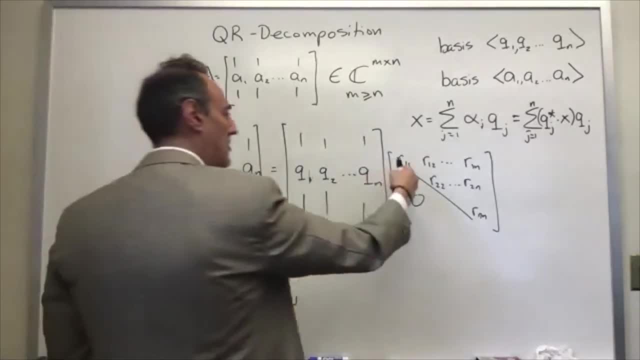 Okay. So the first column- this- hits this: R11 times. this is equal to A1.. Then the second column here hits this: It's all zeros, except it brings in these two. it's equal to the second column here. That's that equation. 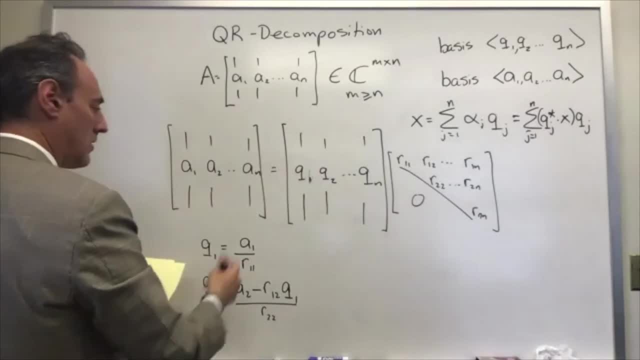 All the way down to the nth equation, which is- I'll write it over here- Q of n is equal to A of n minus j equals one to n minus one. Rj, n, Qj, all over Rnn. Okay, So these are all the equations I get out of here. 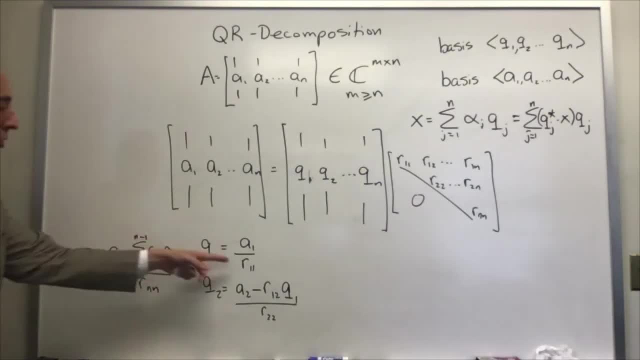 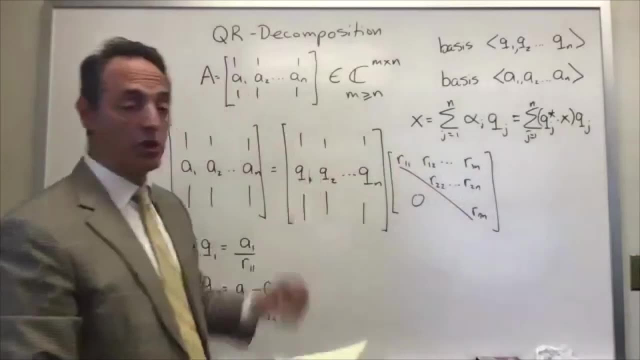 And notice. what I'm going to try to do is figure out what should. how should I pick the R11s, R12s, all the R? how should I pick these values And how should I pick the Qs? And this is where Graham Schmidt is going to come in. 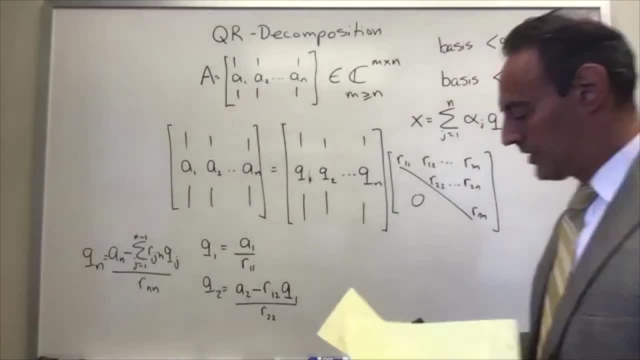 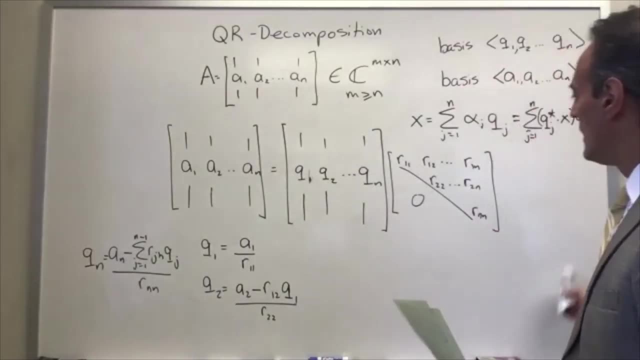 Okay. So, Graham Schmidt, what did I just show you? What I showed you is, if you take a generic coordinate system- and I'm going to go ahead, and it's the only part that is hard right- is when you don't have. 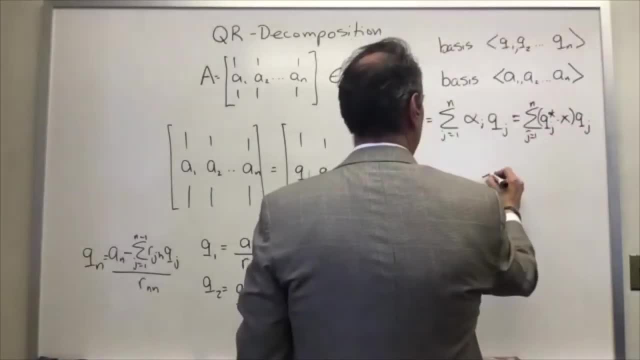 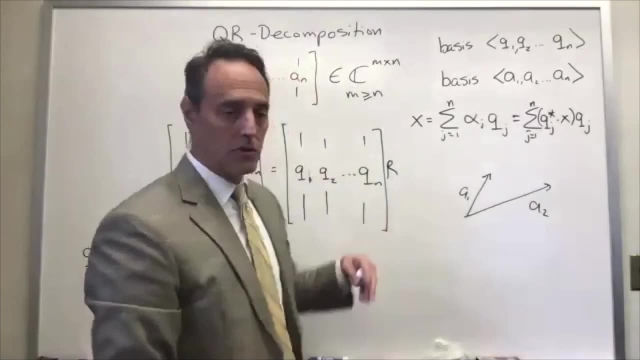 you run out of forward space. Let's take a generic coordinate system: A1,, A2.. And what I just showed you is, if I start to pick coordinates, then I'm going to start pick one coordinate and pick the next one to be. 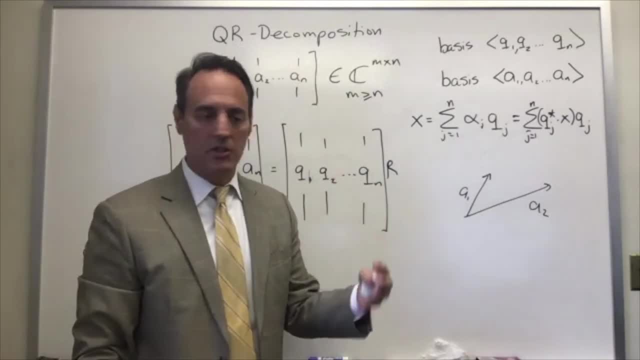 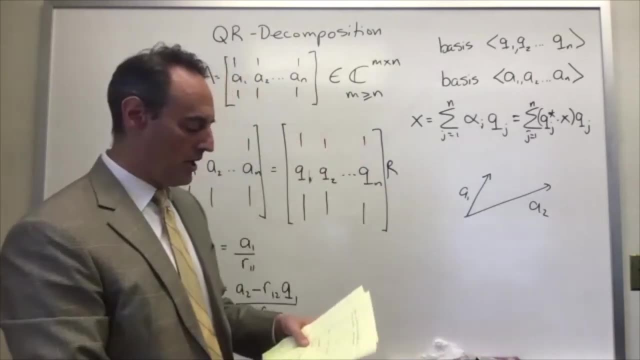 orthogonal to it. That's what Graham Schmidt does. It just says, okay, take A1 to be the direction of Q1.. Okay, So, in other words, the way this algorithm is going to work is you say: all right, Q1 is equal to the A1,. 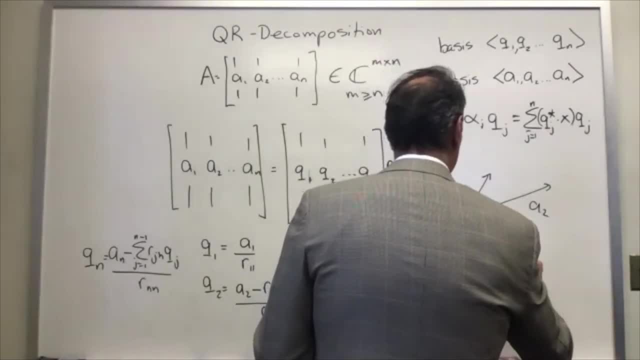 normalized. Okay, So I want this to be unit length. So Q1 is just this vector normalized to one. That's where you start. So I have one Q1 already in place. Now notice once I have Q1 in place. 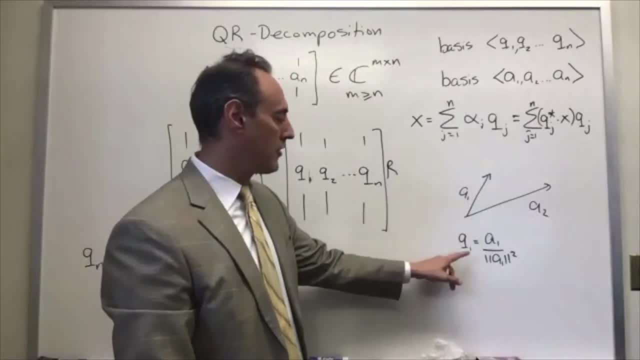 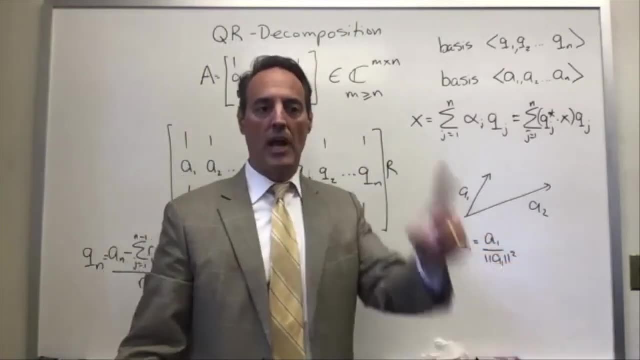 then it's pretty easy. right Here it is. I just take A1, A2, A3, A4, A5, A6, A7,, A8, A9, A10,, A11,, A12,. 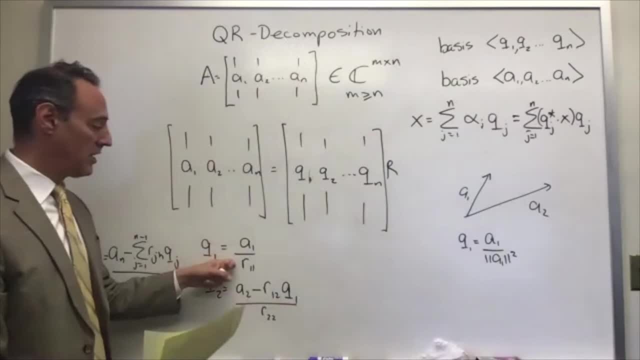 A13, A14, A15, A16, A17,, A18,, A19,, A20.. I divide by R11.. In fact, notice that. notice what I have here. Q1, I said, is A1 divided by this normalization. 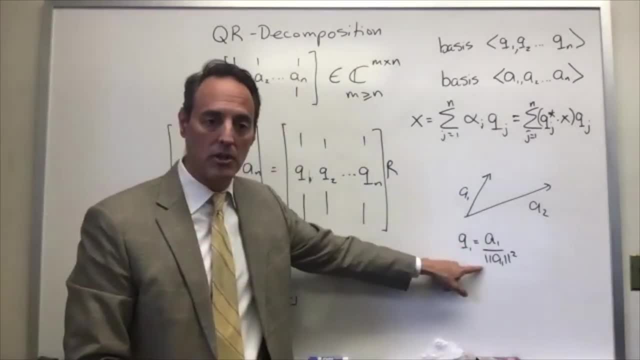 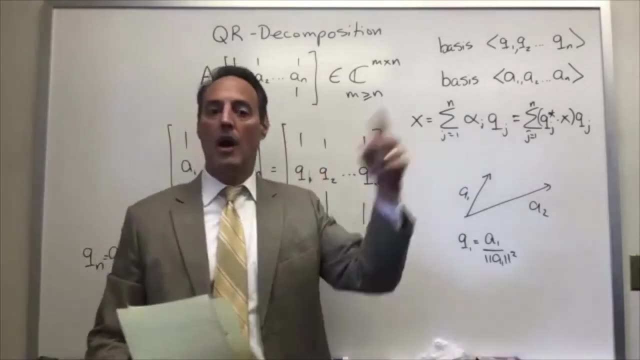 So this R11 is exactly this normalization. So there we go. I just basically rewrote that in a different form. So I've picked the Q, I've picked the A1 direction to start, which is the first column of that matrix, and say: 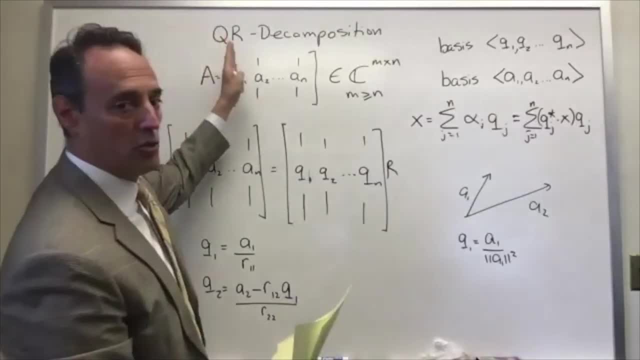 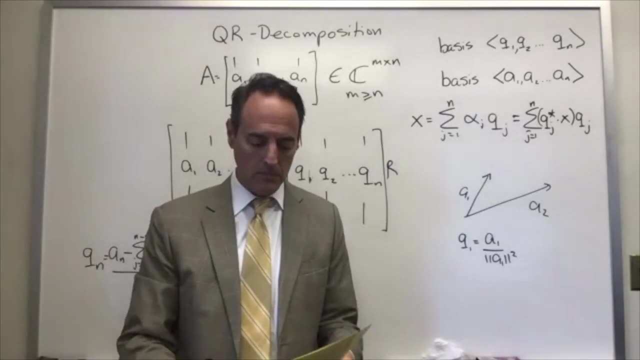 let's make that one direction. That's the Q1 direction. There's what Q1 is. Now how do I pick the next direction? Now I'm going to go to the second column and pick that A2 and figure out like: 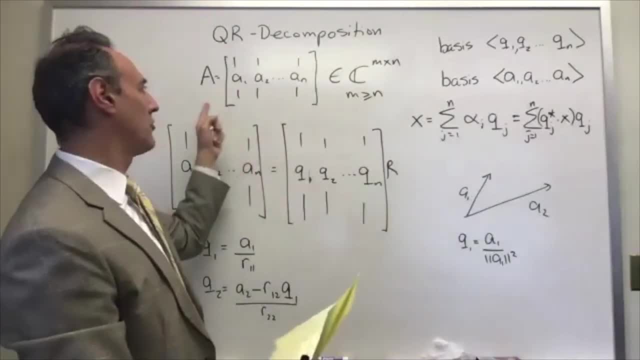 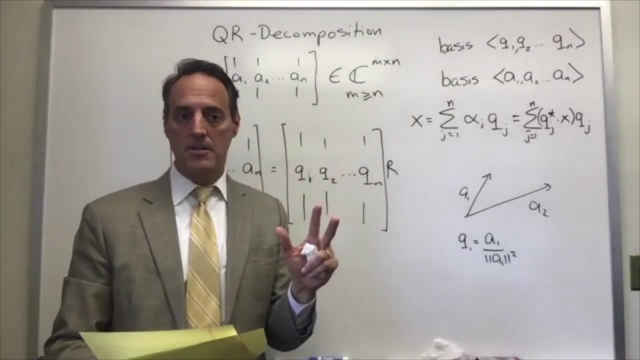 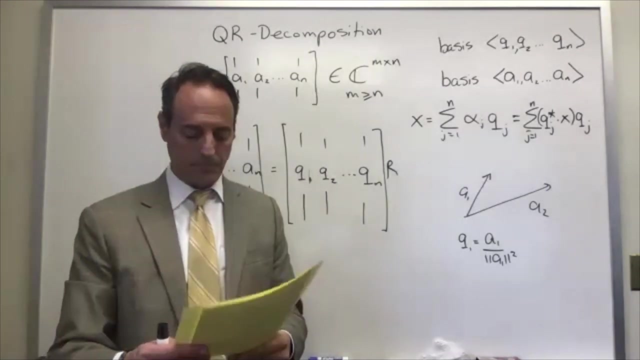 well, I want the next column to be orthogonal to the first one, But of course A2 generically isn't. A2 is just whatever direction it is. And so you say: like: how do I make A2 orthogonal to A1?? 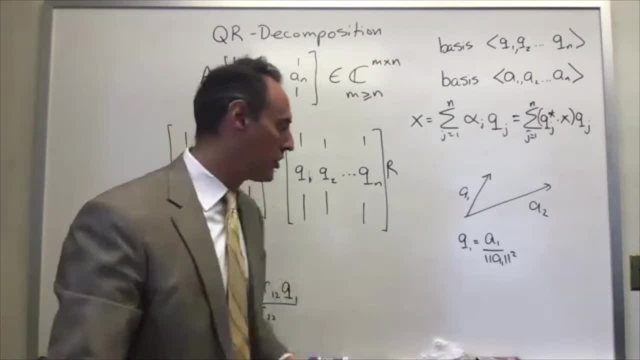 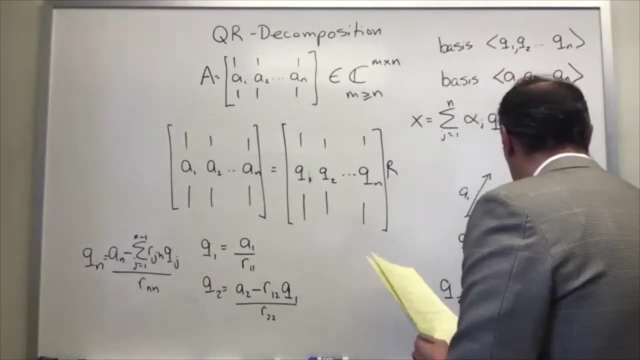 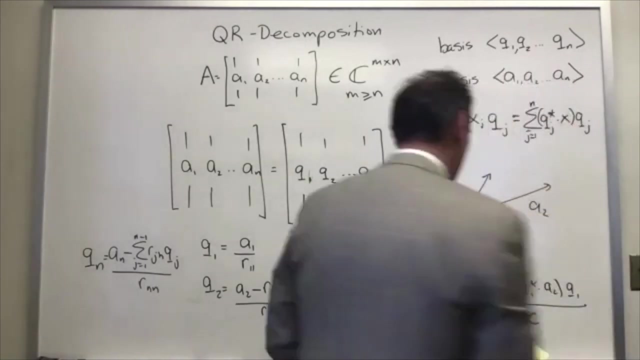 And so the way you're going to do this is you're going to say, all right, Q2, and I just drew this vector- is equal to the A2 direction minus Q1, star dot, A2, Q1 over some normalization. So notice what I did here. 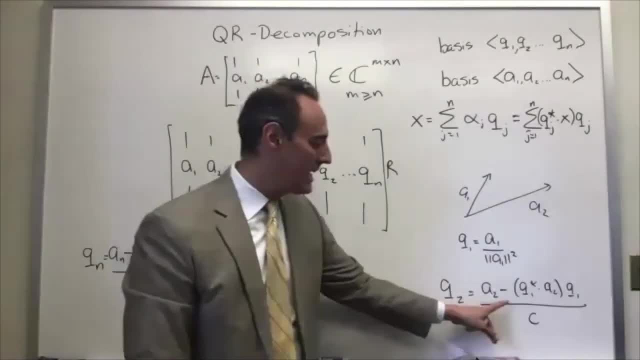 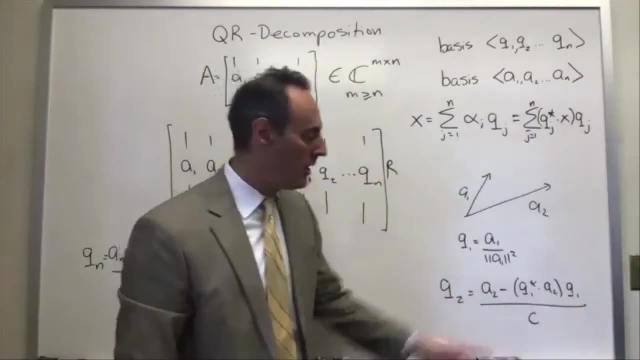 I went to the A2 direction and I subtracted out the portion of A2, which is along the Q1 direction. How did I do it? Well, I projected A2 into the Q1 direction. How much of it was in that direction. 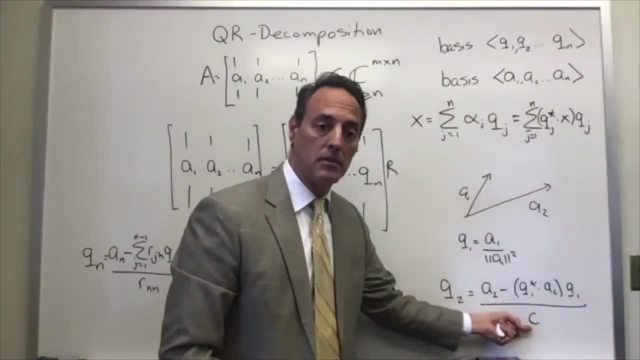 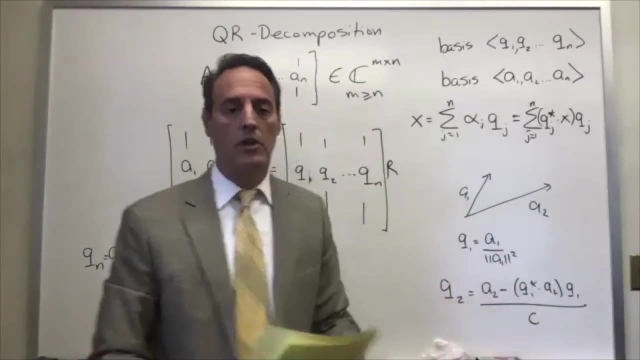 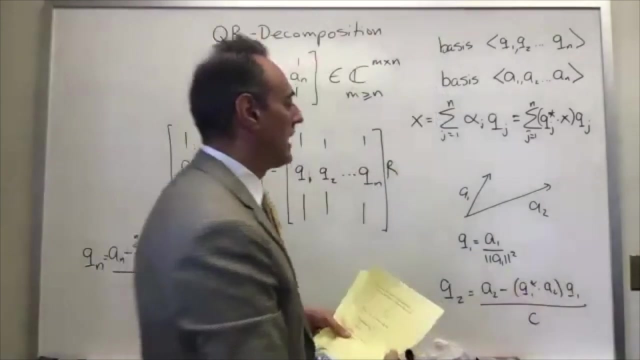 I subtracted it from it and I normalized. The normalization is just the length of that vector. Just a quick question. Yes, Is the normalization for Q1 the square of the norm? Yeah Well, it doesn't matter, because this is one. 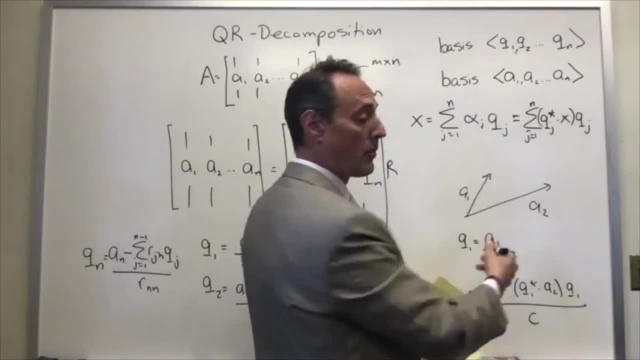 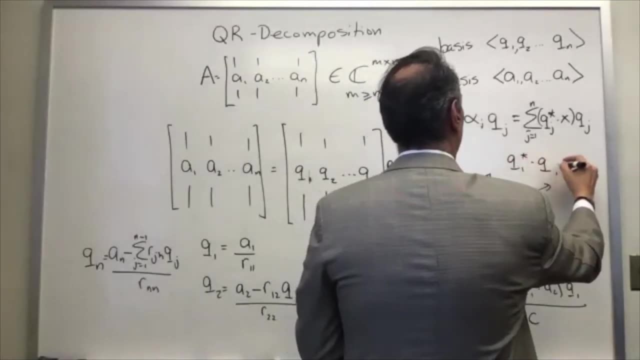 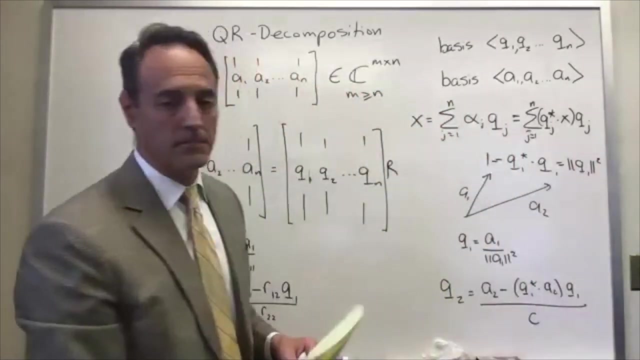 right. So normally what you do is you can either do square root of one, It doesn't matter here, But normally I always like to represent it like this: So that's Q1 star. Q1 is equal to, and that's equal to one. 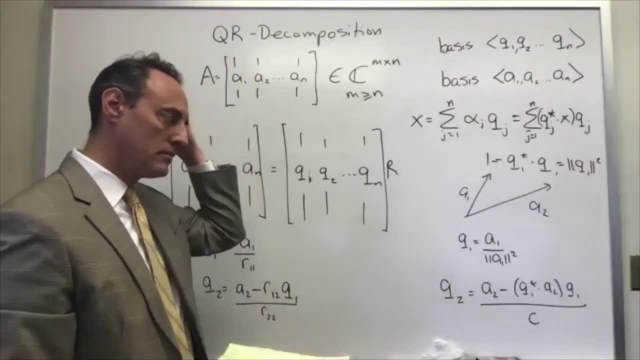 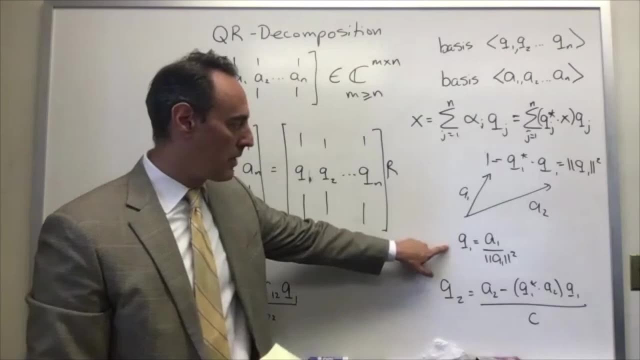 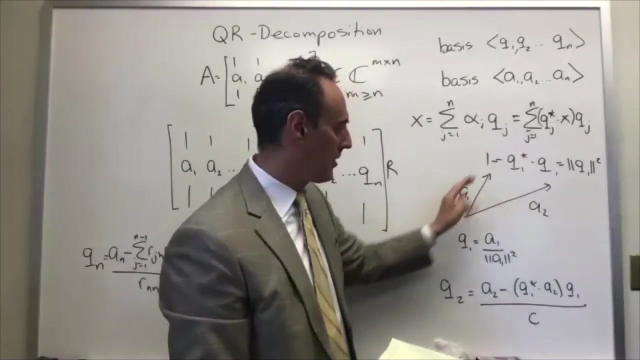 Okay, All right. So hopefully everybody's okay with this. So I picked one direction and the second direction I just say: pick the next vector And notice: this vector here has a component that's along the A1, but also has a component that's orthogonal to it. 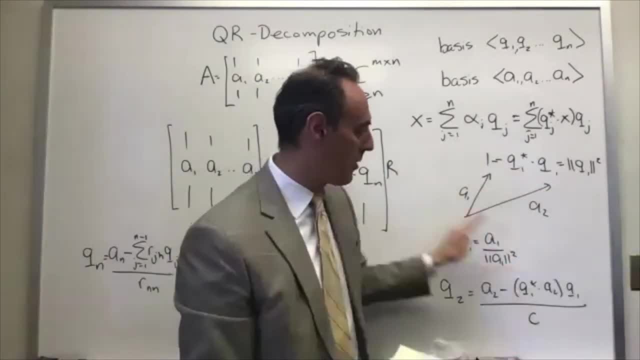 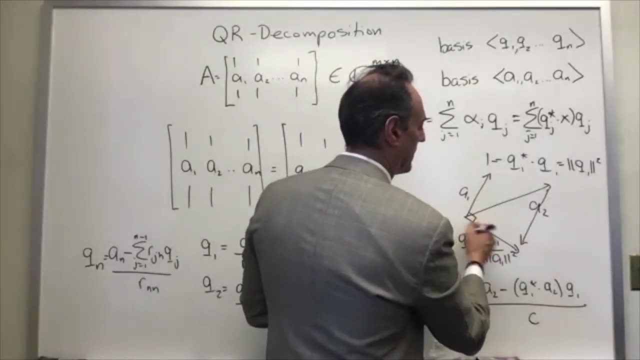 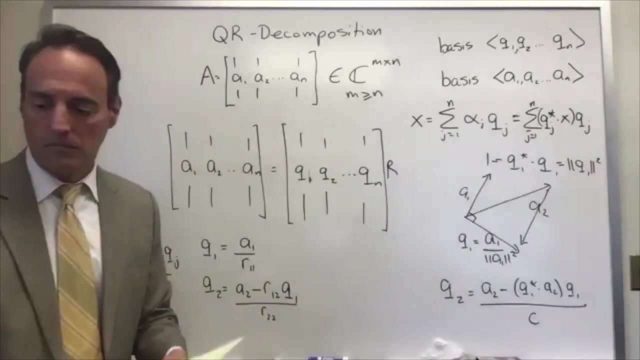 So I take this vector, I subtract out the component along this direction, Right? So if there's some Q1, I subtract that out, And now I have that vector here And that's now orthogonal to Q1.. There, So that's how we use Graham Schmidt. 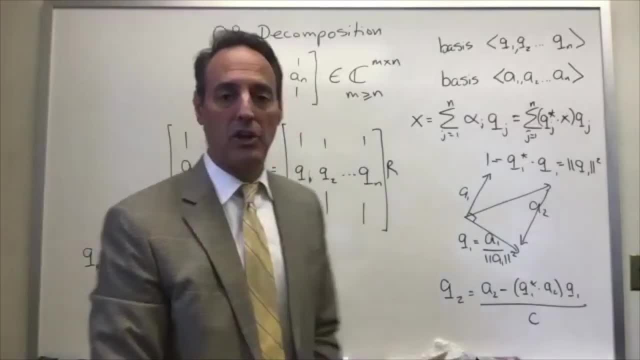 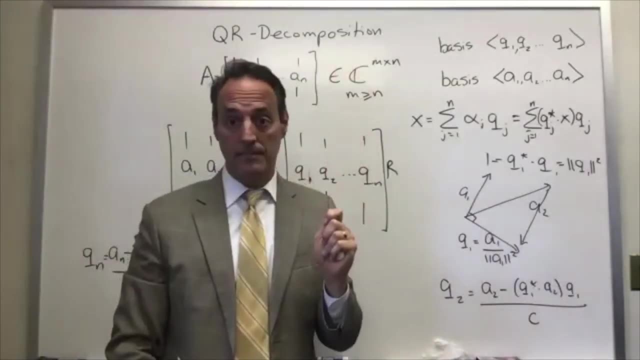 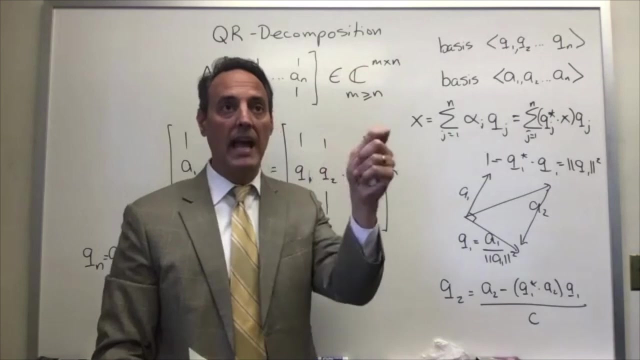 And Graham Schmidt just says, okay, how would you pick Q3?? Same way You say: take now the third vector, A3.. And you take that A3 vector and you say, all right, I want the Q3 vector to be along A3. 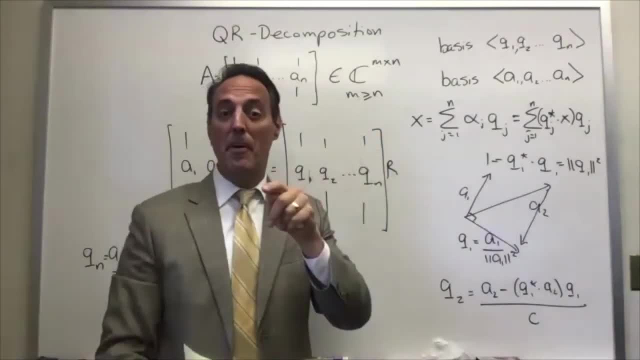 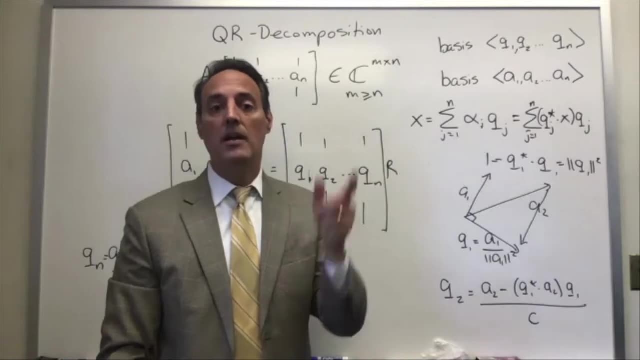 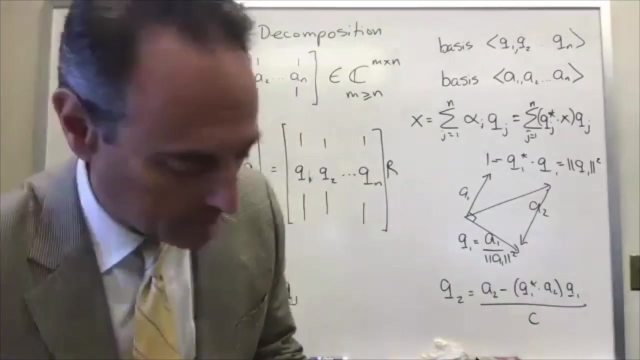 And I'm going to subtract out from A3, the component along Q1 and the component along Q2, so that it's orthogonal to those two, And then I normalize. That's the whole routine For Graham Schmidt. So the way to write this, then, is: what you're going to find is the following: 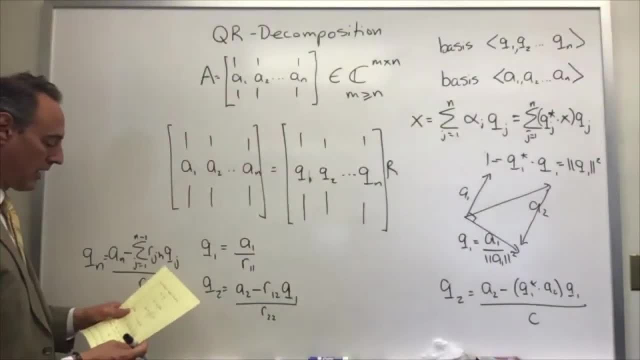 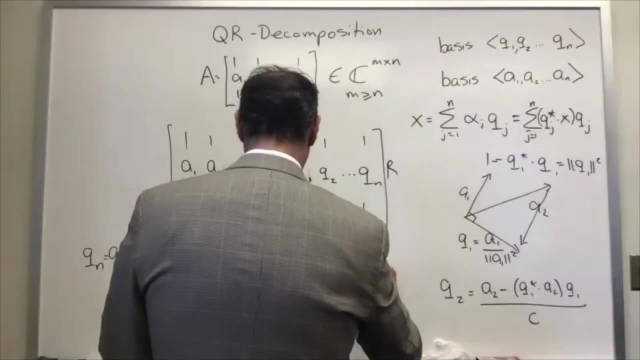 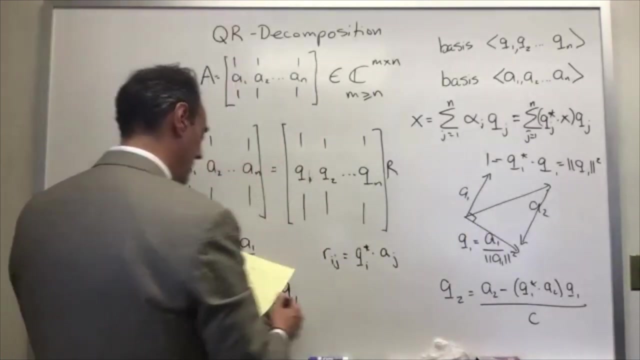 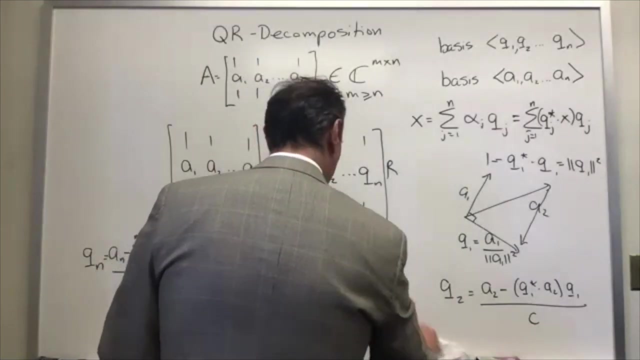 If I come over here and I get this thing, the RIJ- you can work this out- is QI star dotted with A of J, And the RJJ, which is the normalization, is equal to A of J. I'm going to erase this so I can write this. 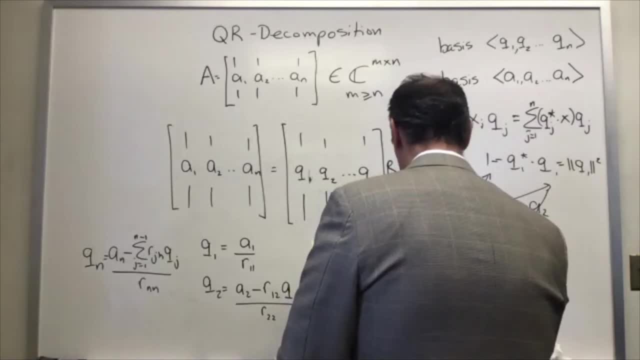 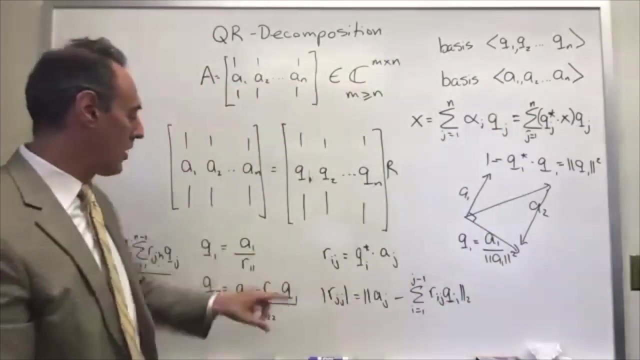 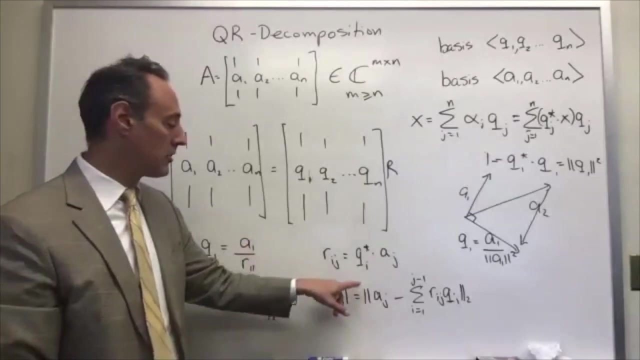 minus sum I equals one to J minus one RIJ, QJ, sorry, QI. So when you work this out, you notice that what I'm doing with all of these R of I's is I'm just projecting onto the previous vectors. 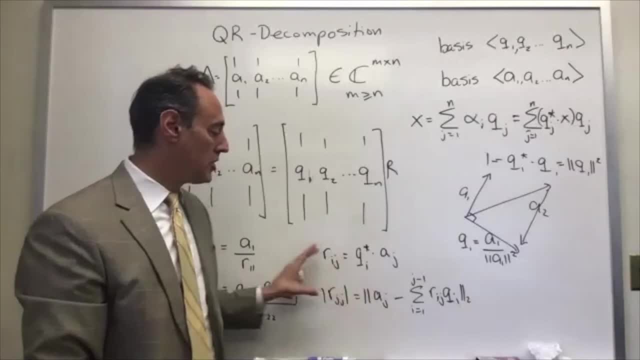 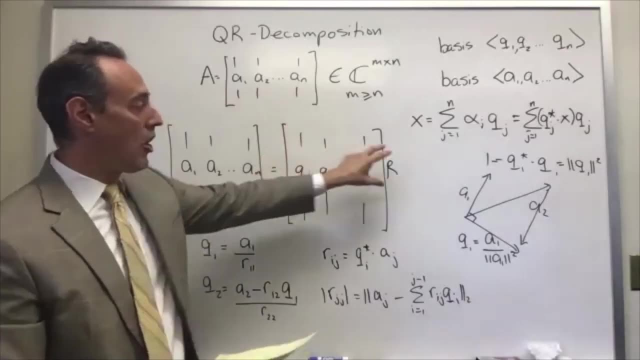 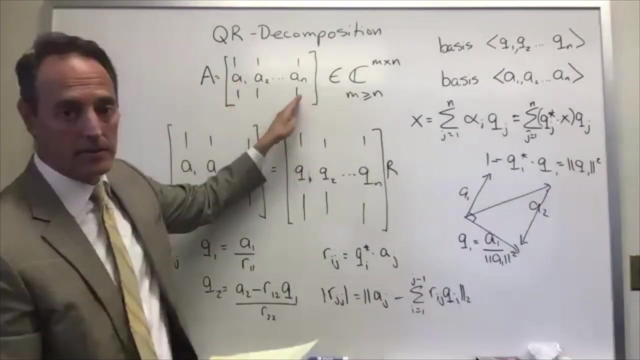 Okay, That's what this does And this is the norm. So this gives me a formula for how to produce that R matrix, which is upper triangular, given that I'm selecting column by column as I move across here, So I pick this vector. 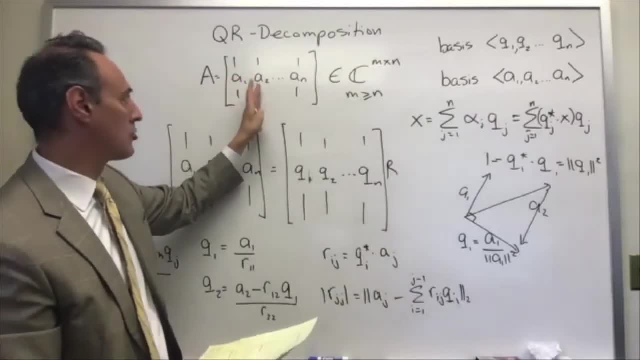 make it unit length. I now take this vector, subtract out the portion that's orthogonal to this. make a new vector of unit length. I pick a next vector. make it orthogonal to the two before it. make it unit length, I pick the next vector. 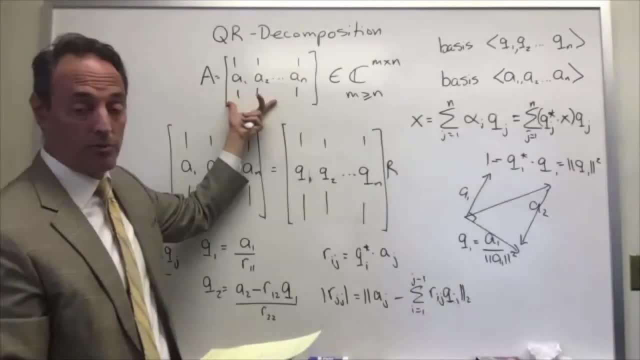 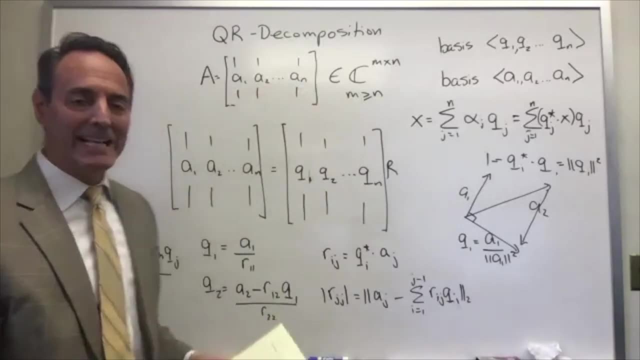 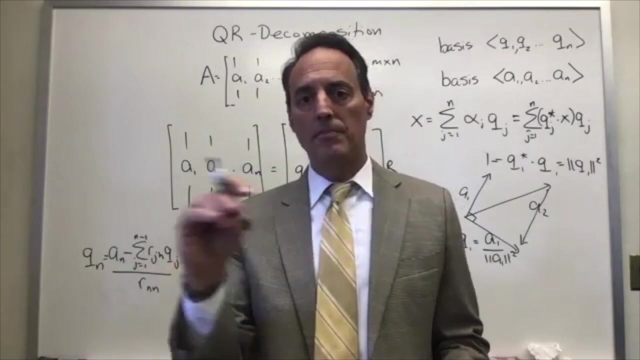 make it orthogonal. project out the first three vectors to make it orthogonal to them, make it unit length, and I just go down that thing. Okay, That's how we just can produce the QR decomposition. Now, what I'm going to tell you is that we're going to spend time in the next 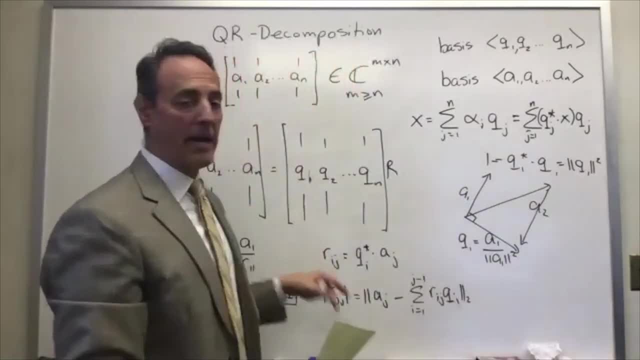 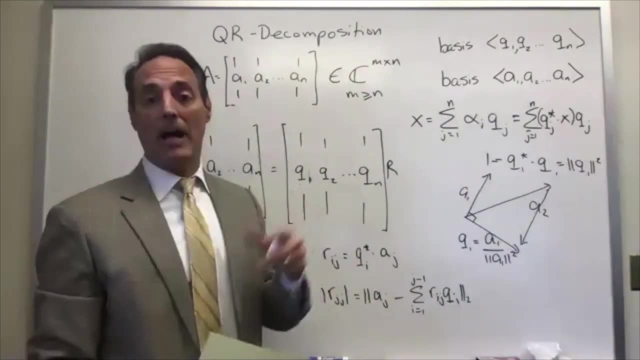 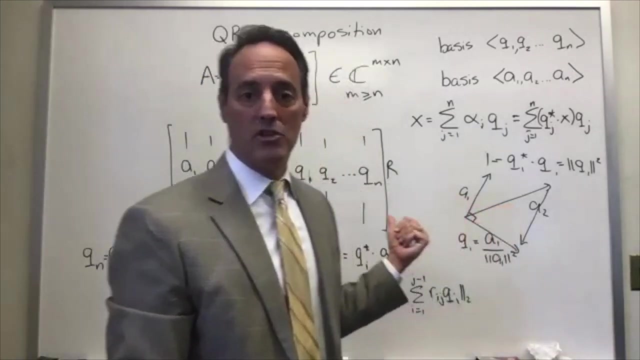 couple lectures is to take this, this basic Gram-Schmidt algorithm, which is actually it's one thing to write it down, It's another thing to develop a stable algorithm to compute it. So the standard Gram-Schmidt often produces unstable algorithm to get these.